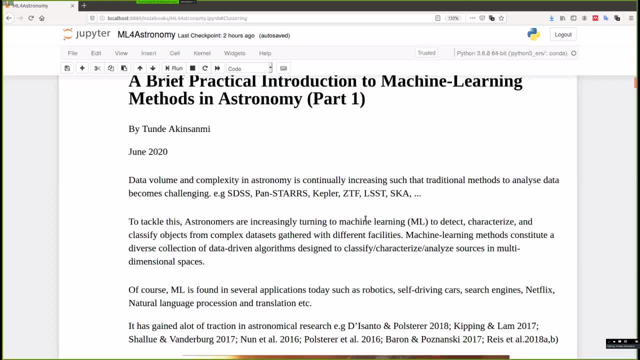 Of course, we are all aware of how machine learning has been used in several applications like self-driving cars, search engines and- my favorite one, Netflix and natural language processing. But if you look through the literature- and I remember talking to Andre on Monday and he talked- 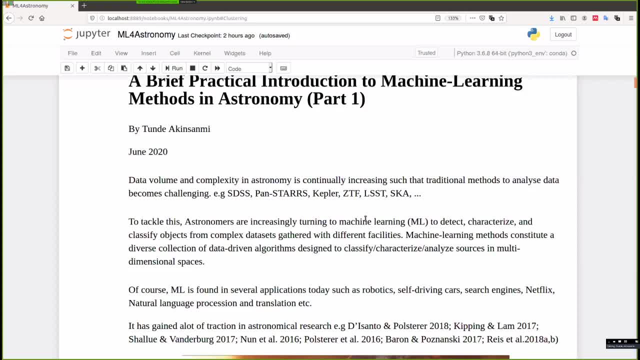 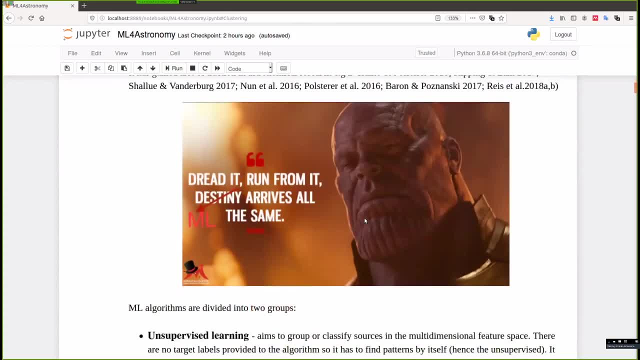 about how most of the papers on archive on Monday we're all machine learning papers, So we see that this is gaining a lot of traction. So you can dread it, you can run from it, but machine learning arrives all the same. So we need to prepare ourselves for this. 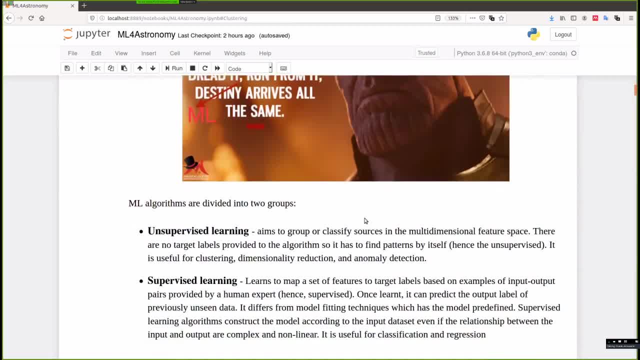 and machine learning are generally grouped into two categories: the unsupervised and supervised learning. In the unsupervised class of learning you aim to classify sources in maybe multi-dimensional features, but that's not the case of feature space, where you don't actually know what is contained in the in the data at first. 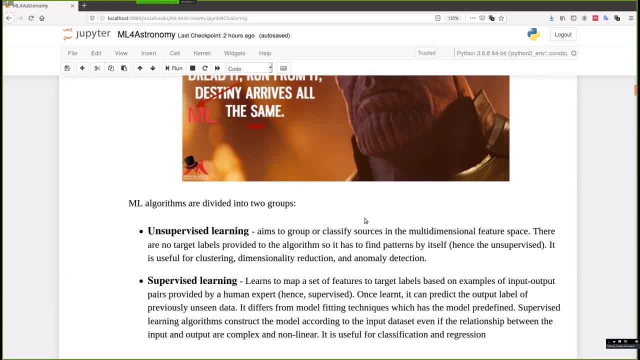 glance. so you you need to find some kind of classification, which you don't necessarily know already. you want the machine learning to be able to classify this data and tell you what to expect from the data. so this has been very useful in, maybe, exploratory science. you want to know what's. 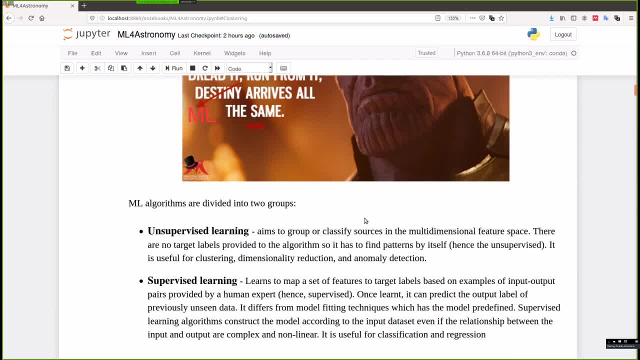 in the data, but you don't want to be too biased to already tell it what to give to you, so you let the machine learning figure it out. this is why it's called unsupervised learning, and it is useful for dimensionality reduction, for detecting anomalies in your data and for clustering. 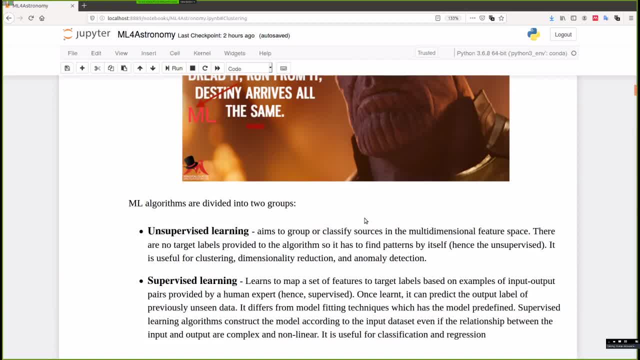 the second part is the supervised learning, in which case you already know what you expect from the data and you perhaps have already labeled data. you already have, say, data labeled as cats and dogs and you want to be able to classify new sources, so either fall in either of these. 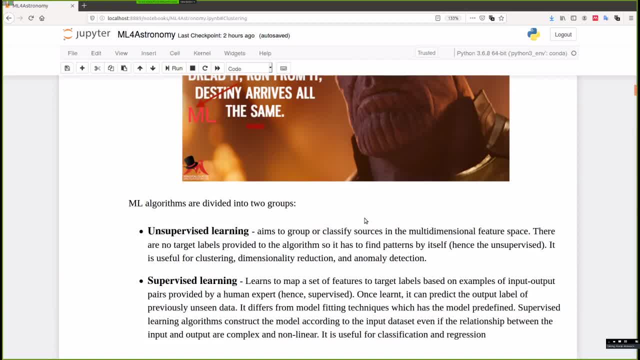 categories. you used what what is called supervised learning, and this requires some training. you have to give examples of input and output pairs which you want your machine learning to train itself upon so that it can perform these techniques, perform this kind of matching on on data it hasn't seen before. 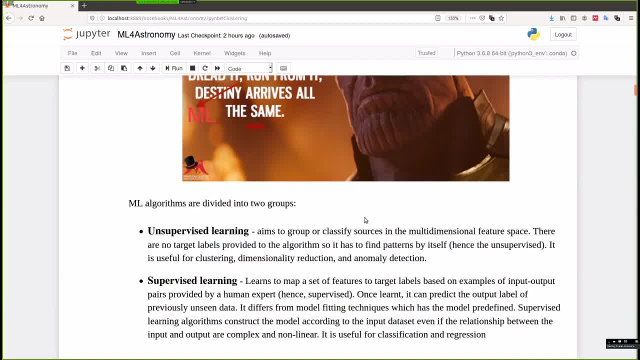 and it is very useful because it can find mapping between features that are not necessarily non-linear and can be very complex and so in a way that parametric models cannot necessarily figure out. so you have a set of data-driven models that can tell you something about your data without you. 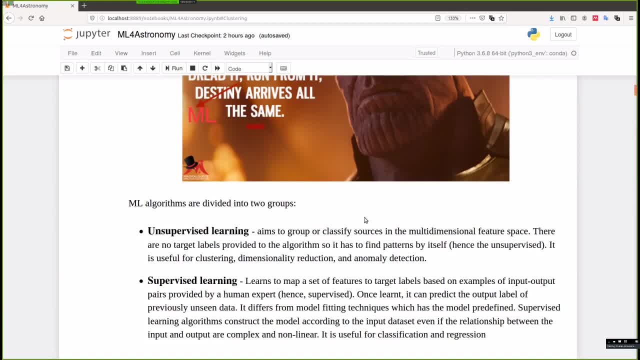 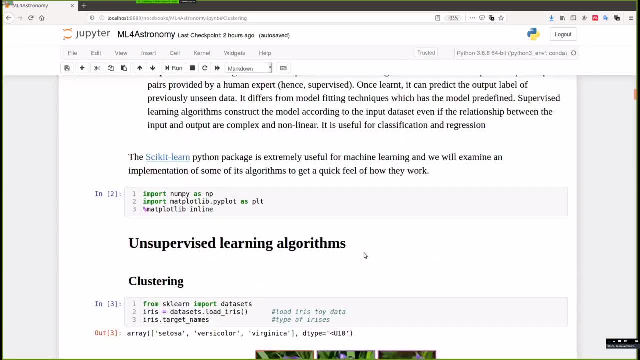 enforcing a particular relationship, and it's also useful for classification and regression purposes. for this, for this particular notebook, i've chosen to make this presentation in a notebook. i don't know, can people see the the text in the notebook clearly? yes, at least i can. okay, i've not necessarily used machine learning in my research so far, but it's something i'm 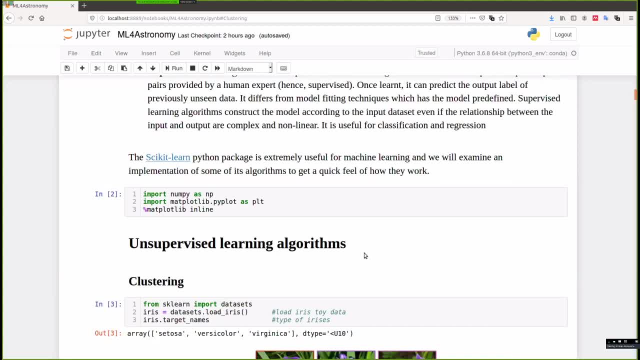 constantly looking to, to explore, in getting the based out of my science. so most of the algorithms i'm going to describe here are things that i've just read about or learned some things about, and i thought it would be useful to share some of them with you in the form of a python notebook, because it gives you a handy go-to place where you can. 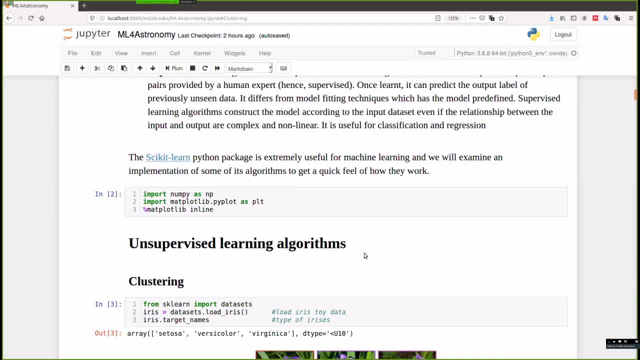 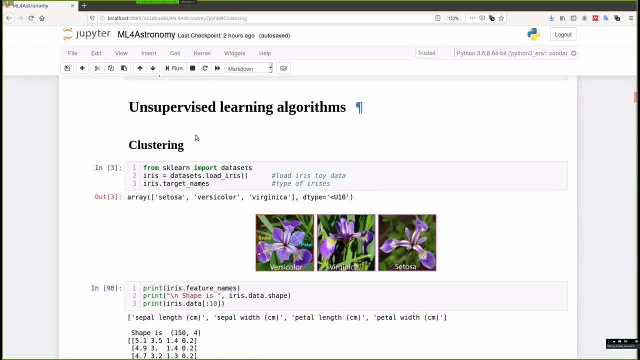 just pick up some contest, some concepts and use it as you wish. so let's start with the unsupervised linear algorithms, the first of which is clustering. in clustering, the task is basically: you're trying to find groups of data that have similarities to each other such that 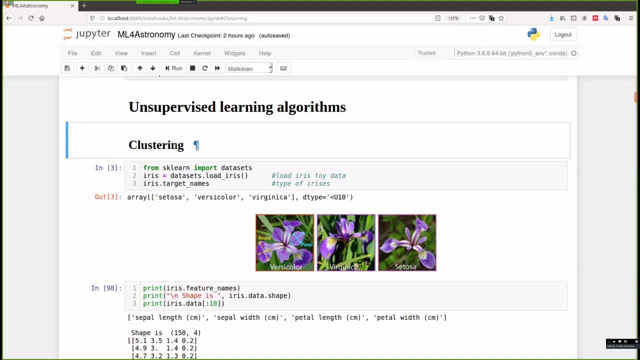 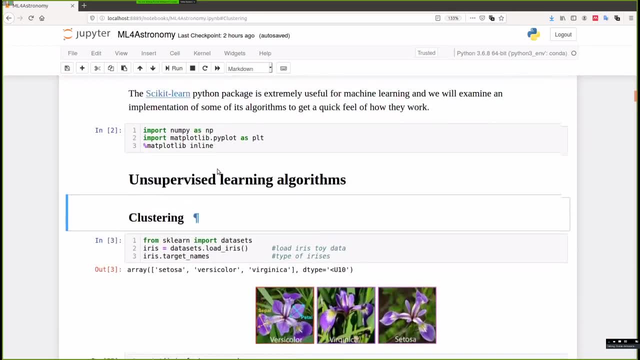 a particular cluster will have some sources which are similar to each other than the other ones. so i'm going to start with the unsupervised linear algorithms. so i think the first example from: oh, i have to mention first that the sql learn scikit-learn python package is very useful for 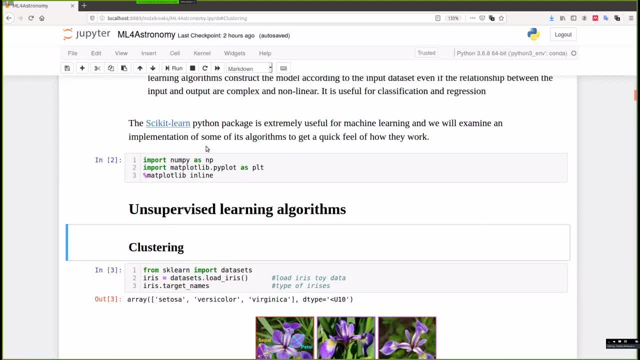 machine learning. it's literally where you go to first if you're trying to perform any machine learning exercise on your data, and has some very useful algorithms- most of most of the machine learning algorithms actually- and we're going to get in the feel of some of this in this. 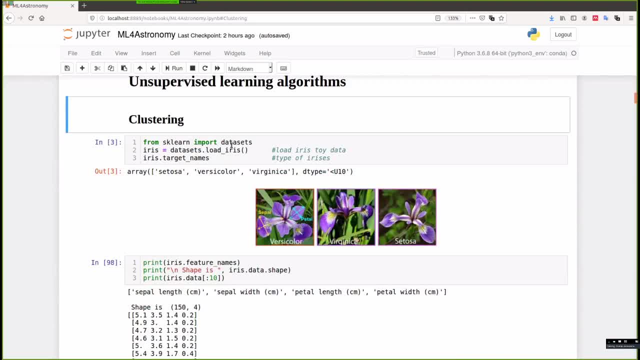 in this notebook. so if you, if you install the scikit-learn package, you can import the very popular data set called iris. set consists of three, three types of irises: the versicolor, the virginica and the setosa. and this: this irises are defined by features called the petal and the sepal, the petal and the. 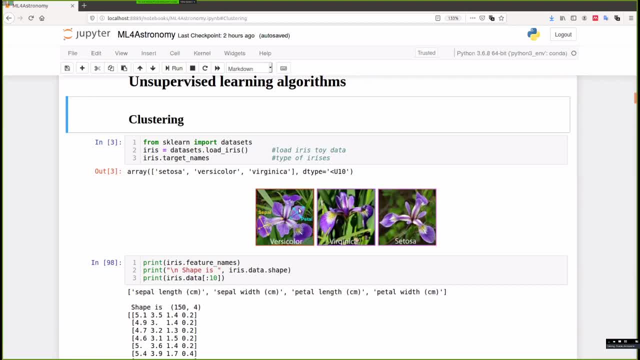 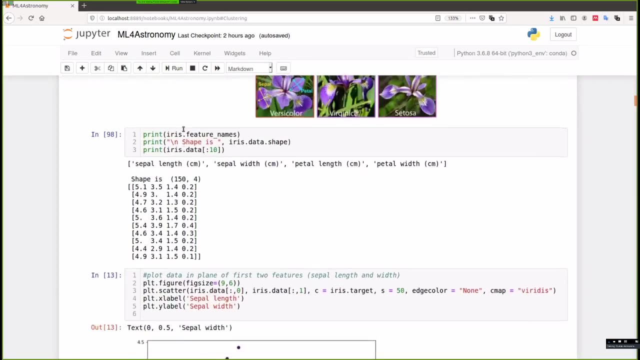 sepal can be. you can measure the width of each of the, the petals and the length of them and also the sepal. so you have four features which particularly describes each of this, each of these types of iris. i print out here the kind of data that's inside the sep, the iris data which shows it's a 150 by 4, meaning you have 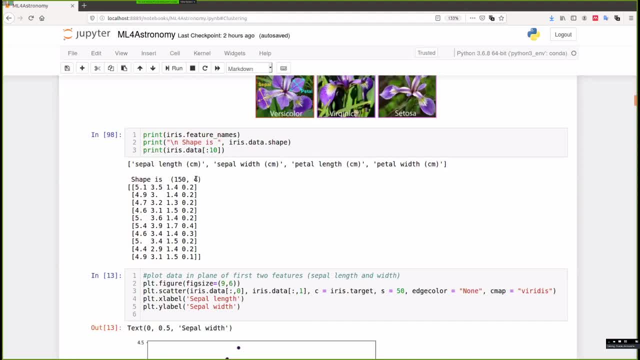 four features in the data, like i just said, and you have 150 classifications so you can measure for each of this class of irises. you have measured all of these features and you have them here. they have been labeled in this case, but let's assume that we don't know the labels of this data. 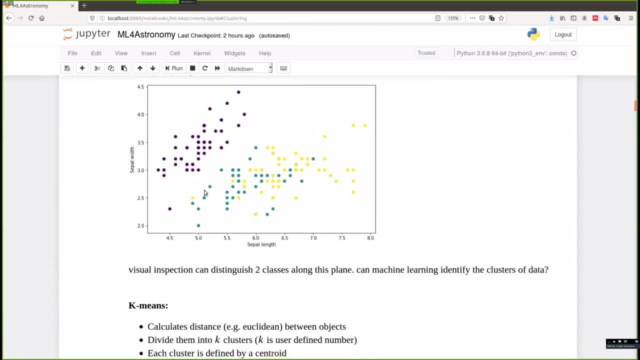 i plotted the data here for you to see on a two-dimensional space of sepal width and sepal lens points. here i can can be linearly, uh, distinguished from the, from the other two sets. but imagine you don't know anything about this data set and you plot it in this, in this space. 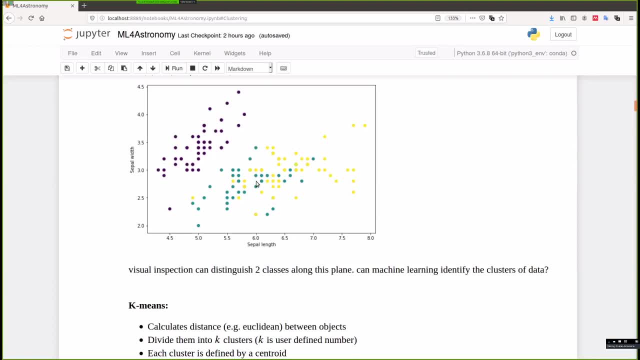 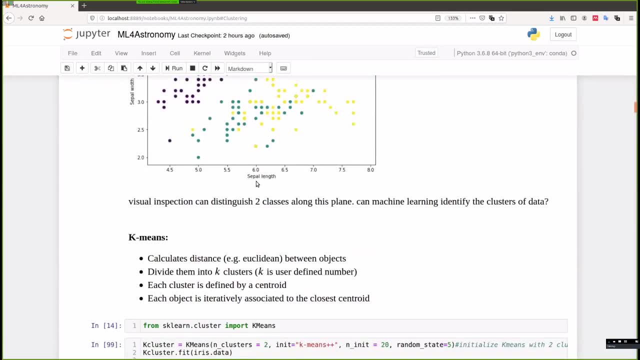 how would you be able to cluster this data set in order to identify which ones are the diversity versicolor, the septosa and the what's the third one, the virginica? the first algorithm i'm going to introduce is called the kaemins. kaemins clustering in chemist clustering. 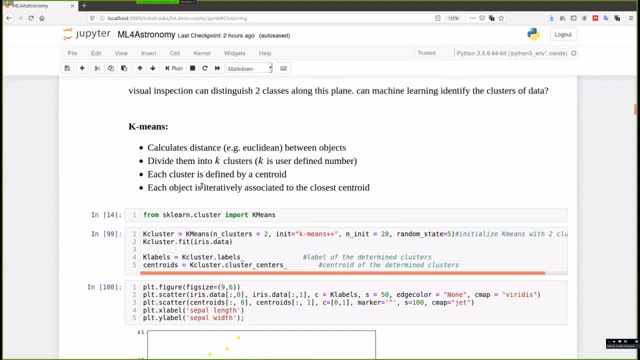 you literally have to calculate the distance to each centigram in the bibliography by whether you would like to know the less part of the way that the setosa near the seriously. now here comes the: the distance to each of the data points that you see using, say, collinear distance between the objects. 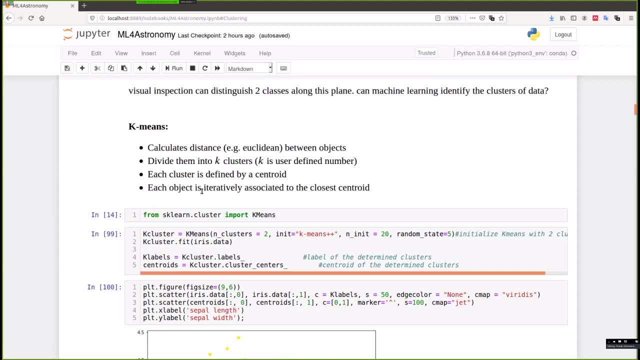 divide them into clusters. You have to define how many clusters you aim to find in the data, which is the rub of this algorithm. You have to define the amount of clusters to find in the data, And each cluster is then divided, is defined by a centroid. 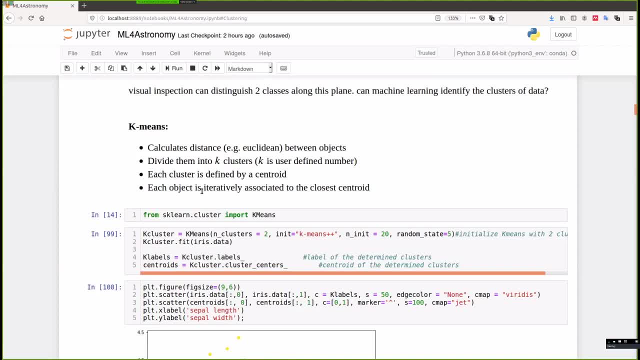 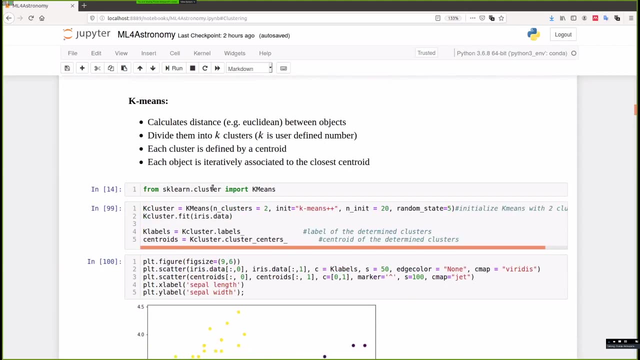 A centroid is like a mean of the cluster points in a particular space, in the parameter space. Then you iteratively associate each of the random points to the closest centroid that you can find in the data. So it's a practical presentation. So I'm going to do this practically. 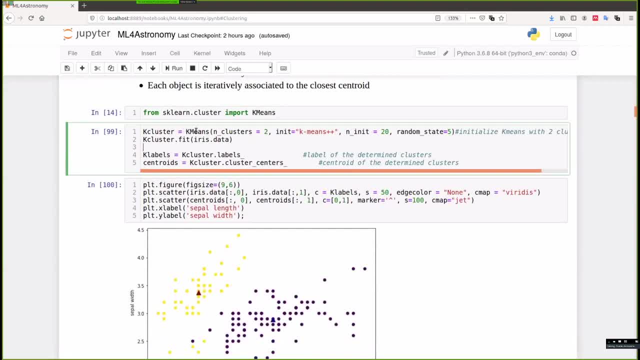 So imagine that I initiate a K-means object with two clusters. Let's forget about this initialization for now, but this is basically how the K-means figures out where to start from in identifying the centroid and the data sets. So all you basically need to do with SQL. 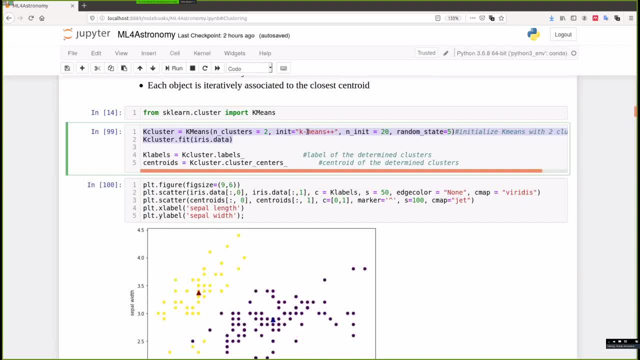 is to define an object to classify the sources I put in the data here as iris data and fit it with the objects that you just created. After this is done, it creates the labels for each of the data, telling it if it belongs to label 0.. 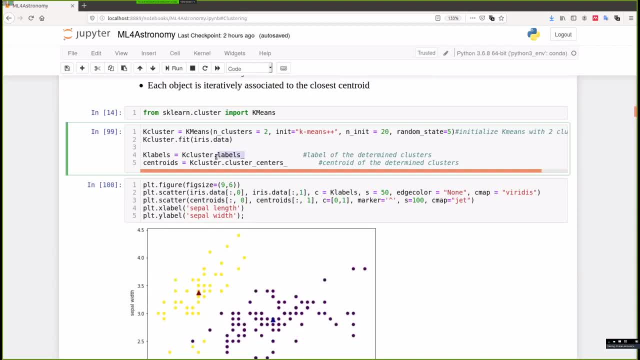 It doesn't know the names of the labels. of course, the labels are 0,, 1,, 2,, 3,, depending on how many clusters that it finds in the data sets, And you can also point out the centroid of each of the cluster data sets. 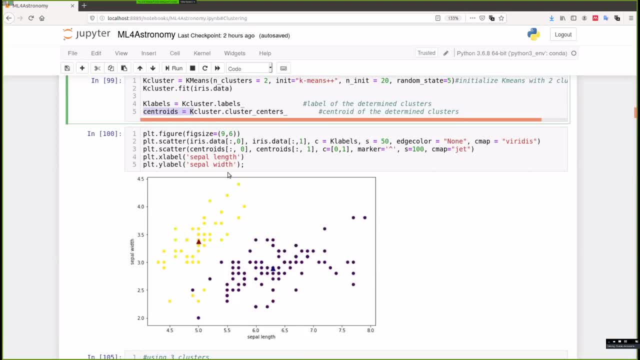 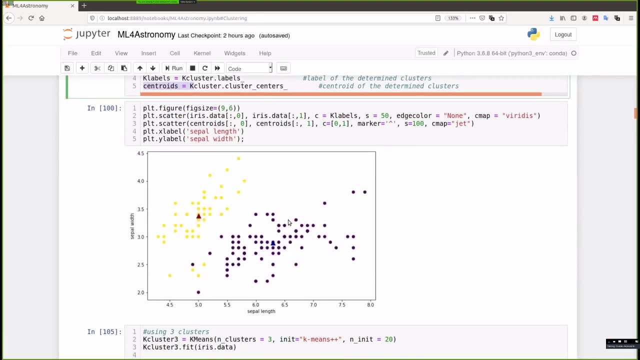 Running this on the K-means on the iris data sets using two clusters, you can see it has identified two distinct clusters, but we already know a priori that there are three clusters in this data set. so this is one problem with clustering algorithms. it gives you. it gives you what you tell it to give. you give to you. 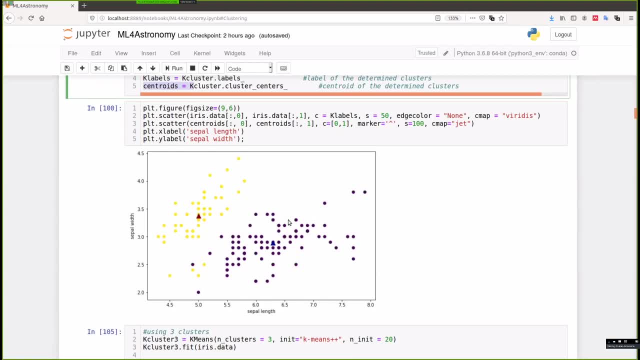 so it doesn't necessarily know how many clusters there should be in the data set. you don't know when it has converged, but if you ask it for two, uh, two, two clusters, it gives you this result. let's assume now that we know that there are three clusters in this data set. 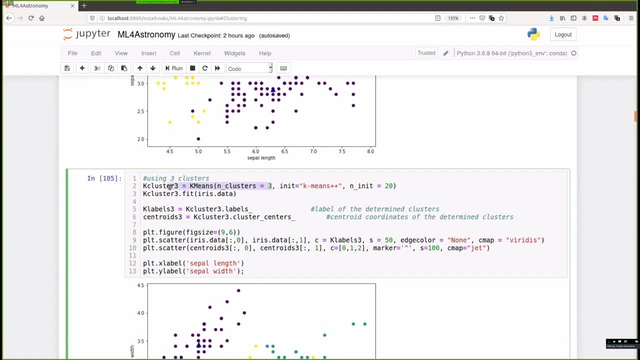 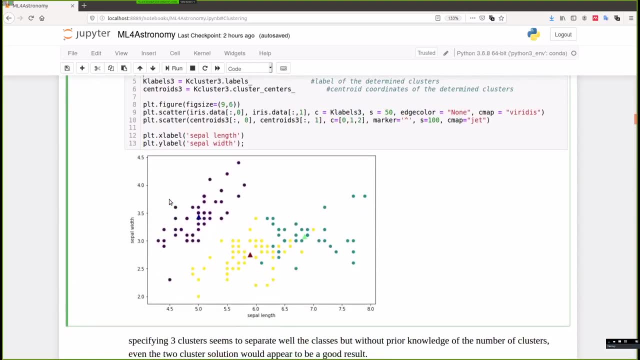 we can run the same algorithm again now with three clusters and fit the data sets. in this case you can see that it has pretty much recovered three clusters of data sets in this, uh, three clusters in this data set. but then one would ask the question: how do i know how many clusters to? 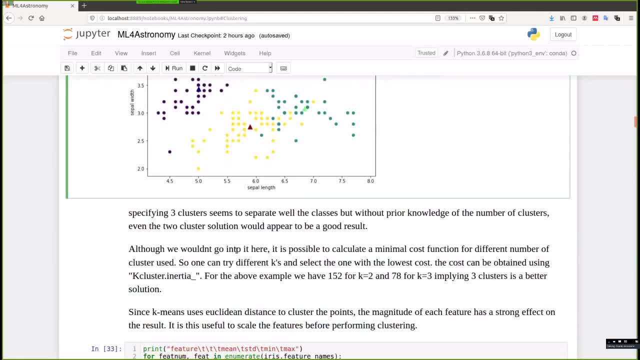 initialize my, my model. so the truth is that it is very tricky, but it is possible to actually calculate what you call the inertia or some kind of cost function for the for the fit that you just performed. in which case, if i run this for my data we i have a value of 152 for k, equal to 2, which is 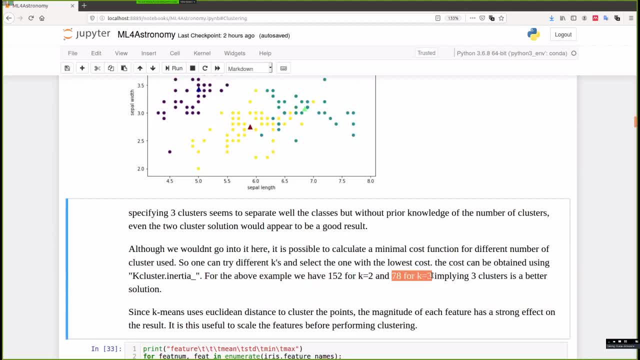 the number of clusters, and 78 for k equals three. the lowest. the lowest number tells you that it's a better fit to the data, which implies that in this case, um k equals three, which is three clusters, is more appropriate to distinguish this data, set a more. 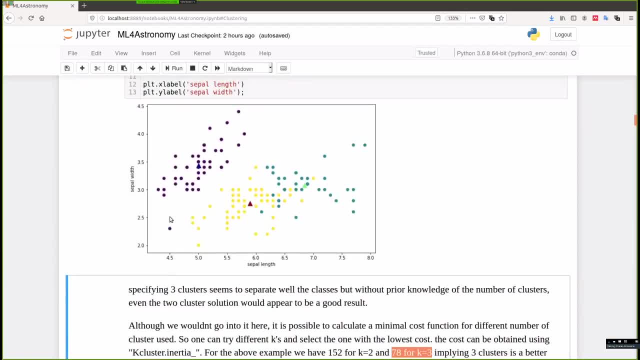 pessimistic person might say, but by eye i can already see that it's possible to classify, to split this data set. in some sense this is very true. but when you begin to have dimensions that are going from, say, 3 to 12 to to- whatever you might think of- 64 uh dimensions, then it becomes. 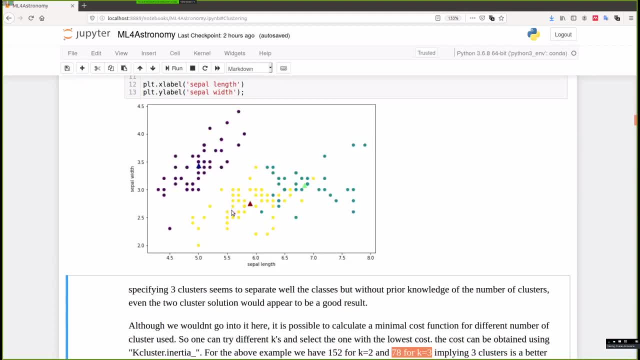 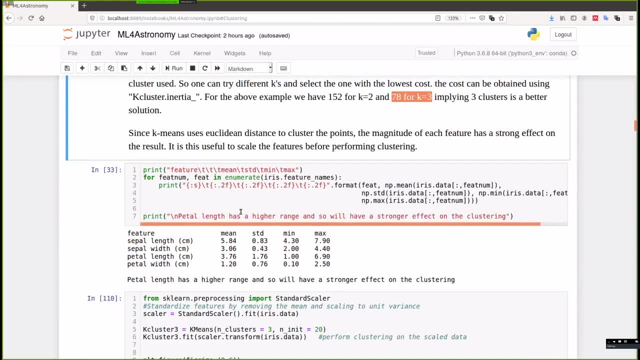 difficult to separate these things by eye, which is where machine learning needs to come, really comes into its own in separating data into different different clusters, um. but since k-means actually uses the euclidean distance between the points, the magnitude of each of the feature can actually influence how it clusters data data sets. i print here the mean. 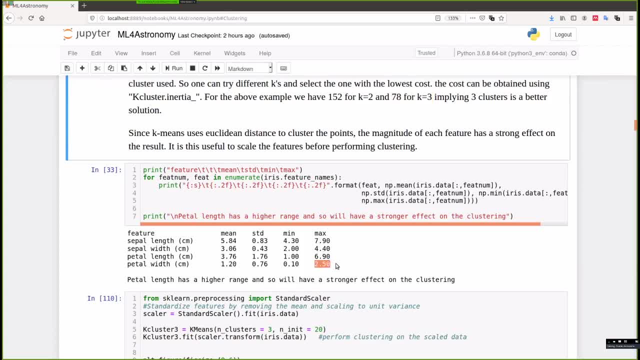 standard deviation and minimum and maximum of each of the features in these data sets. you can see here that this petal length has a larger range, going from one to six. that means that this is going to have a huge impact on how you you cluster the data sets and especially in astronomy we can 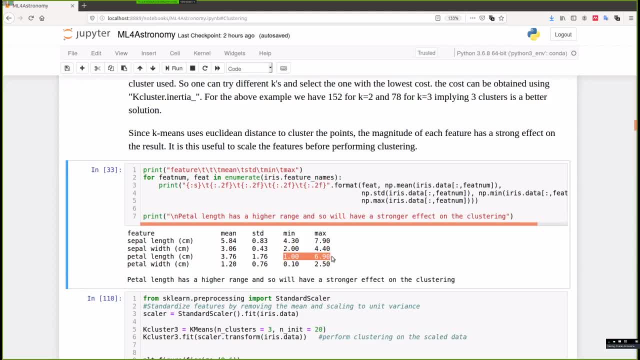 have, uh, we can have features in our data set that range from uh three orders of magnitude, whereas one just goes from, say, metallicity goes from zero minus 0.2 to 0.5, something very small like that, whereas you can have some ranging from one to one thousand. 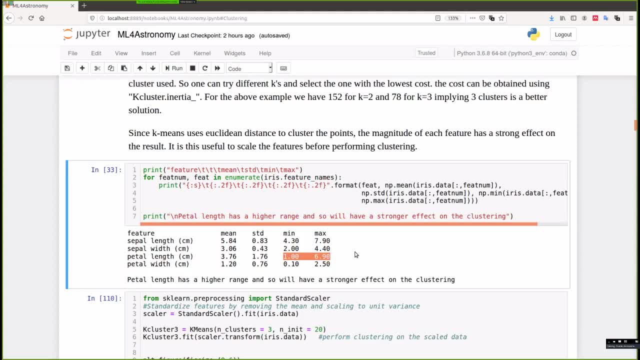 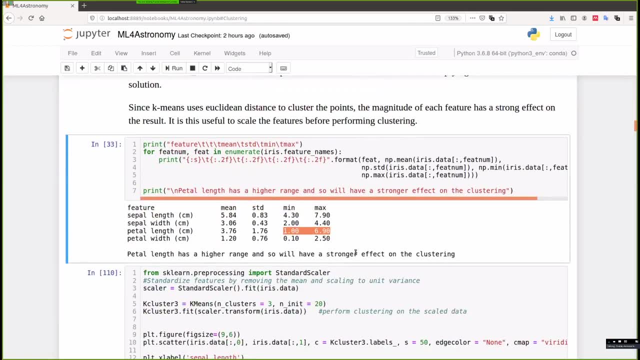 so a a good effect, before you run any machine learning algorithm, is to actually scale the data set, to have uh, to scale the data set across the features. so you have say that you have them running from, say, zero to one in all the cases and you can have a more efficient clustering uh in this case. 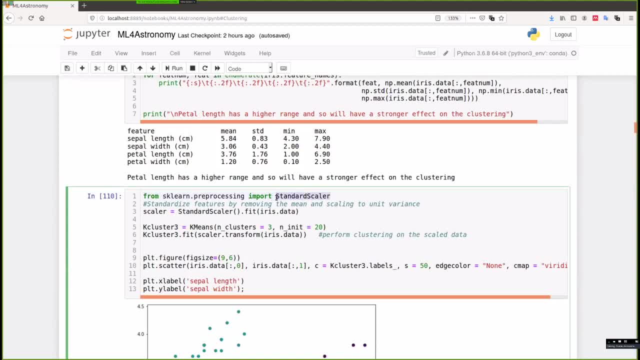 you can use a mean max scalar to scale your data. but within the sgln you also have this. uh, you have. you have this method called the standard scaler you can use to scale your data. so, uh, you can. this, the stand standard scalar actually removes the mean of the data to zero, then gives it the unit. 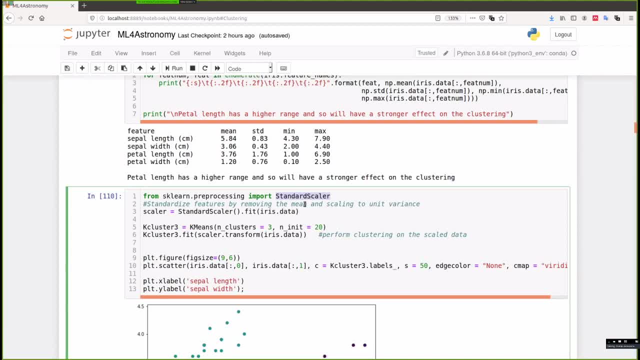 variance. so every data, every point in the data set runs between zero and one. you can also use a mean max scalar where you subtract the mean, the minimum of data, and scale them between zero and one. in our case, because this data set is very small, it doesn't have much of an impact on the clutch screen. 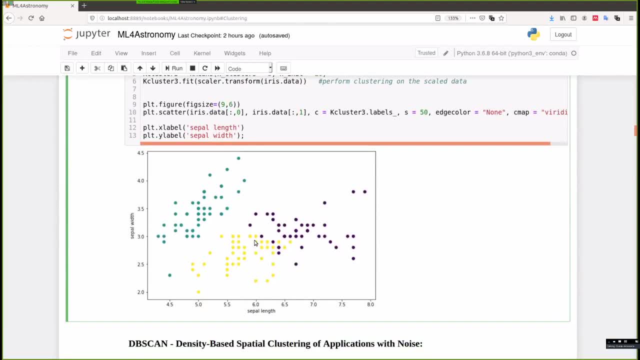 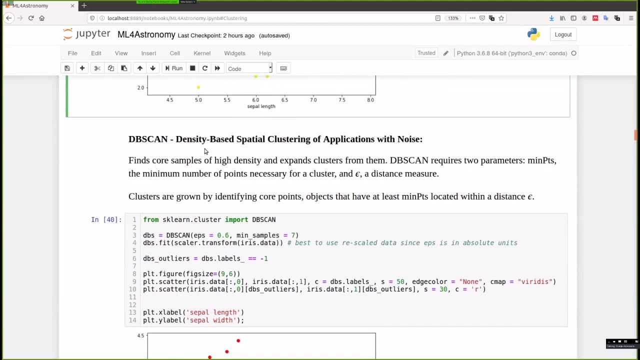 you can see that it actually looks more similar to the initial data set than when i did it without the- without the scaling right. feel free to stop me at any point, okay. another clustering algorithm is called the db scan. it's a density-based spatial clustering algorithm and what it does is to 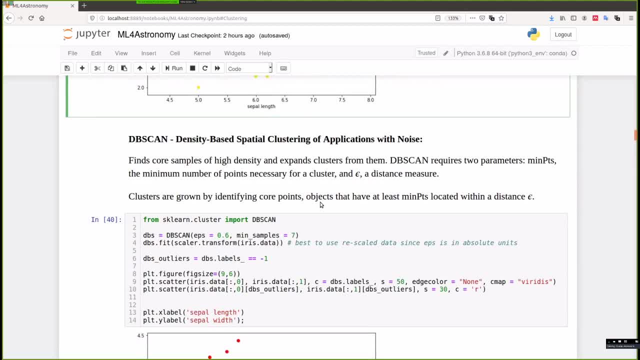 actually find a core sample of dense of high density points, which then expands from there to the to classify every source that is within a particular distance from this source. in this case you have to give two parameters to the algorithm. you have to give it the minimum number of points to associate to the cluster. so before i can define something as a cluster, i need 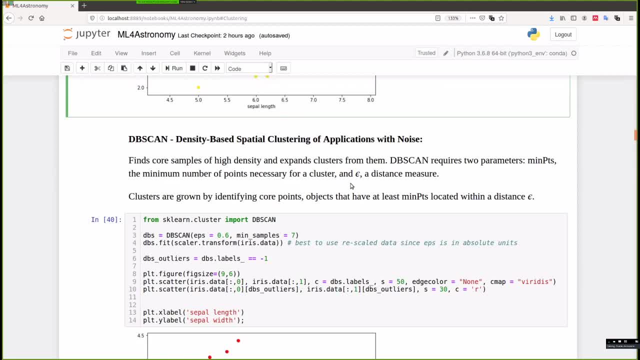 to have, say, seven points, 10 points, 20 points. you have to define this depending on the problem you're trying to solve. then you define how much distance in euclidean space, for instance, for which to associate things to a cluster. so you need to define epsilon here and the minimum number of. 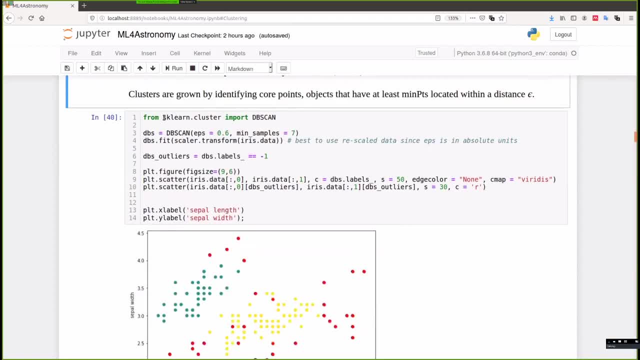 points to show to each of the clusters. um. so to try this also on the iris data data sets: um, i run it with an epsilon of 0.6. i'm scaling my data, so epsilon, now it's a scaled feature going from 0 to 1. so i can say 0.6 and i should shade at least seven points to a cluster. so if you find, 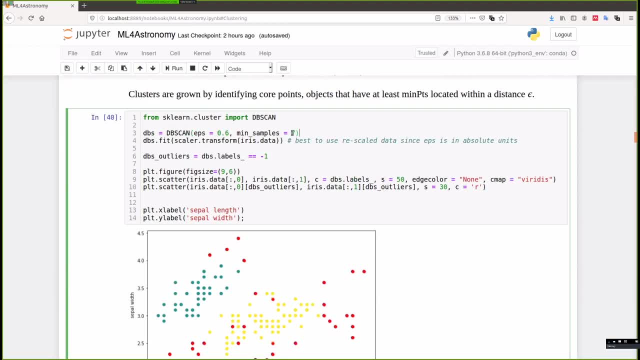 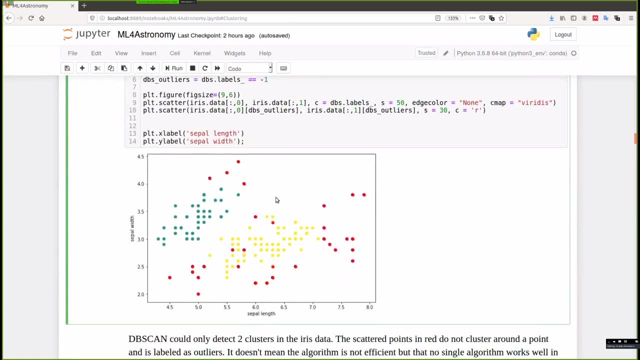 the cluster with, say, five points. it's not going. it's not going to have shifted to a cluster because it doesn't match the minimum requirements to be a cluster. running it on this data, you can see that it has kind of found out two, two clusters with some red points all over the. 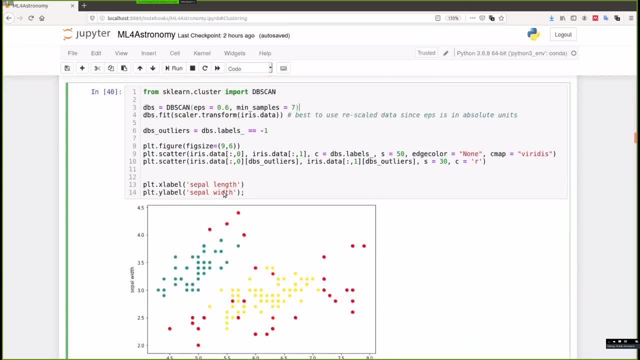 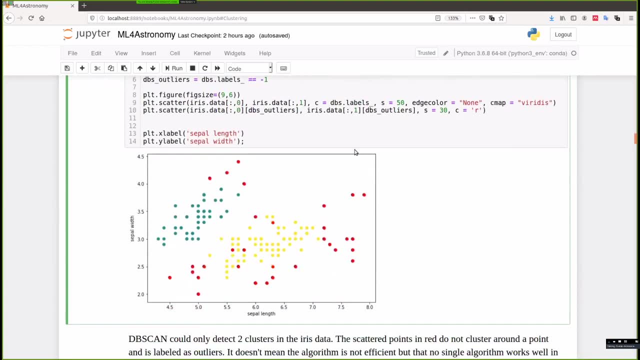 place which are labeled as outliers. in this case, if it cannot classify some of the points because they are not close enough to each other to form a cluster, it classifies them as outliers. all of the red points here are all around the place and they cannot close that to each point. this 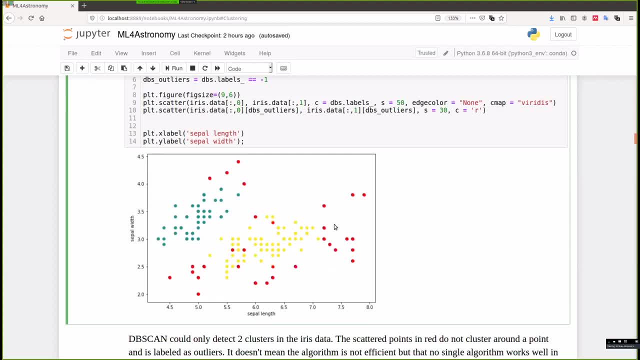 is why it is labeled as an outlier. so in this case, if you knew nothing about the data, would you say that the closed chain algorithm has performed very well? no, perhaps no, but you don't actually know. yes, but in this case, isn't the clustering algorithm very dependent on the 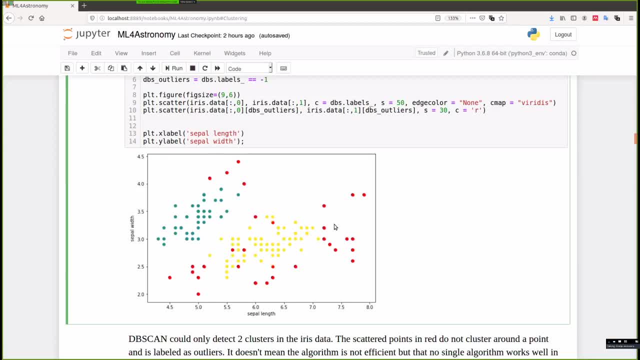 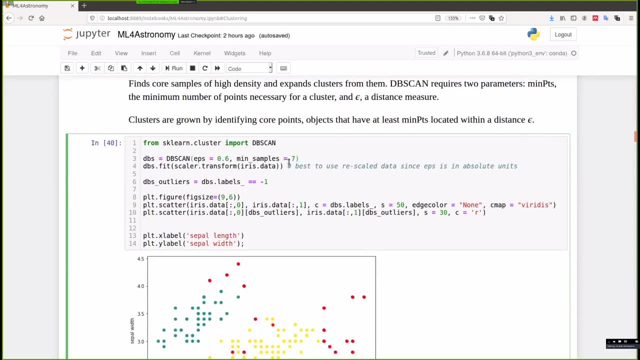 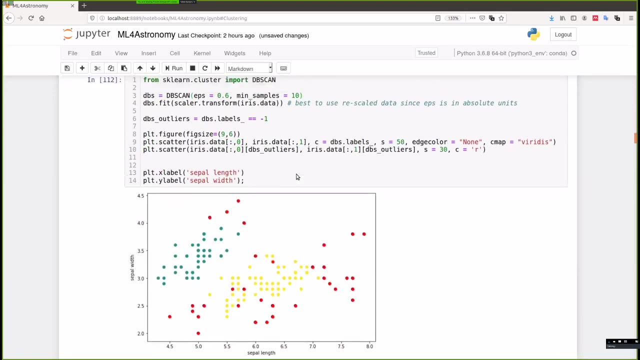 values that you use to initialize it. so, ah, but you mean the epsilon and the minimum samples. yes, yes, yeah, so that's possible. i can change this to say uh, to say 10.. the result is not so different, is it? no, sometimes they are not. they are not so sensitive, depending. 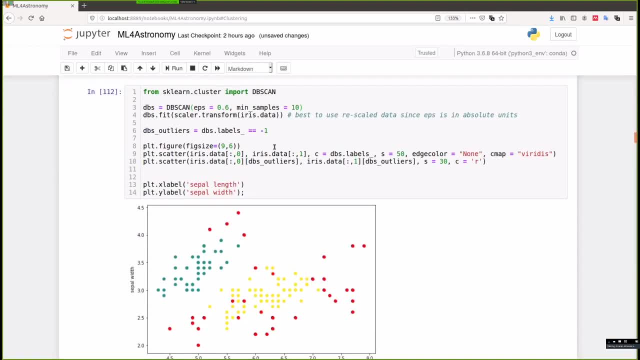 on the kind of data you're working with, which is why there are methods, uh that. so i trade over the samples to see how your, how your algorithm is performing, how sensitive it is to these parameters. so you can always do this to see, to see the values. you can see something. 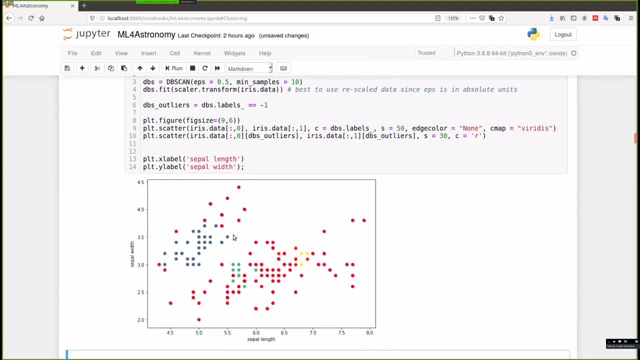 has actually changed here. now you find three clusters. the red points are the outliers. you can see it has found this blue and the green and yet, and the yellow which, which is still not correct, because now you have a high density of of non-clustered points, which are the red ones. 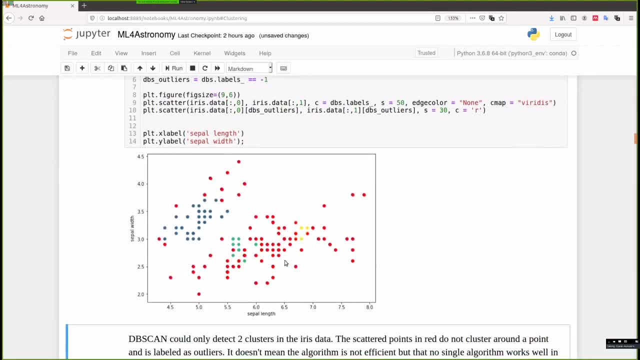 so it's my. the reason of putting the example here is actually to state that not all algorithms work the same, depending on your problem. you need to have a very good understanding of the problem you're trying to solve, to know which algorithm fits best. fits best and most cases. 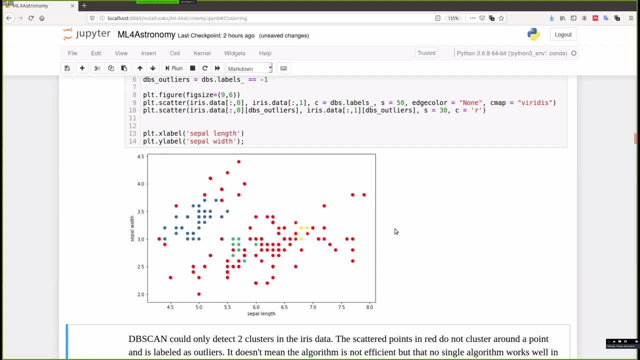 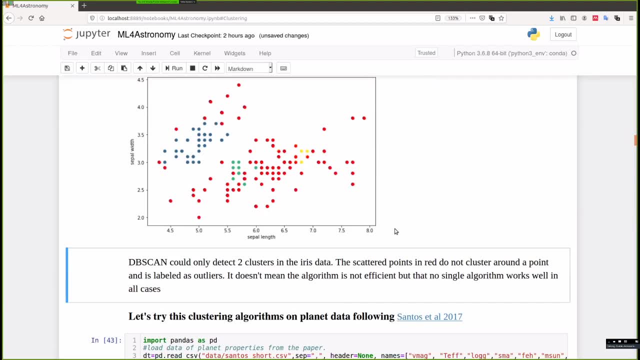 people never use one algorithm. they try they tend to use two to confirm the results from one another. so this was the single point here: that nothing works in all the cases. so there's no, there's no quick, quick pull pull out of the bag algorithm to use to solve your problem without actually knowing. 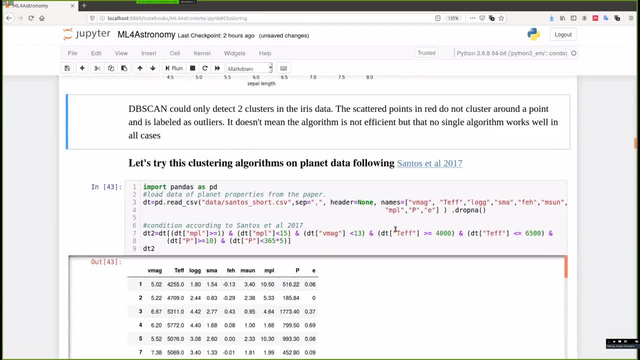 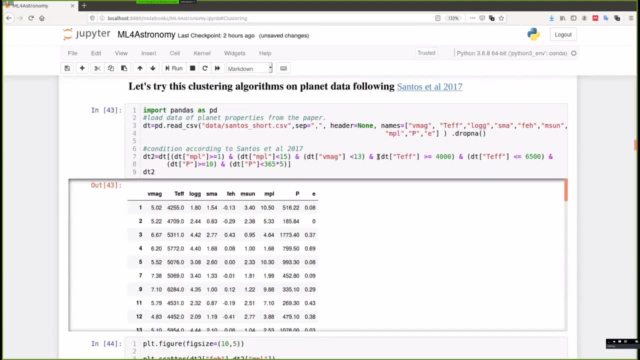 defining your problem in a very good space. but, knowing this, after all this astronomy, let's try to use this cluster as this clustering algorithm on some data. uh, there was this paper by uh santa cheto nuno, which actually tried to do some question based on some features of of planets. 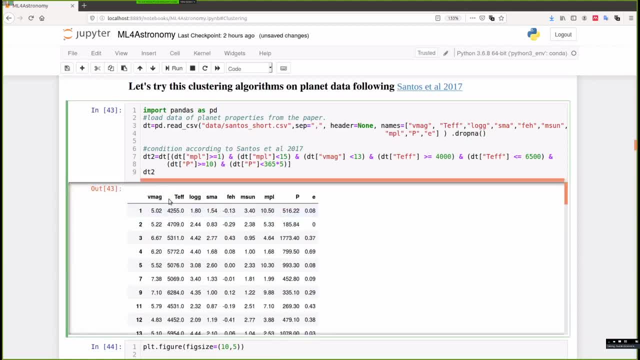 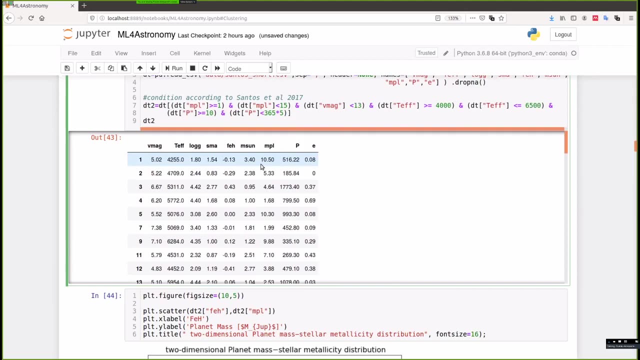 and i downloaded this data from the planets which includes the magnitude of the, of the of the star, the effective temperature, the log g, the same major axis and stuff like that, and i've actually done this criteria based on what they did in the paper. so basically, what they were trying to do was find a correlation between the metallicity of the star. 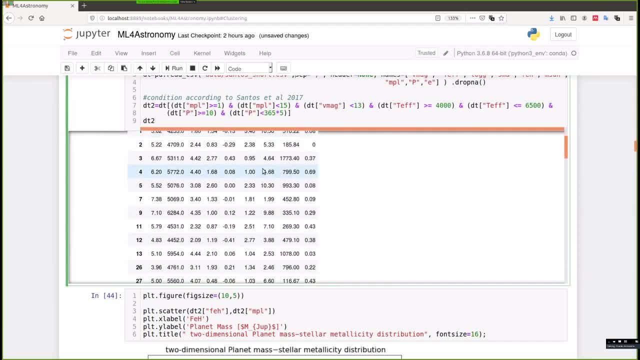 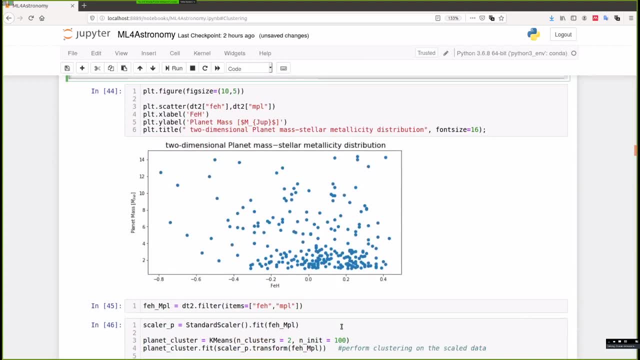 and the mass of the planets, and if i plug this data that they have here, it looks something like this: by eye, you can already tell that there's some sort of clustering for planets around two jupiter masses below here. but you need- you need something to actually delineate between the ones. 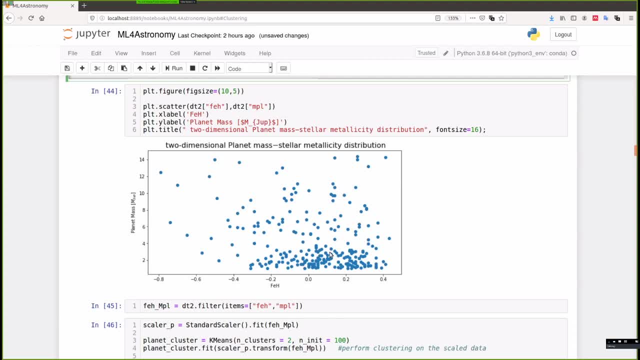 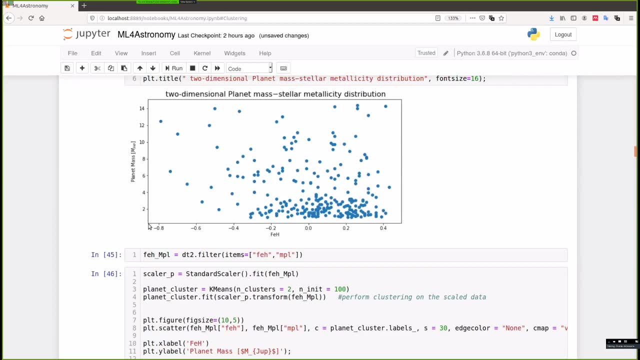 that are within this cluster and not within this cluster. so, if you try to first, i scale the data because, like i was saying before, the planet masses now go from 0 to to 15, which is a bigger, bigger one order of magnitude, whereas the metallicity is between is just one order of magnitude, right? 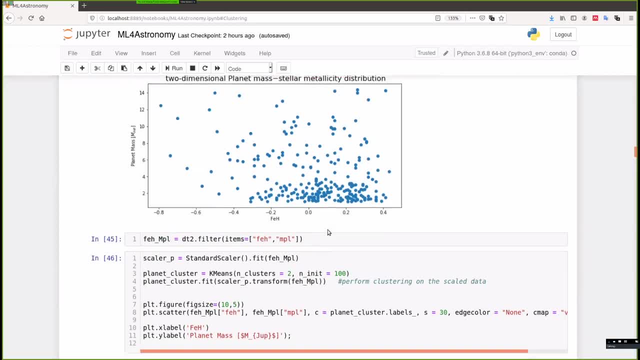 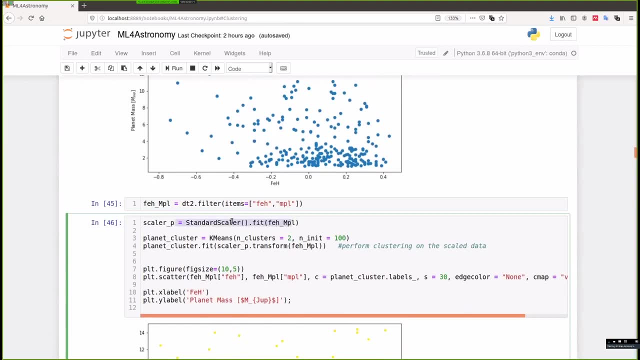 it's within that, within the same range. so i rescale. i rescaled the data sets here so that they both have the same scales. then i run caymans, which is the first algorithm we just did on it, assuming two clusters in the data sets. k-means actually has an algorithm method called the k-means plus plus, which it iterates over the. 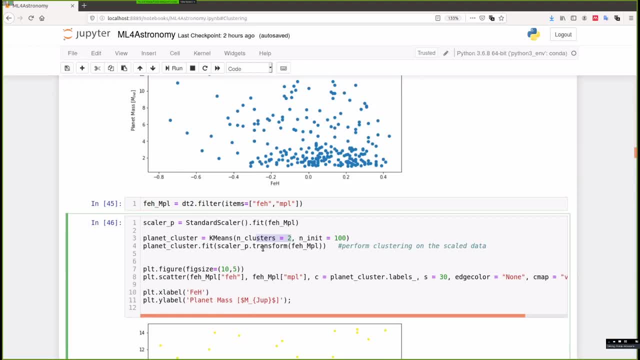 data set to find the best points to start as initial centroids of the data, because the output of the data can be very dependent on where you start from, so it needs this algorithm to figure out a very good space to start from to make sure that you get the best of of results running this. 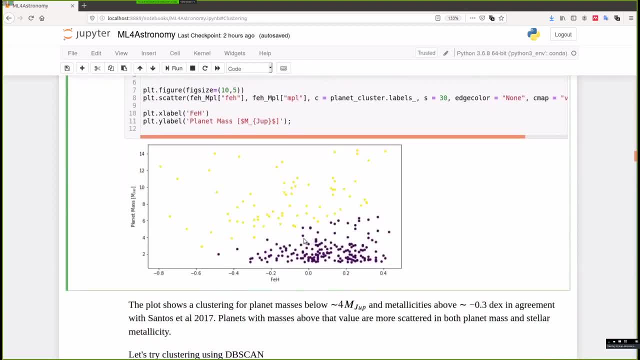 algorithm. so you can see that in the first case we have a cluster density of points at low mass and high and high metallicity. then you have some scattered number of points all around here, which in this case might infer two different population of planets, two different populations. 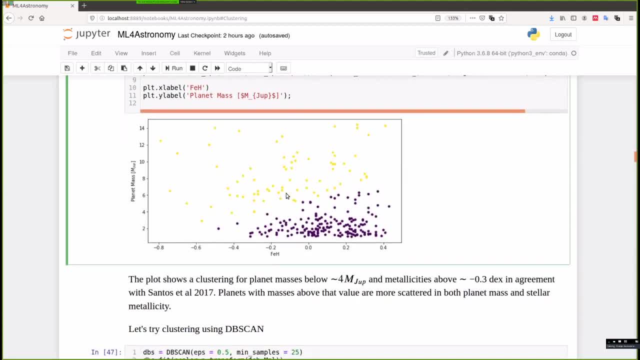 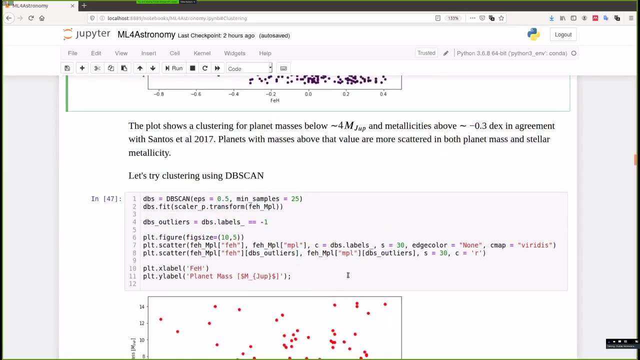 of giant planets actually, which was actually the the conclusions they reached in the same paper. that's: uh for planets, uh with masses below 4m jupiter. they tend to be around stars of higher metallicity than the others. so this is basically confirming the results of the previous paper. if i use db scan, which did not 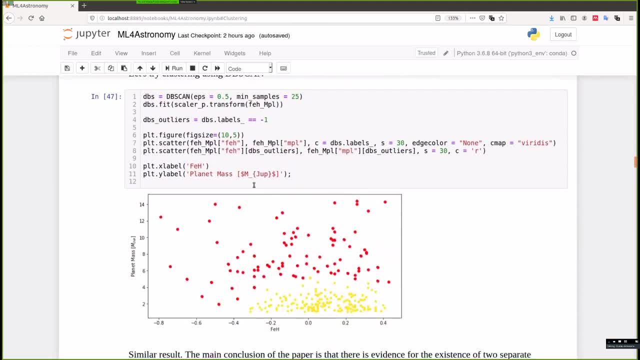 perform well in the previous case on this same data set. it provides similar results with all of the red points as uh as as outliers. in this case because i um, because i labeled it's and i find the cluster and labels the rest of them as outliers, so which was the case here in this case? 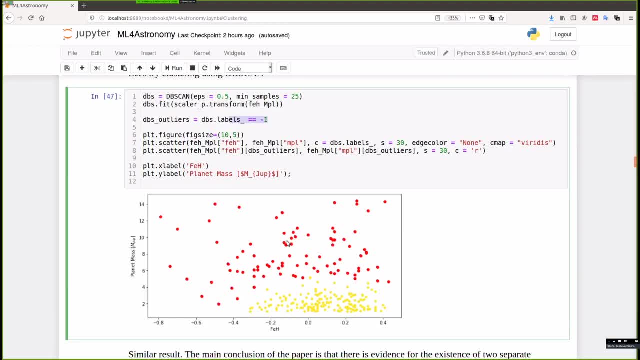 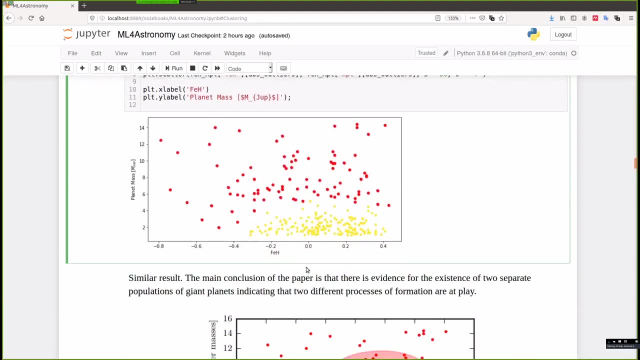 so what's been found? so what we've shown is that you cannot really call the red point clusters, because they don't stay around the same place. they're scattered all around the place and this is also in agreement with the result from the paper that's for for masses beyond. 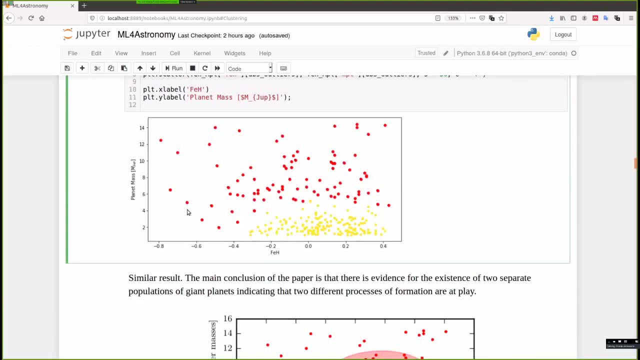 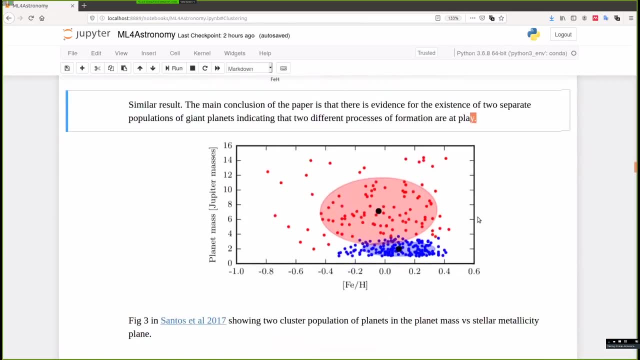 four, jupiter. they don't have a well-defined uh range of of metallic star metalicity that they have found it spread across the entire range, which is what they found. so this is actually uh, the result from the paper, which was exactly the same result as a question algorithm. so we can say for: 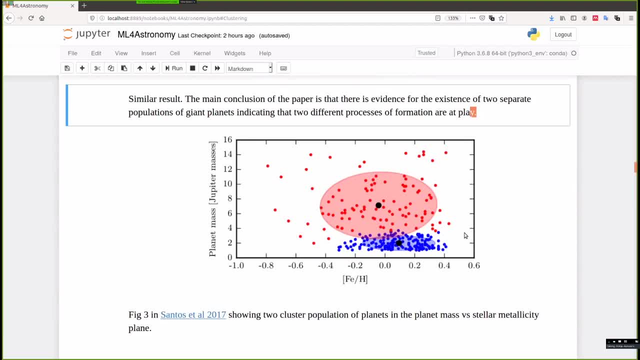 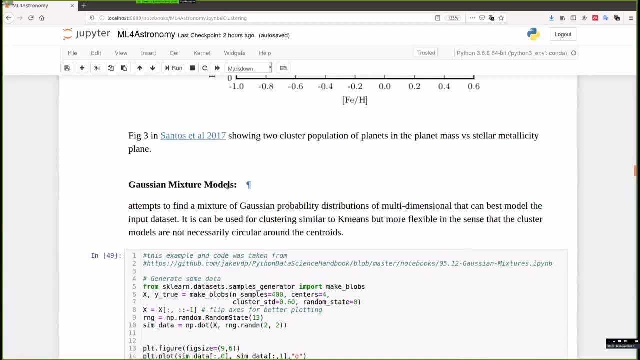 that these things can work right. i hope another method for clustering data is called the gaussian mixture models, which is actually what was used in the santos paper to actually cluster these points, but i chose to use something different, just to make sure that things are doing all right. 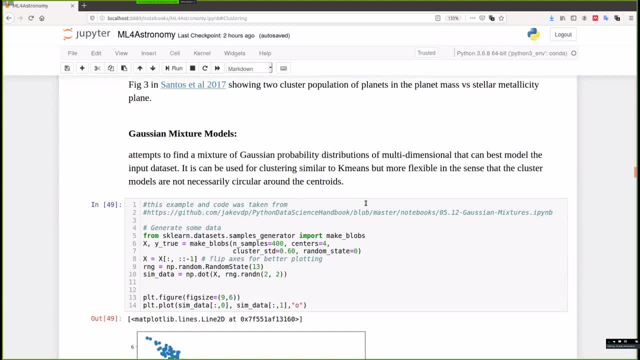 for the gaussian mixture models. it basically takes a mixture of gaussian probabilities of multi-dimensions that can best match the model. so in this sense it's kind of a regenerative, generative model in such a way that you can always reproduce the same gaussian distribution, the same. 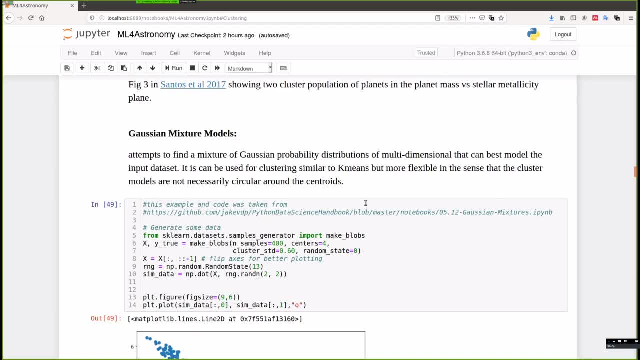 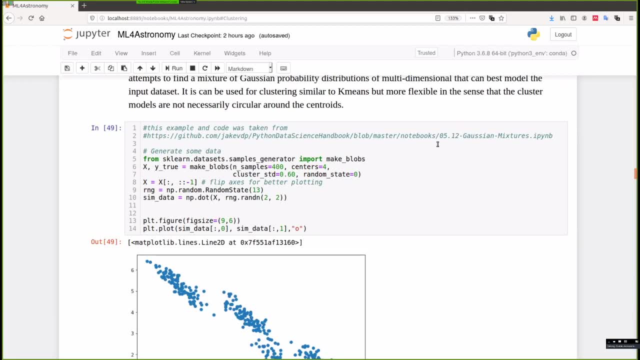 distribution that can explain the data. but it can also be used for clustering and it performs actually better than k-means because it doesn't have some of the limitations of of k-means. for k-means, if it goes out the centroid points then it draws a circle around it. 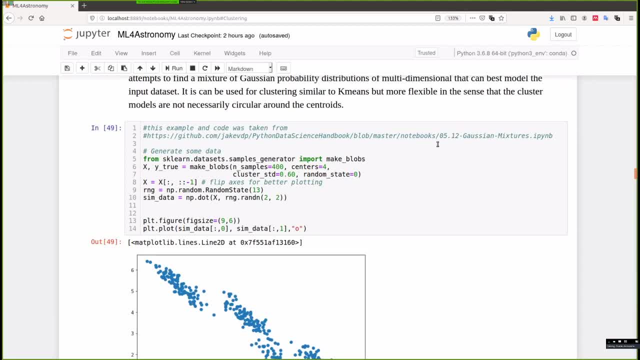 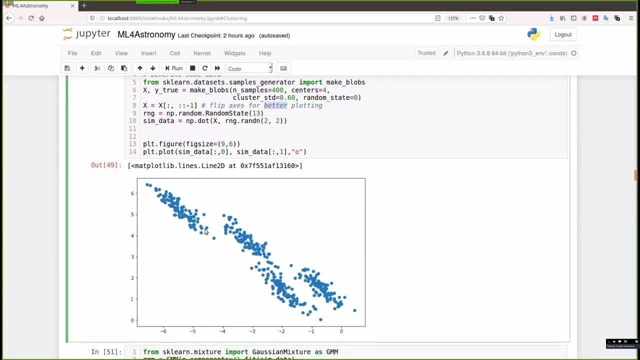 with the minimum distance at which it associates things to a cluster. but for gaussian, mr mr, you can have different shapes associated to the clusters. this is a, this is a simulator data here showing four different clusters which don't seem to form circular shapes, because if you draw a circle around the last ones over here, 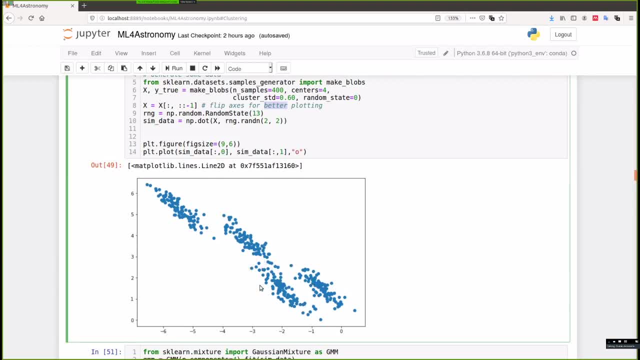 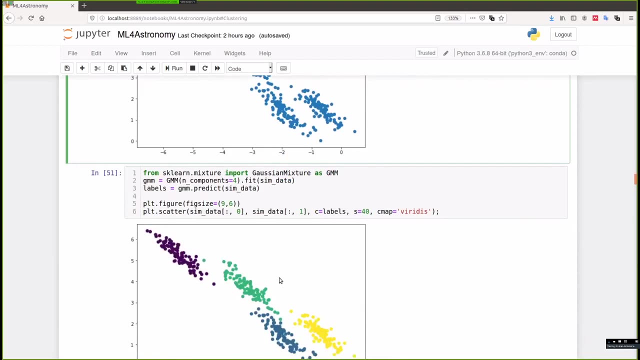 you'll see that there will be an overlap between two of the clusters which would be difficult for k-means to to to define, to define between each other because some of the points will be jumping into each of the clusters. but if we run gaussian, gaussian um mixture models on this gmm, you find that the the points are well. 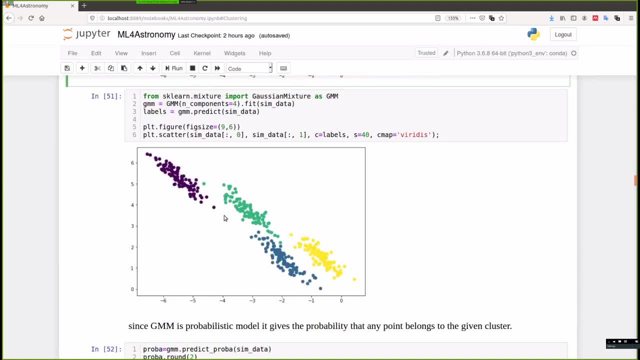 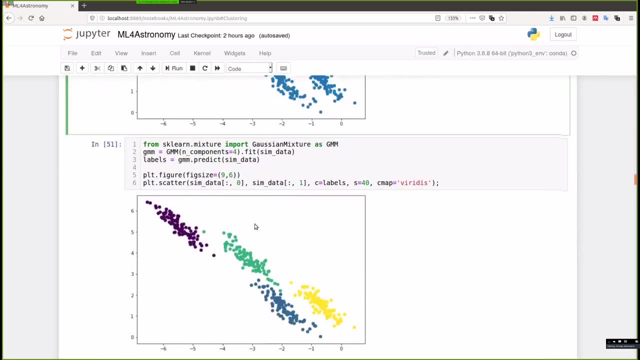 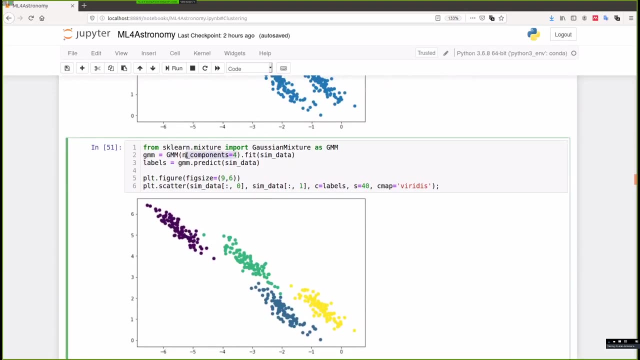 separated in the parameter space. yes, so this gives a very powerful tool to overcome some of the limitations of k-means. and gaussian mixture mixture model doesn't require you to specify the amount of clusters you're trying to find. it only requires to say how many components of the gaussian mixtures do. 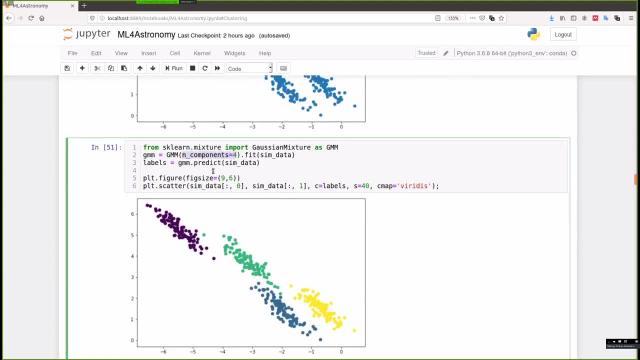 you want to use. the number of components do not relate to the number of of of clusters you're looking for, so it just means that you're using up to four gaussian distributions to explain these data, which could in any case, have need to use up to 30. i've seen cases where they use up to 30. 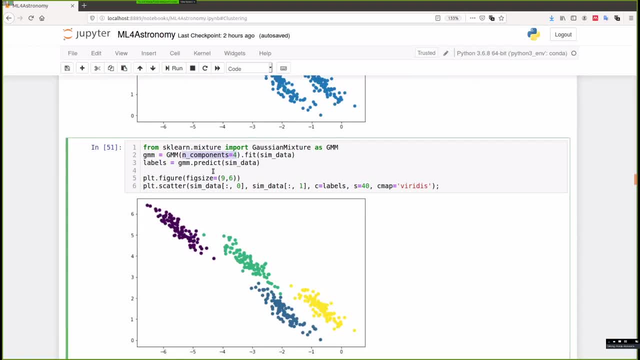 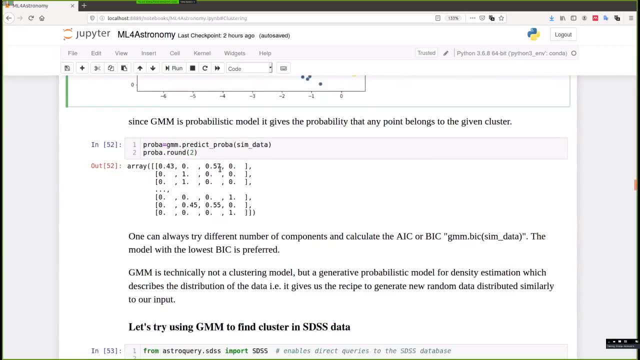 depending on the geometry of the problem, 30 gaussians to explain the distribution of the data points. and because it's a probabilistic model, it can tell you the probability of each of the points in the data set belonging to a particular data set. so if you run this, predict proper method. 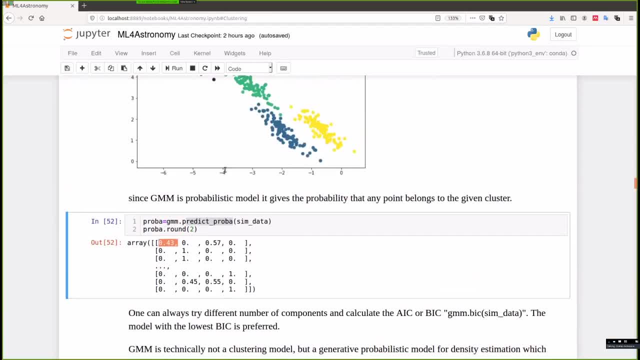 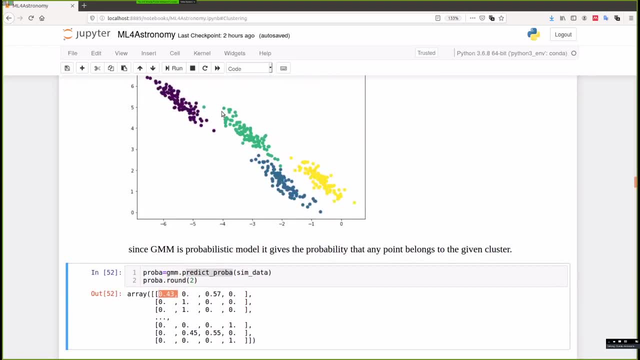 it can tell you that there's a 0.43 uh chance that say this point belongs to this, this cluster, and a zero percent that belongs to this one over here. what's a higher probability? that's 0.57 that it belongs to this one. so you know for a certain that it belongs to this data set based on the. 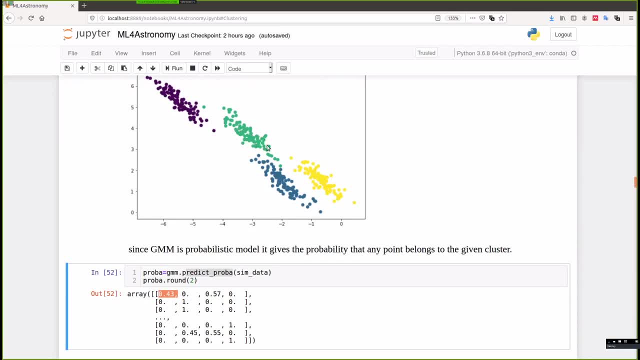 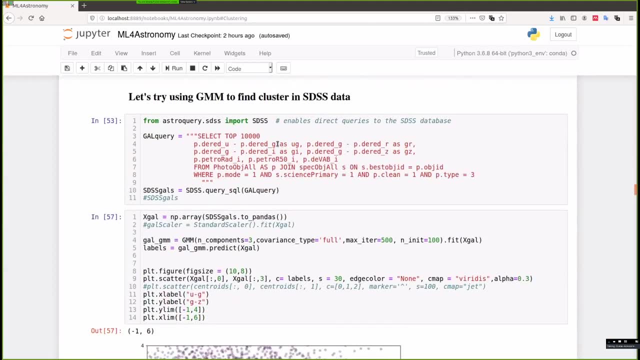 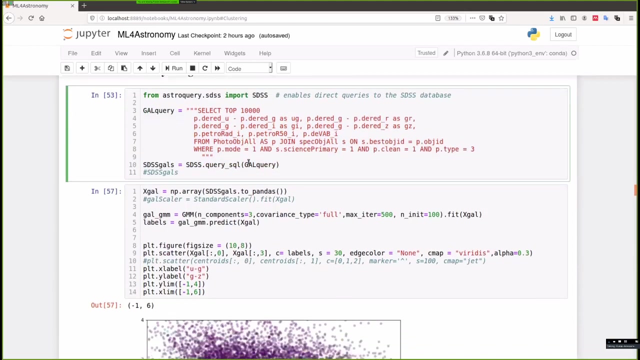 fact that it has the highest probability to belong to this cluster. so another astronomy example: let's use gmm on the slow and digital sky, soviet data. so i've run this, this query, basically to download 10 000 points from sdss sdss website outlining different properties of stars or 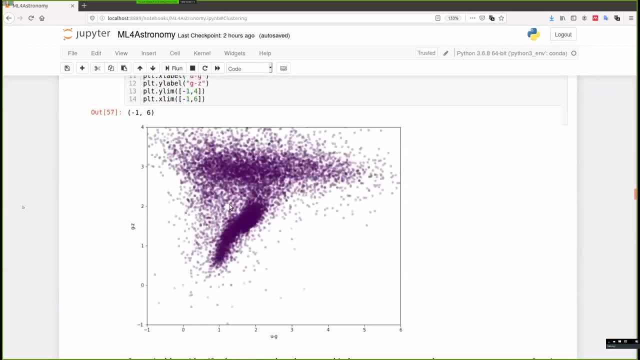 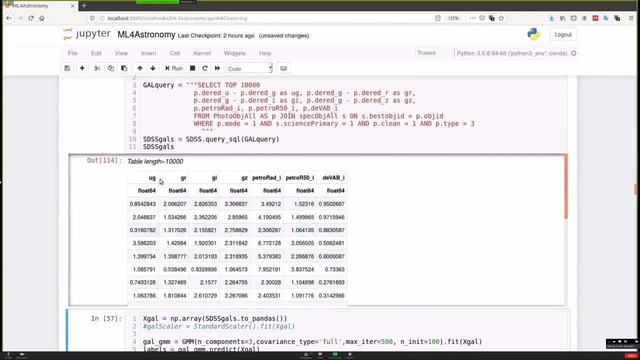 galaxies. um, i thought i printed it out somewhere. okay, let me make a print of this. okay, so the ug u minus g color, the g minus r- these are all spectroscopic uh filters that are used in the solver. g minus i, g minus z- the real details are not very important. 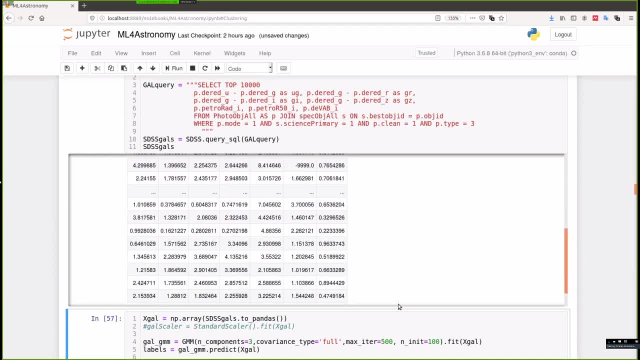 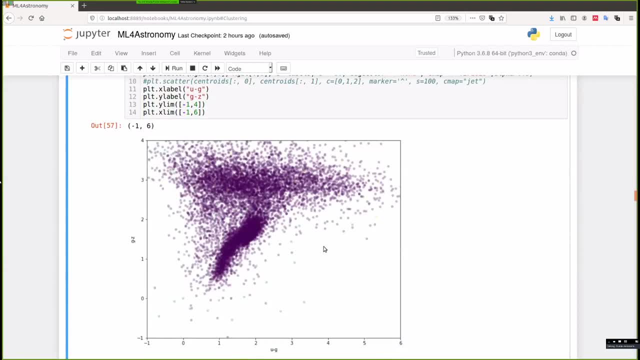 but i tried to use gmm to cluster these data points but voila, i was not able to cluster the points. no matter what i did, the points did not close. that, even though by i you can tell that there's a kind of cluster of points down here and another one up here, but my gaussian mixture does. 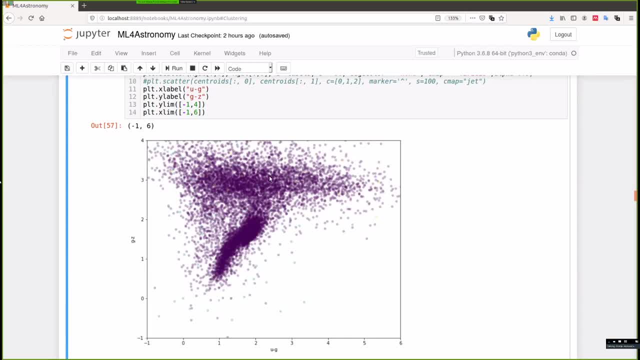 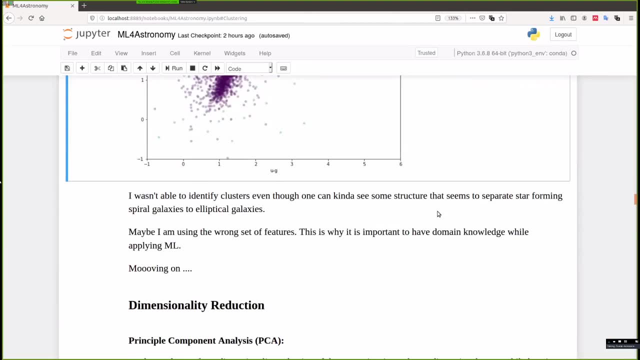 not do anything very well. what is the point of showing this is to tell you that i know nothing about galaxies. you know i don't know anything about them and i can't tell you anything about the galaxy. you can only do whatever you're listening to. so if i wanted to say like a man, i can't do it, and i'm doing this is to tell you that you have. 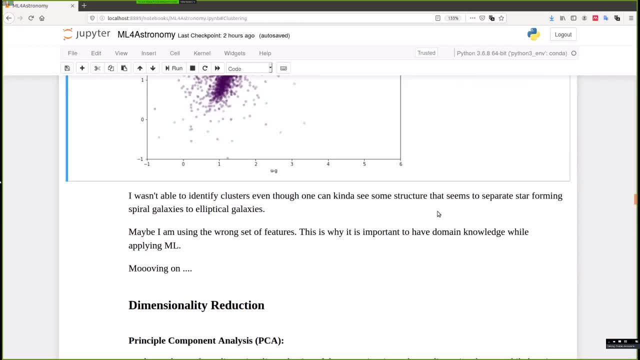 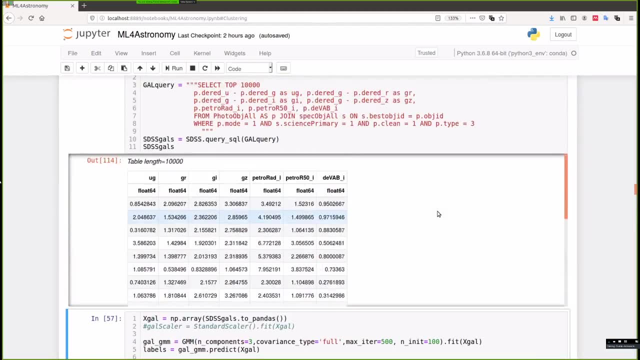 to consider a lot of things in order to have the best and the best data set. you need to know- i think this is a good point- and you can't do a lot of things in order to cluster them, so at some point, you need some level of domain knowledge in order to pick the right features. 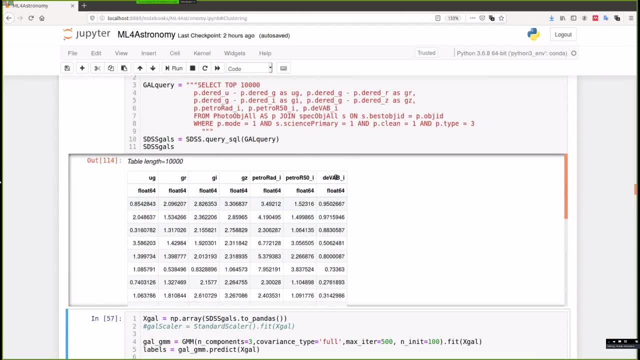 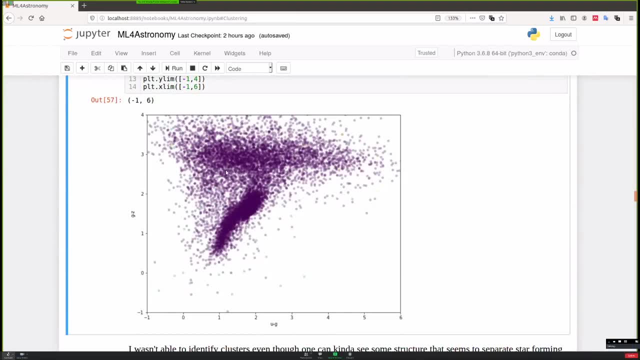 to close out your data points. the algorithms would not do any of these things for you. you need to know the best, the best data set, the best features that can tell you something about your data for here, for if it's providing the cluster and those other points. 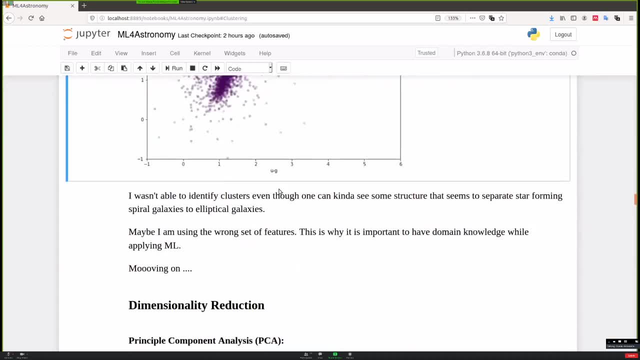 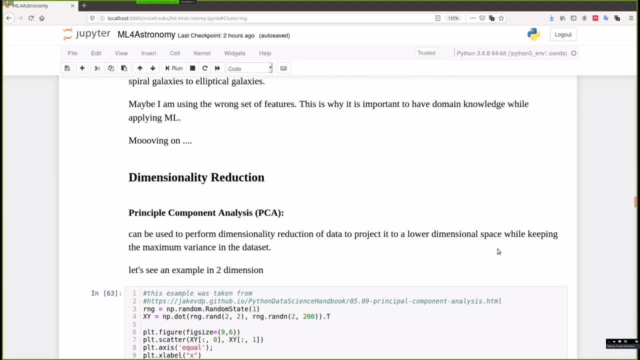 I don't know, But for this, I know nothing about it, So it's very important to know something about your data. There are some other clustering and unsupervised learning models, but I'm going to stick with these three within this paper. 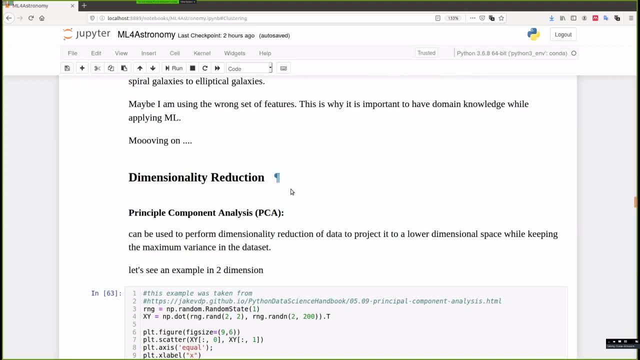 But another thing you can do with unsupervised learning models is to do dimensionality reduction, which is to reduce the dimension of your data In. there are cases where your data is in a 64 dimensional space and you need to be able to visualize. 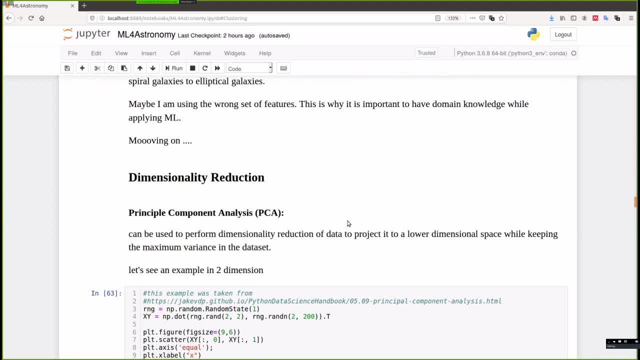 There's no way you can plot something in 64 dimensions right- At least in my case- So you can use dimensionality reduction to bring them down to two dimensions or three dimensions, which is something you could actually plot, And principal component analysis is one way to do this. 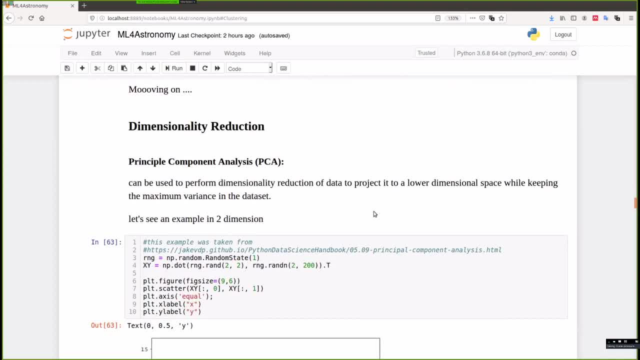 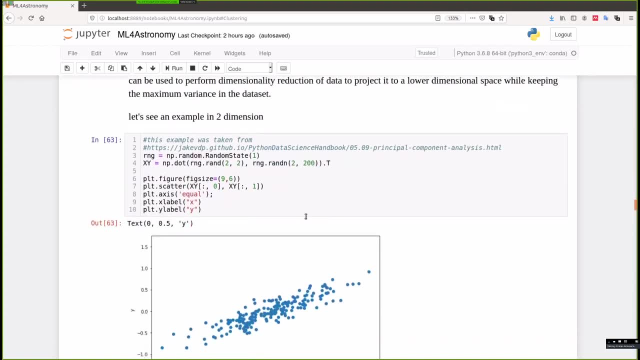 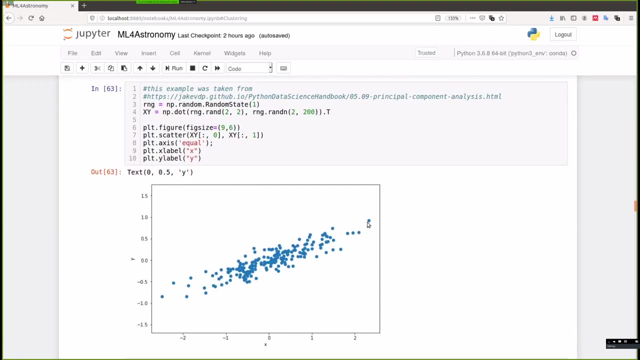 It has a way to actually reduce the dimensions of your data in a way that it still preserves the highest variance in your data, which is the most interesting feature. Taking some random data sets, which really doesn't matter, within X and Y axis, you have this data in this way. 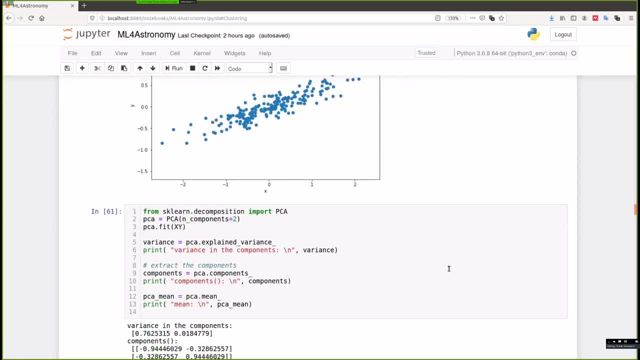 and you want to see the components of this data along the X and Y axis If you run the PCA. and another thing to mention is that most of the methods within SQLen they use exactly the same way they are called, So you don't need to necessarily learn so much. 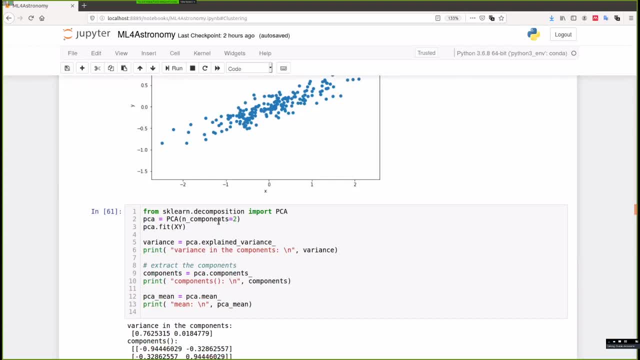 about every method in order to use them. You can see, usually you just initiate the model using something like this. then you fit it to the data directly. So now I'm fitting a PCA using two components, because this data is in two dimensions. 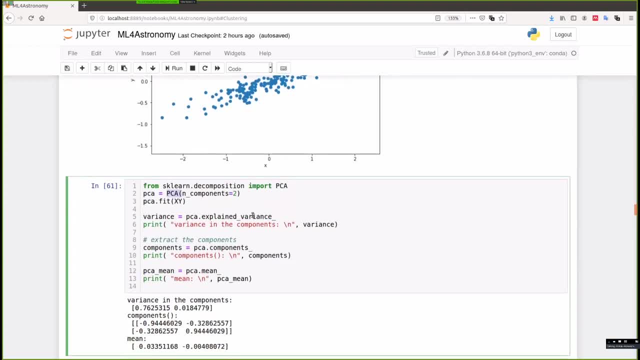 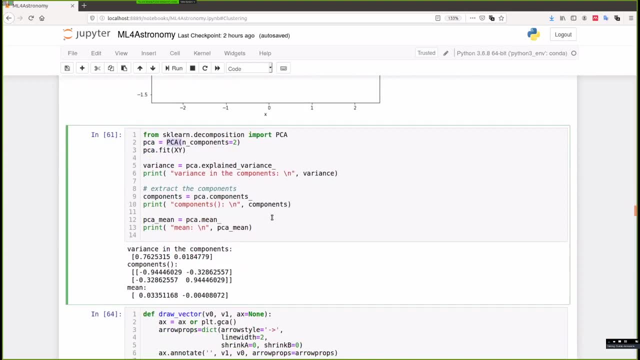 So these data sets and what it gives you is the explained variance in both of the dimensions of the data and the components in those dimensions. You can see the variance in the data set here is 0.76 in one dimension and 0.01 in the other dimension. 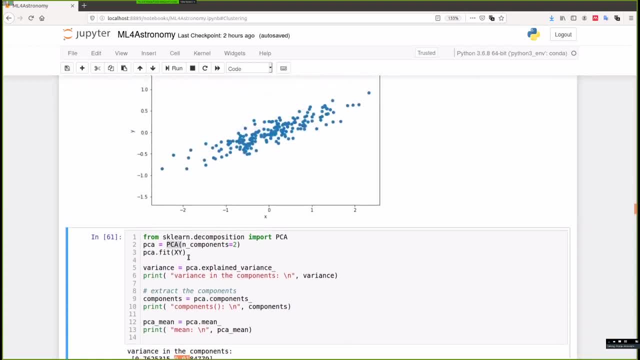 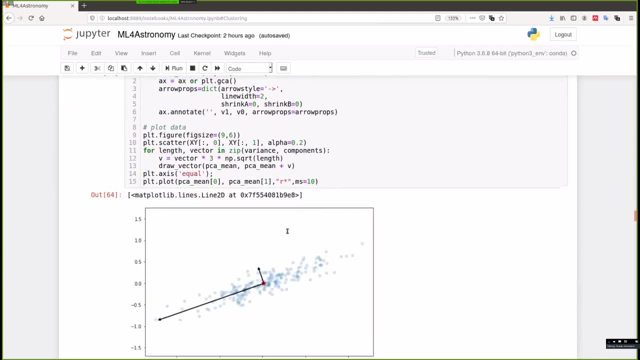 You can already tell that you have more variance along the X axis here than you have along the Y axis, which is what the PCA just gave us. So if you draw the vectors along this, along the data set, you see that there's more variance along here than here. 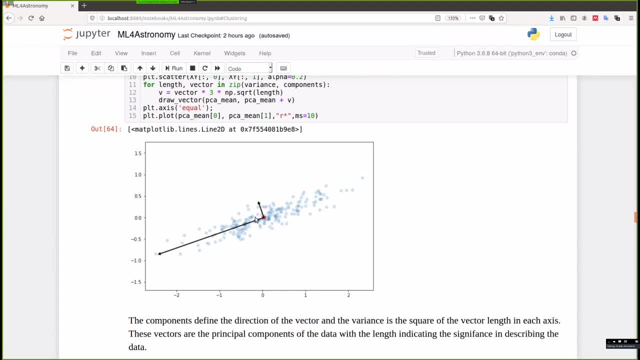 So if PCA were to reduce the dimensions of this data set, it will suppress the smallest variance in the data set And if you had more, it will actually keep suppressing from the smallest variances to the top, because it needs to preserve as much information. 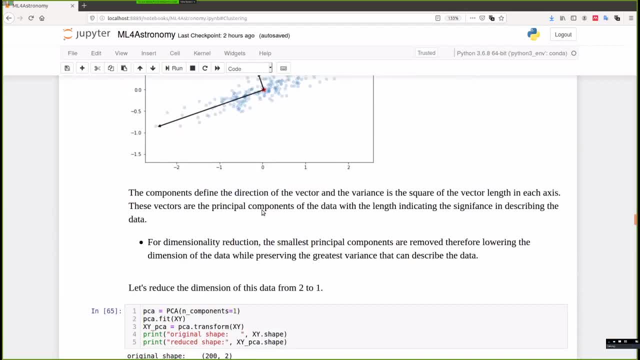 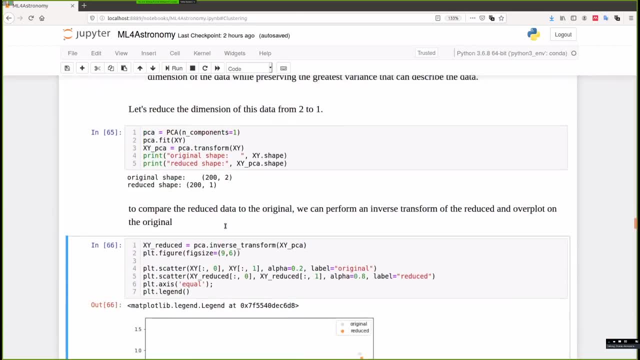 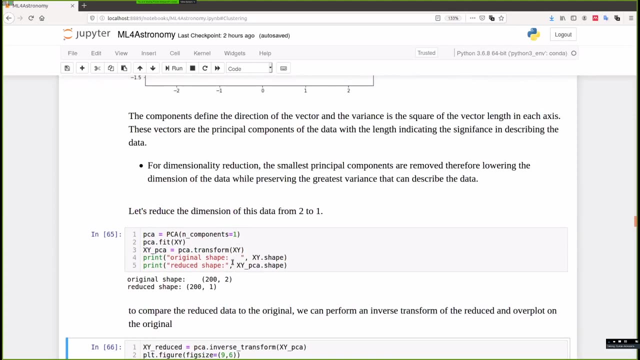 about the data set, as is possible, right? If you then try to project this data, they reduce the data. Ah, okay, Now if we were to reduce the dimension from these two components to one component to one dimension, you would run PCA in this way. 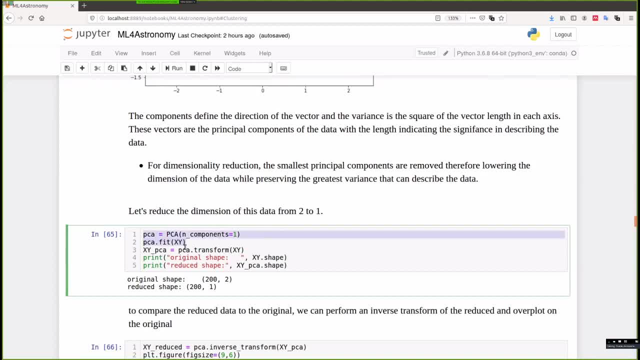 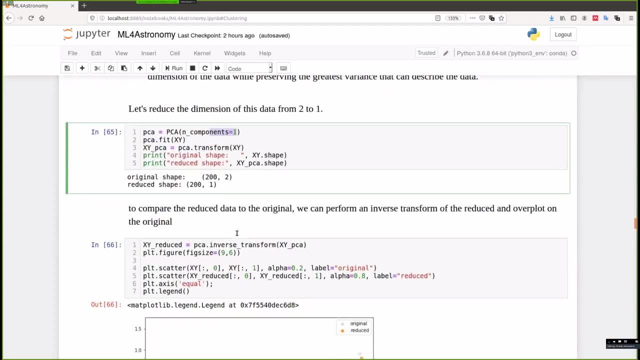 Previously I did PCA with number of components too, because I wanted to see both of them, But now that I'm sure that there are two components, I can reduce them to one component using this And, you see, it goes from an original shape. 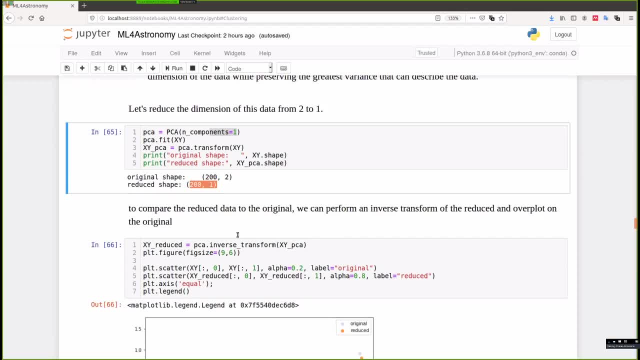 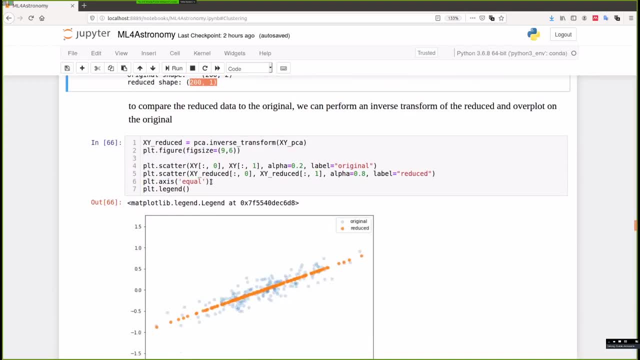 of 200 by two to 200 by one, which means I've surprised one of the components of this data And if I plot it on top of each other, you see what the new projection of the one dimensional component is on top of the other one. 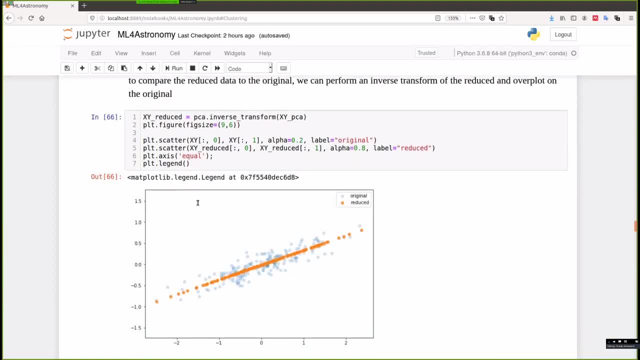 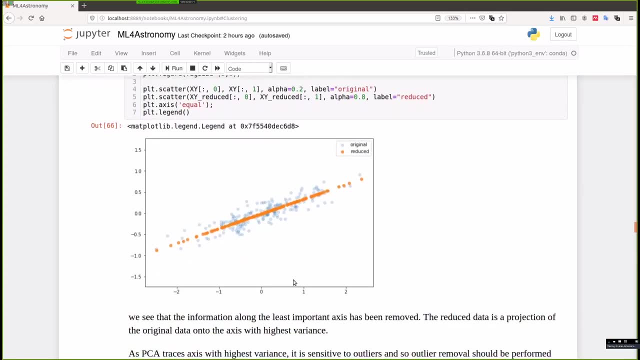 So, in basically, I have reduced this data, but keeping as much variance as I can within one of the axis, And this looks very much like a fitting solution right, So it can also be used to fit into data, which this, I reckon, will be a very good fit to this data. 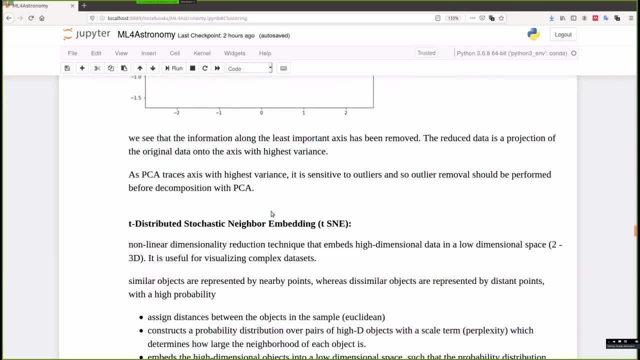 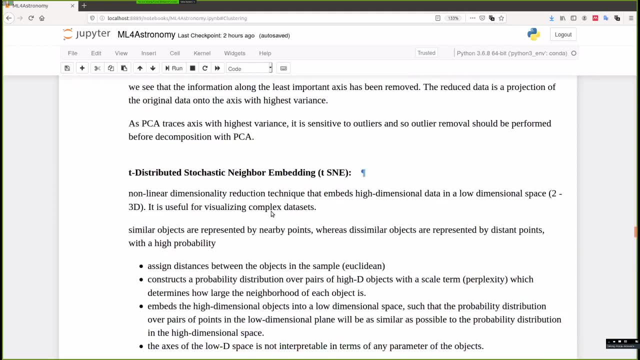 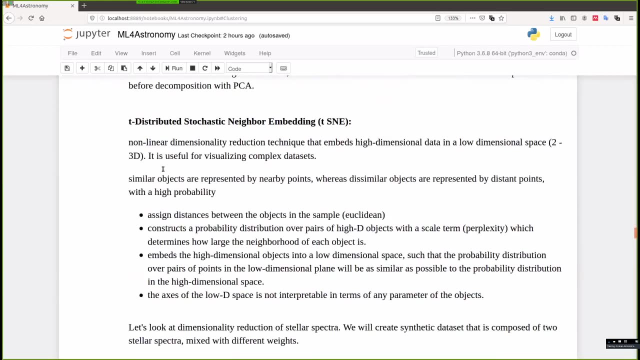 To show another example of what dimensionality reduction can do for astronomy, I'm going to use another method called the t-SNI, the t-distributed stochastic neighbor, embedding t-SNI. it's a difficult thing to say, not so usual thing to say, but it works very well. 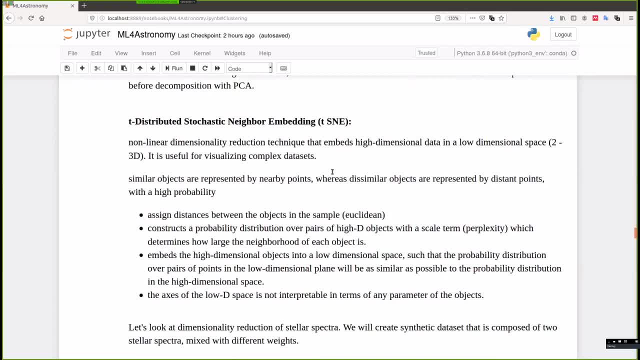 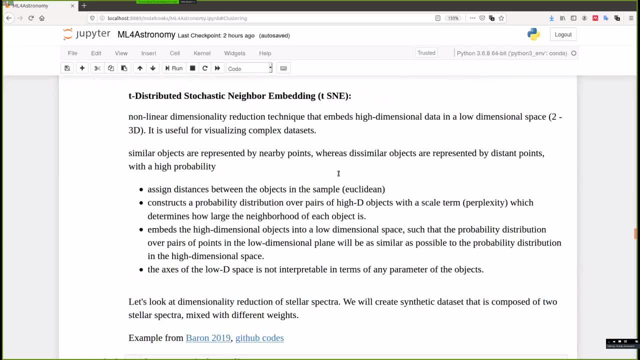 What it does is it performs nonlinear dimensionality reduction to embed high dimensional data into a low dimensional space. In a way. it does this in a way that, despite the large dimensions of the data, the reduced data still have points that are similar to each other. 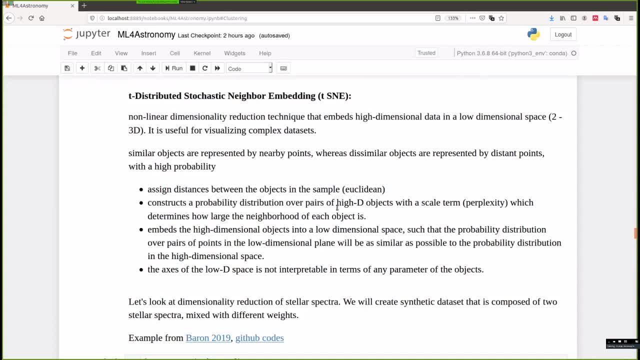 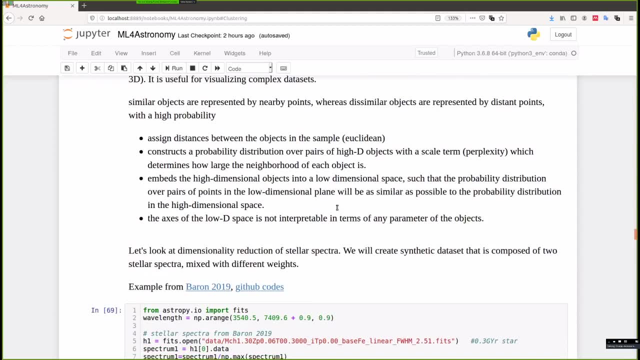 close to each other on the reduced data space. So what it does is to assign distances between each object, construct a probability distribution with an over a pair of the points. Each of the points has a probability of being close to each other or far from each other. 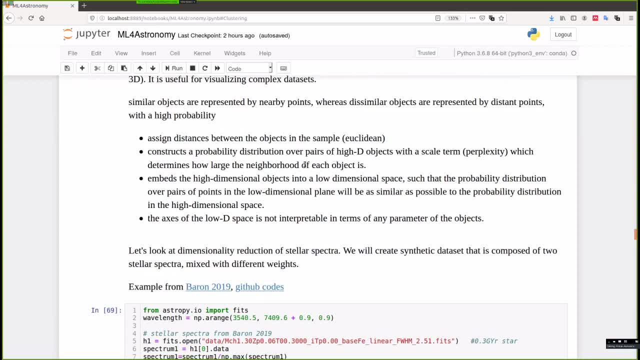 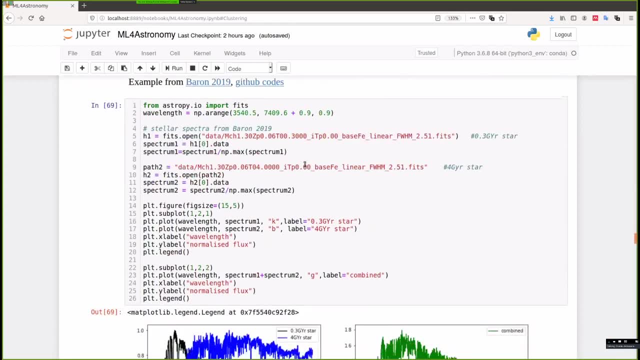 Then you embed the high dimensional data set into a low dimensional space, knowing the probability of it being close to each other or not. An example that I'll take for this is two different spectra- blue and green in this case- which I took from some source online. 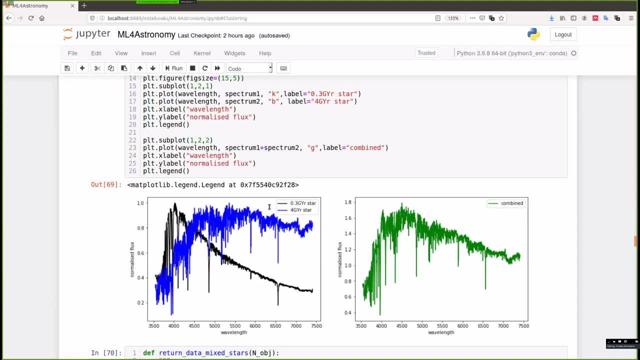 The blue one represents a very old star- four giga year- whereas the black one is a young star with a young star. If I mix both of these together, I get this green data set. What I'm trying to do here is to mix this two spectra. 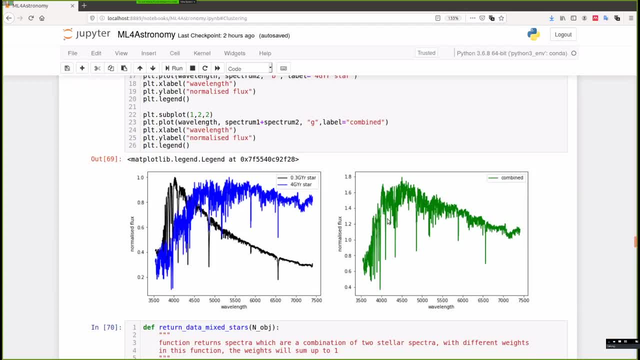 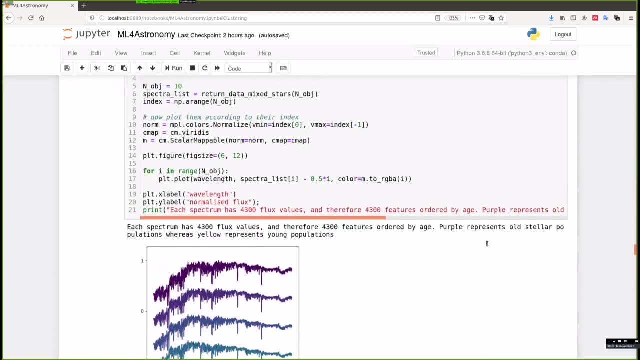 in such a way that I have different spectra with different ages mixed together. So if I do this, mixing them with different weights, in the first case I have a weight of zero for the young star, so that it's exactly a young star. 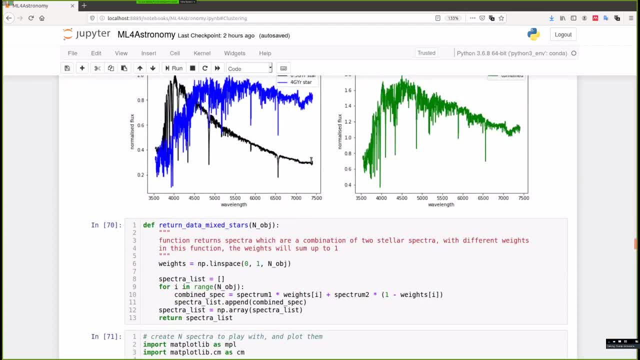 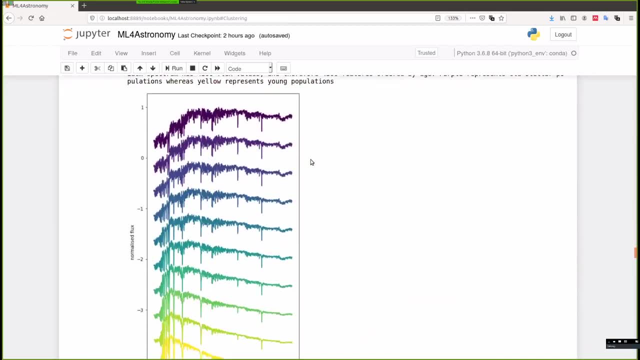 In the other case I have a weight of one, one to 10, between zero and one, basically to have different ages of the star. In this case I create 10 different spectra by mixing them both with different weights and it goes from the youngest star in yellow. 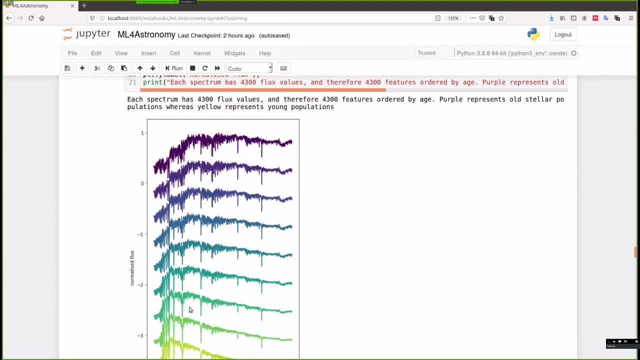 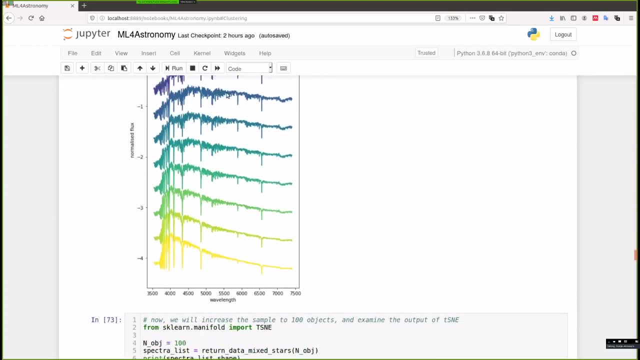 to the oldest star exactly four giga year in purple. So from 0.3 giga year for yellow to four giga years for purple. Now I'm going to try to represent this information by reducing the actual parameter space. 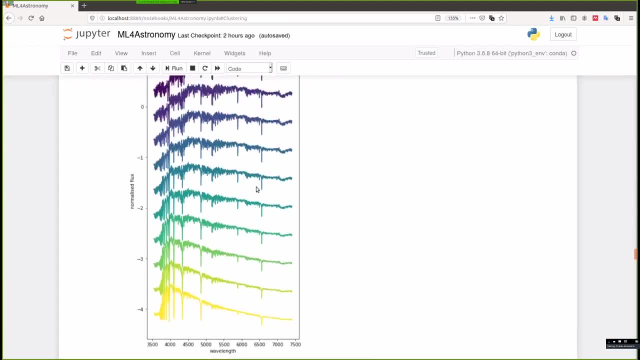 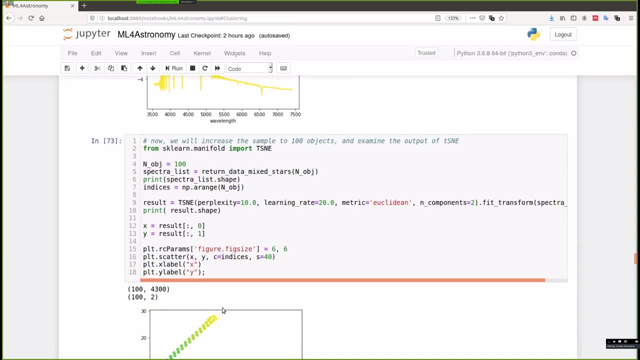 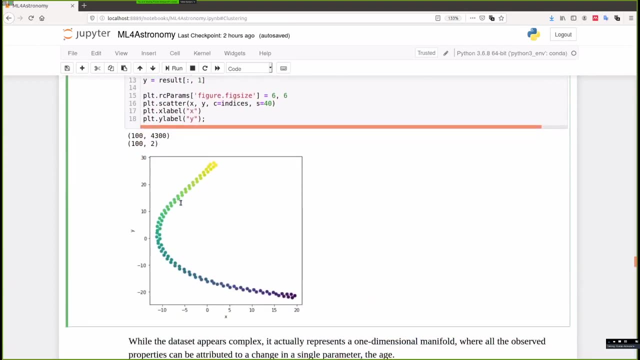 In this case, now, every single point within this spectra, that 4,300 points, is a particular feature that needs to be reckoned with within the algorithm. If I reduce this data to two dimensions using this t-SNE algorithm, I can represent the whole data with just this plot. 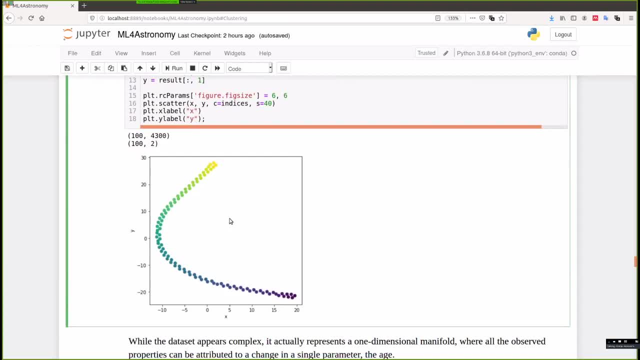 You can see. what it has effectively done in this case is to associate, without knowing any of the structural data, because I do not tell you the ages of the spectra. is to associate each of the spectra with young age in the same parameter space. 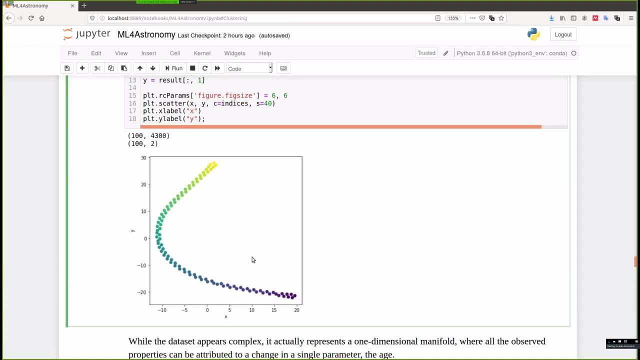 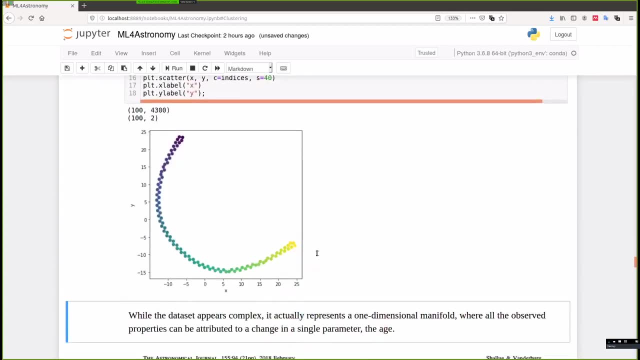 And all of the old stars- the purple ones- have been associated together in this space. This algorithm doesn't always produce the same shape. I can run it a second time and I'm going to have something different. It's a bit different from the first. 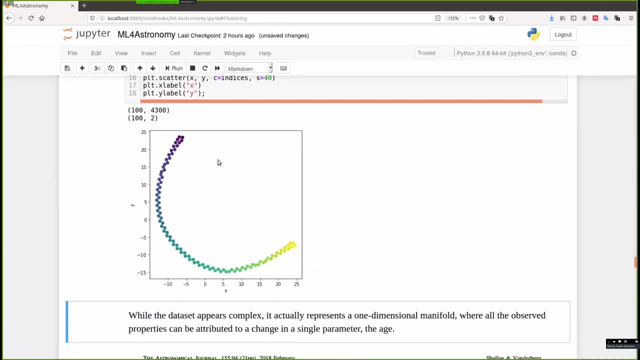 But one thing is always to understand is that it puts objects that have high similarities in the same parameter. space X and Y in this case means absolutely nothing, because they don't refer to anything specific about each of the spectra. It just tells you in Euclidean space. 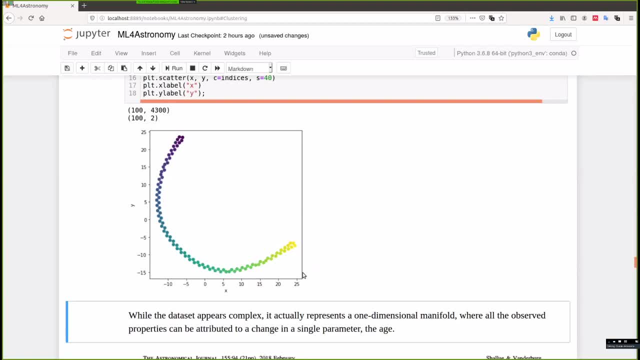 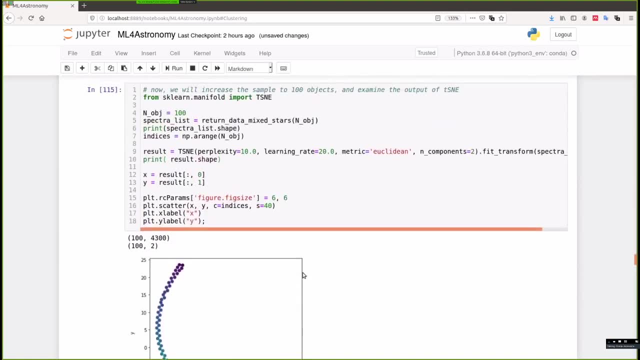 how close enough to each other. two different data sets are to each other, So you can know how to. for instance, if some of my science required me to use only young stars, I wouldn't have to go through a million spectra of different stars to actually figure out. 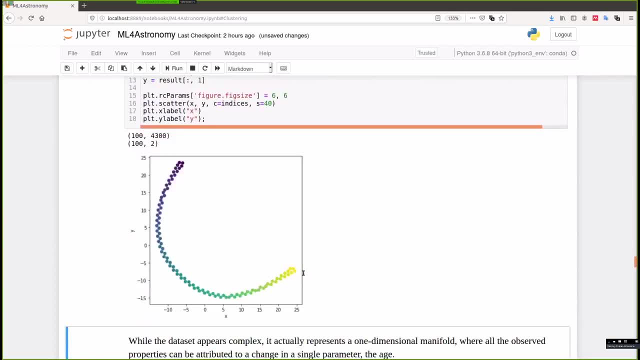 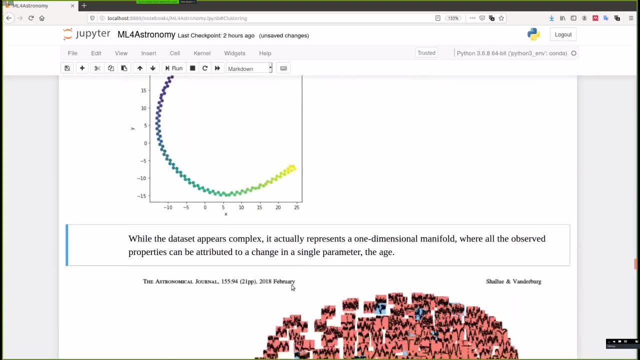 which ones are old or young. I could reduce the dimensions and I could reduce the size. I could reduce the dimensions and only take out data sets with that fall within a region that I'm interested in, So while the data set actually appears complex, 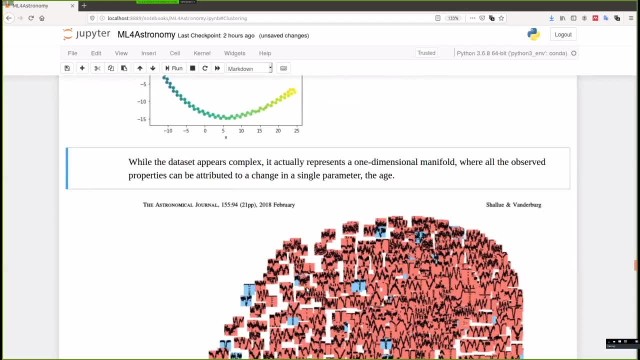 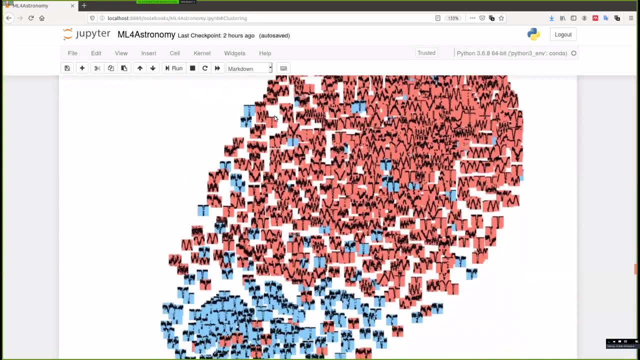 everything could be represented in a manifold where only the age is the deciding factor of how close enough to each other. each of these data sets are A very good example in my field is in planets, is in detection of planets. Taking, say, light curve data from Kepler. 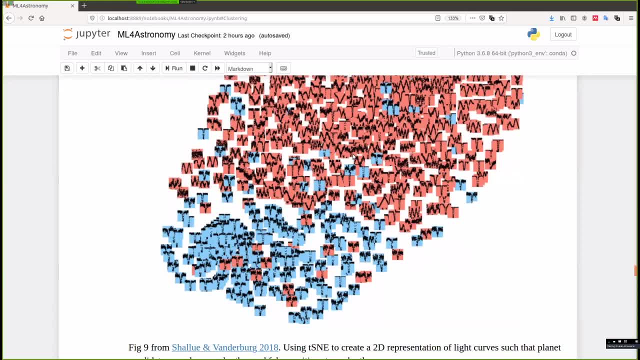 you can plot all of them using t-SNARE and it tells you, for instance, which light curves contain planets transiting the star and which ones do not, or which ones are anomalies. In this case, this paper by, I think. 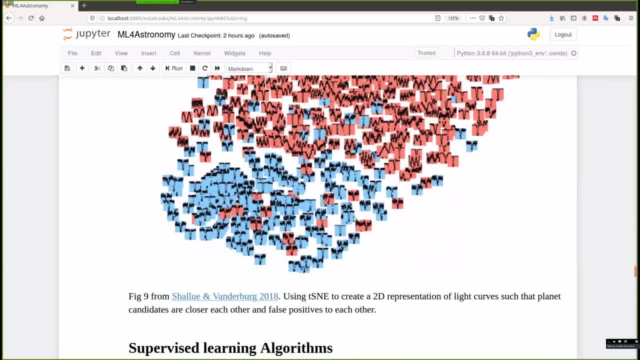 Shalloway and Vanderburg. they use this t-SNARE to separate out planets that have other systematic sources and ones that actually have planets clustering around each other, And you can see the planets- the planet candidates, actually fall in a parameter space. 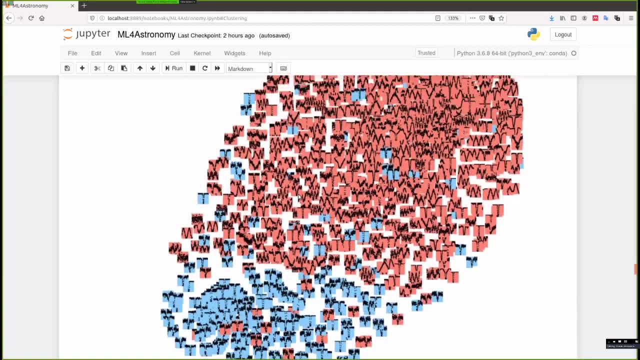 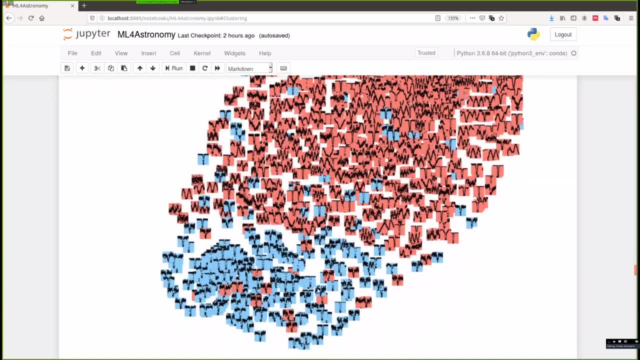 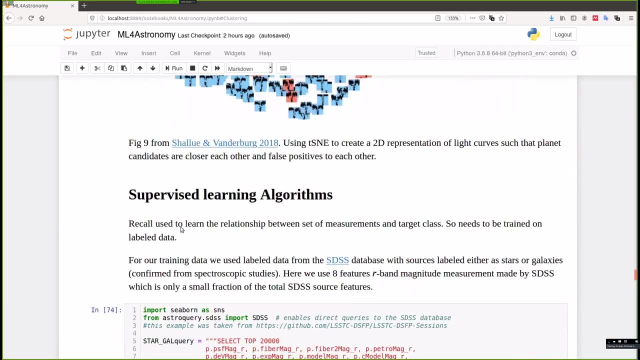 that are close to each other than the other cases. So if they had to actually do further analysis of this planet, they only have to go to the planets, to the data points that fall within this parameter space of the reduction. Oh, time is running really fast. 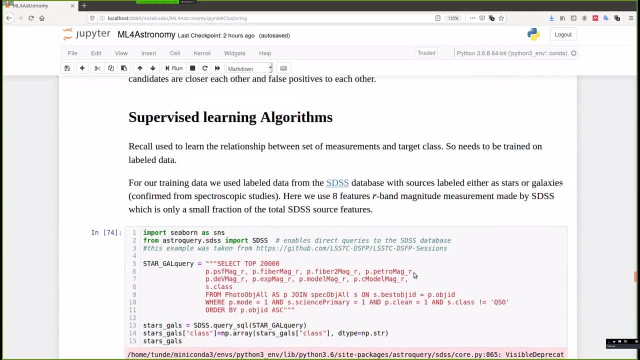 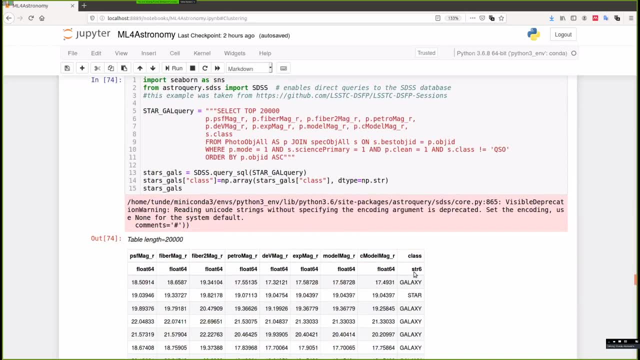 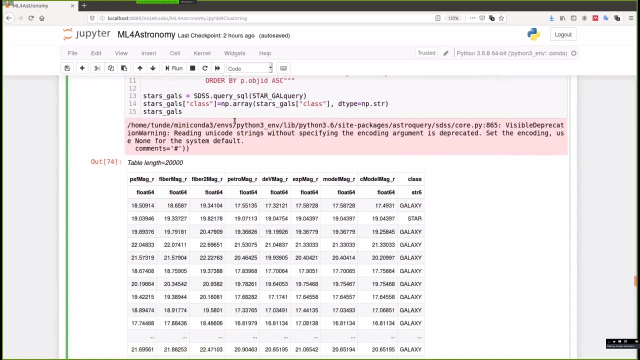 Now to go to supervised learning algorithms Again. now, even though I already acknowledged that I know nothing about galaxies, I take data from the SDSS which I'm showing in this way: all are balanced: urban magnitude. that tells you something about galaxies or stars in supervised learning algorithm. 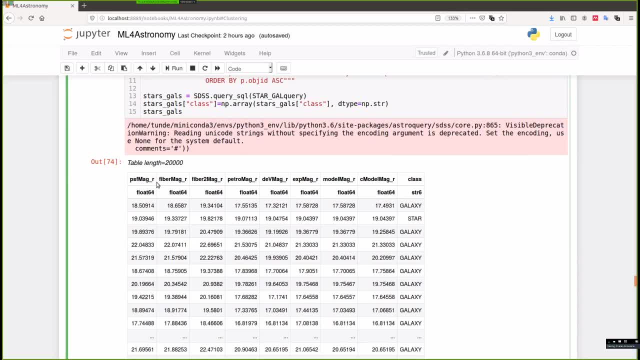 you already know something about the data because someone has you found a way to actually examine some of these cases. here i'm trying to to distinguish between stars and galaxies from the from there, from there from the sdss catalog. so i've taken a labeled catalog which already 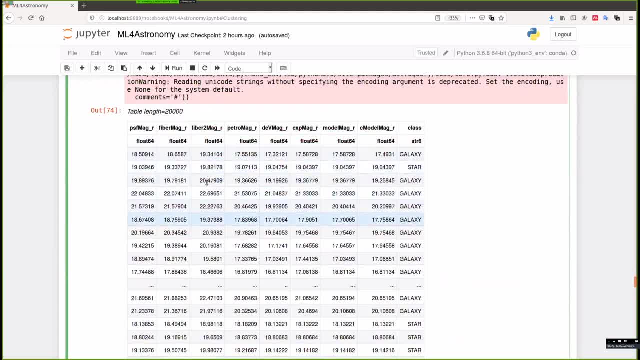 assigns a source to each of this. each of this, each of these sources, has been assigned a class, so you can see that it's either it's a galaxy or a star- a galaxy or a star- using eight of these features. so the point here is to try to use a supervised learning algorithm to predict if a 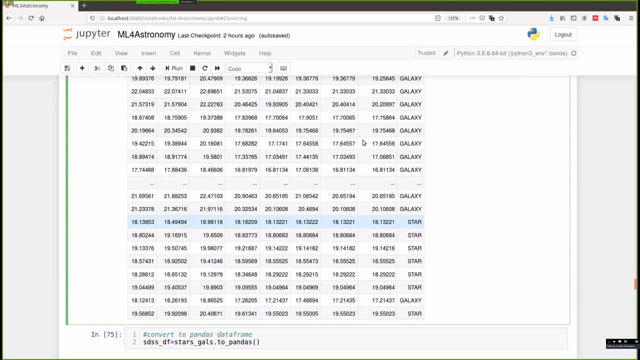 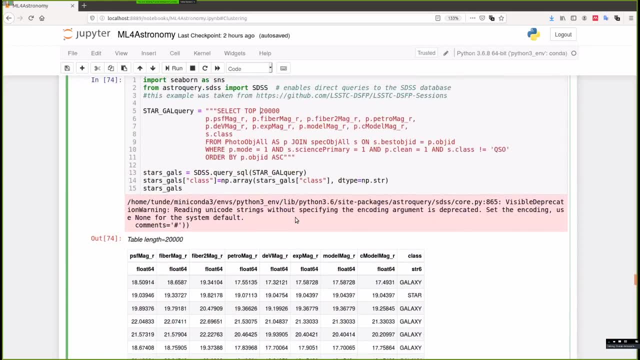 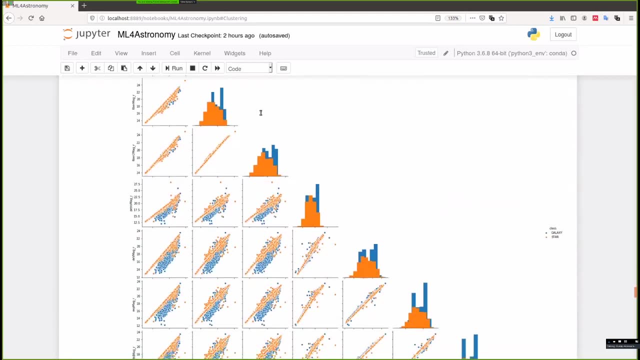 source is actually a galaxy or a star, by learning from these already known spectroscopic observations of this, of this data. so here i have to 20 000 data downloaded from this, from this data, from the, from the sdss catalog, and you can plot all of the data points using this sns plot. it's from seaborn. 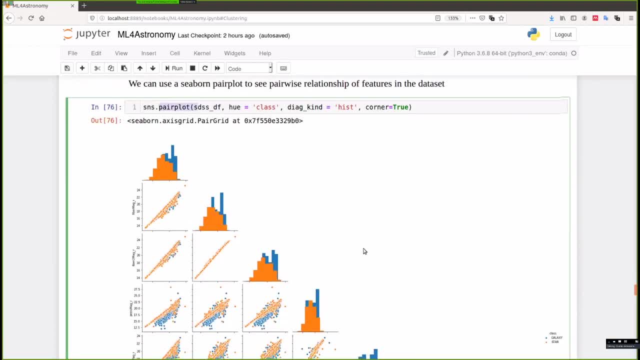 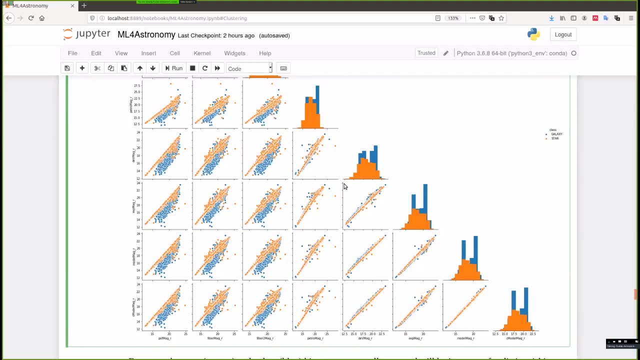 it's a very good feature to actually explore your data. it shows you the relationship between each object object in your data, in your, in your data, you can see the stars have the orange histograms and the orange points, whereas the galaxies have the blue points, in order to be able to 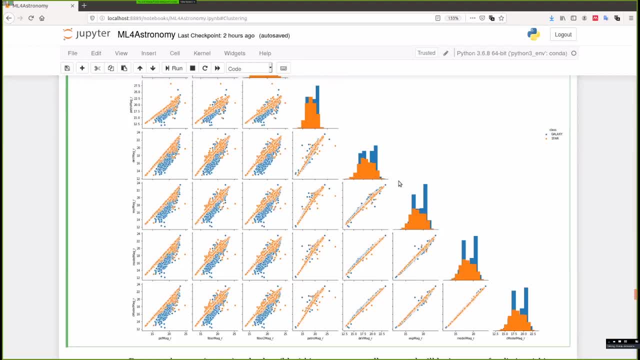 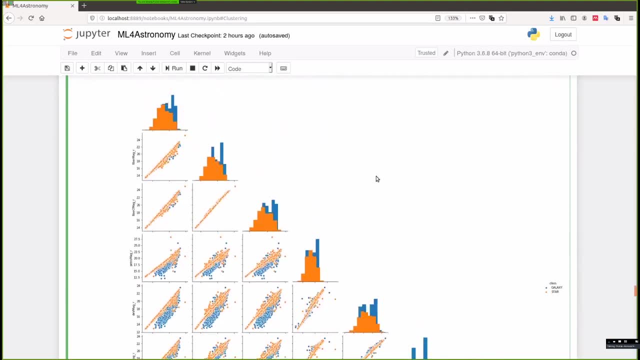 well separate these sources. they have the kind of. they have to have some kind of separation in the parameter space. i don't know if anybody can determine which of these features will easily be separable if we run a supervised learning algorithm on them. i would say the first one because you can see the blue points here are a bit. 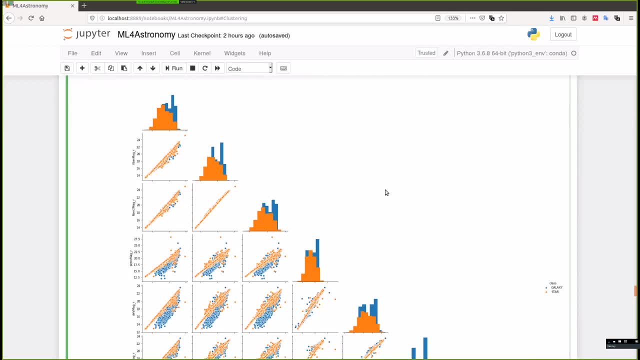 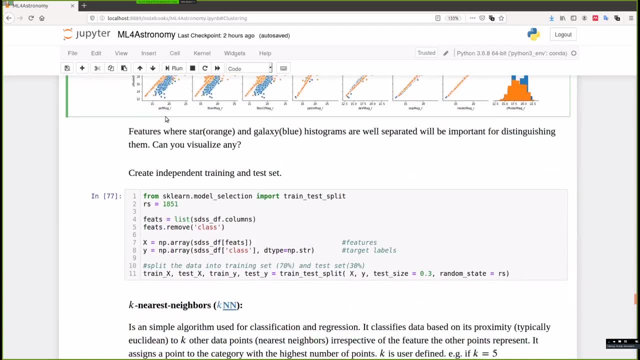 shifted from the orange points, so it might be very important in in distinguishing stars from planets, uh, distinguishing stars from galaxies. so what to actually do in supervised learning algorithm is to actually split the data sets into a training set and a test set, because if you train, you train the algorithm on the training set. 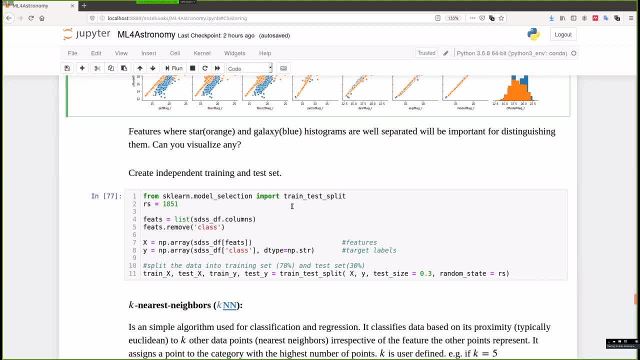 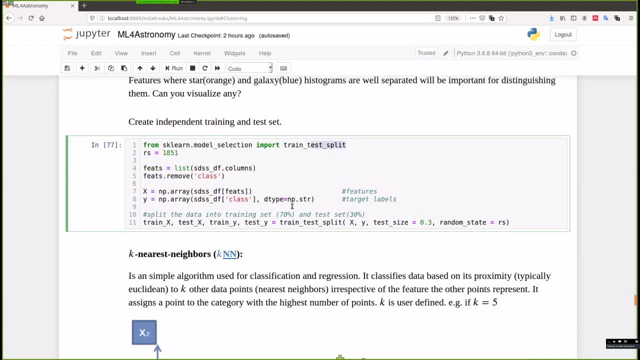 then see how much how it performs on the on a different set that it hasn't seen before. right, the s kill then actually also has a method to actually easily split this data randomly between training and test sets. in this case i'm using seventy percent for the train, for the test sets. 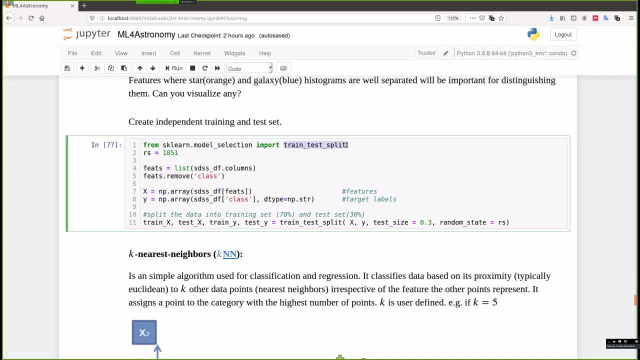 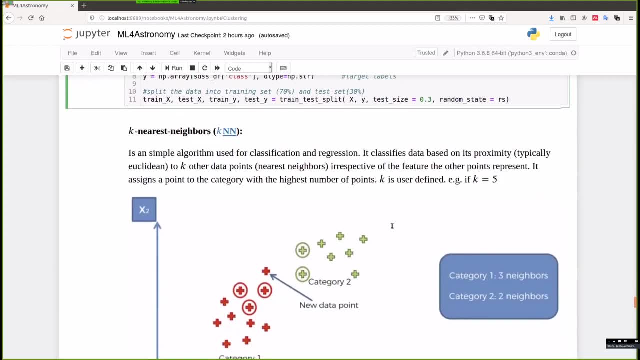 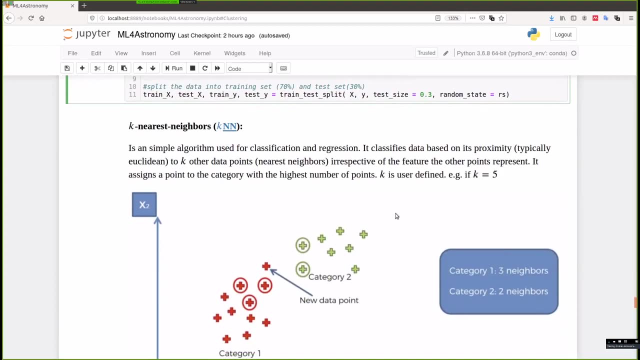 and thirty percent for the seventy percent for the training sets and thirty percent for the test sets and the algorithms to go to first is the k nearest neighbors in the in this algorithm, which is used for classifying or regression, depending on the problem that you have, 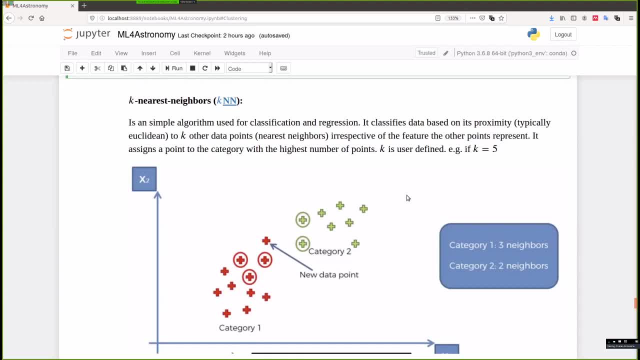 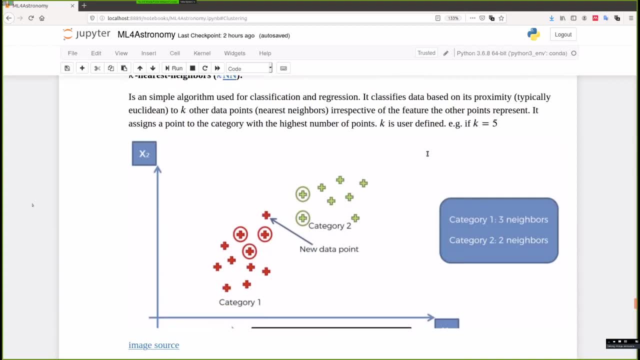 You define a K value, which is number of neighbors that you expect every point to have, And I think it is well captured in this schematic Imagine- I'm trying to classify this point right here. being pointed to, I find first the five nearest neighbors. 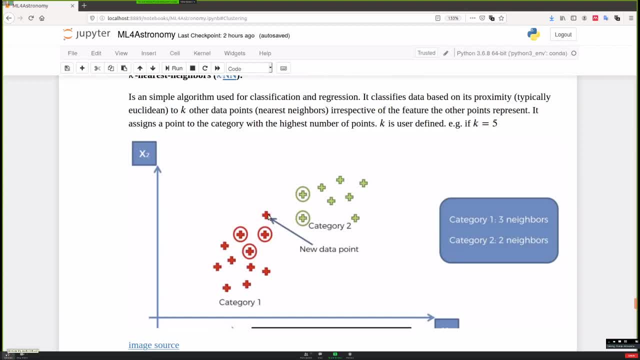 which is the K value here, the five nearest neighbors. Then I count It's closest to how many of the sources in each class. In the case of the red ones it's closer to three of the points, Whereas in the green it's closest to two of the points. 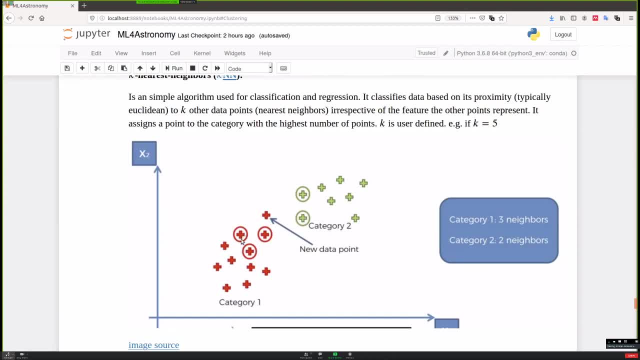 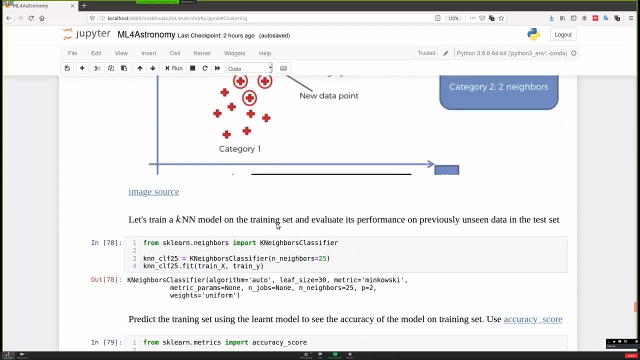 So the K means the K nearest neighbors algorithm in this case will associate these points to the red because they had the higher number of sources in that class. This is basically what it does. So if I try to use this K KNN in the case of our SDSS, 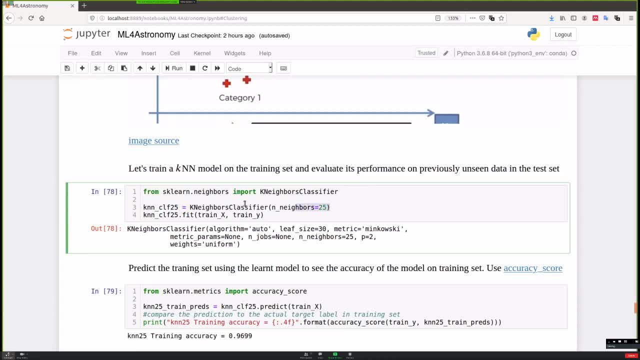 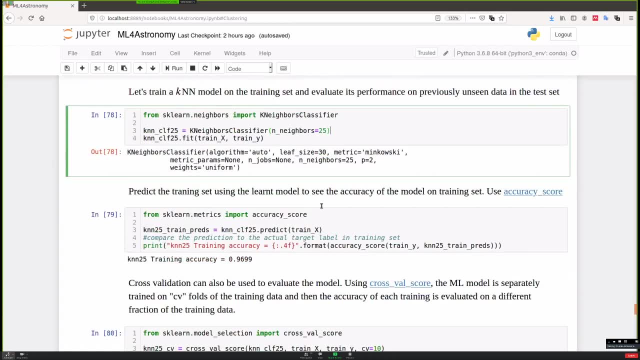 assuming 25 neighbors, because I have 20,000 sources right. It has to be close enough to a fair amount of sources to figure out which class it belongs to If I run the method, the K classifier- with 25 neighbors. 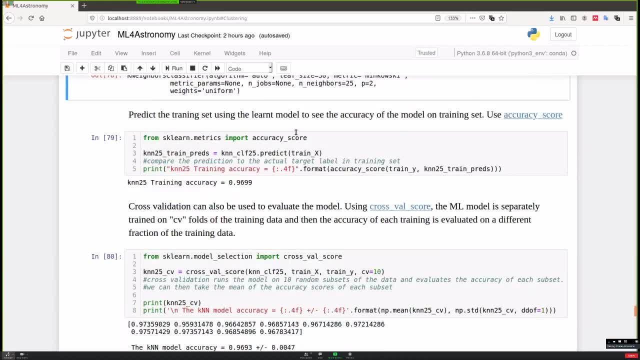 I can see how well it performs on the training set by comparing, because I know the labels of this data- by comparing the training sets to the actual predictions from the model, in which case it gives a 0.969% accuracy, not percent. 0.9 out of one: 0.96 accuracy. 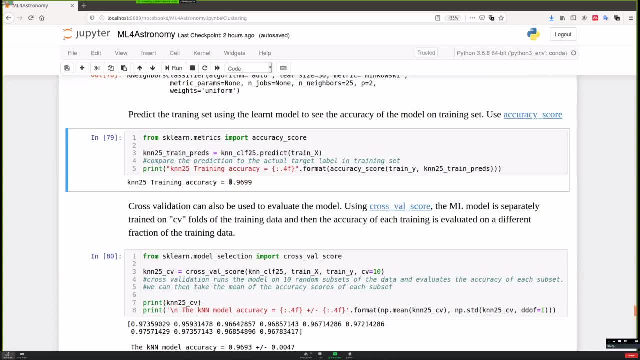 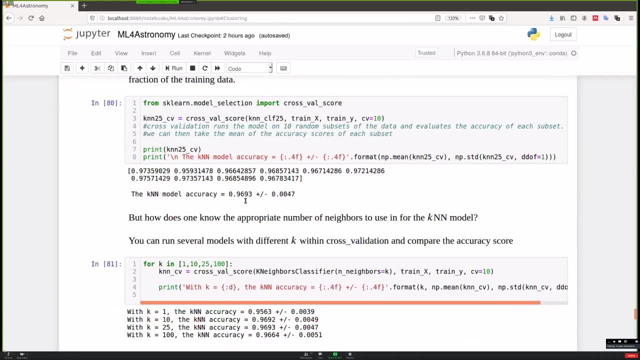 which means that this is very well distinguishing between the, the stars and the galaxies. But it's also difficult to know how much what value of K to use in each of the algorithms. right, So you can run something across a cross validation. 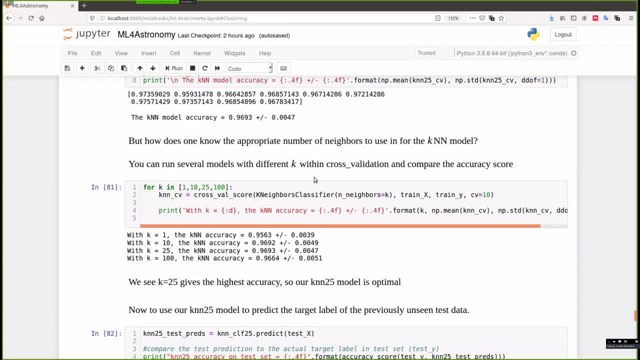 So I trade over each of the different numbers of Ks to see which one actually provides the best accuracy of your training sets. And when K is one, it gives an accuracy of this, And when K is 100, it gives an accuracy of 0.66. 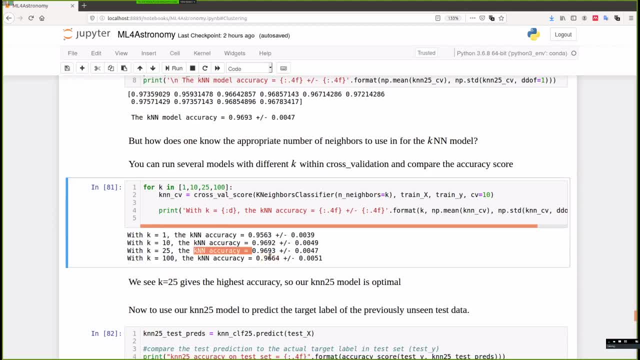 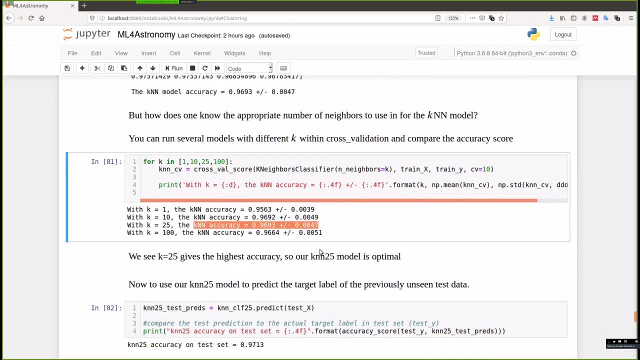 We can see that at 25, you already have one of the best accuracies to distinguish some of these data sets, So it's a good enough number of neighbors. This method is very interesting because you don't need to optimize any other parameter besides the number of neighbors. 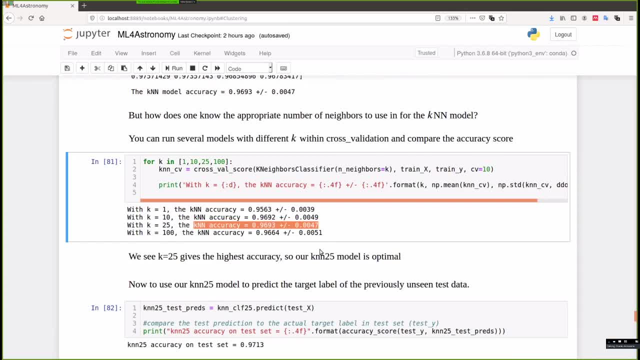 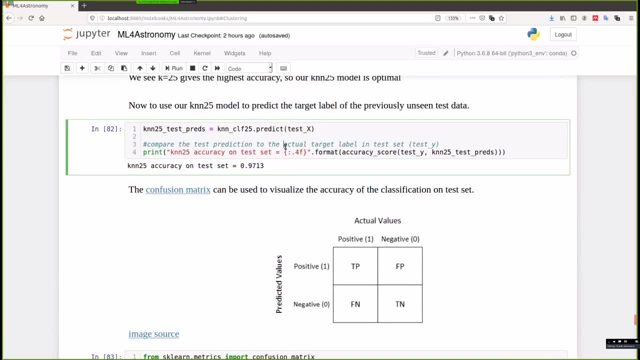 that the algorithm uses to define each of the classes. So a prediction now of the test data, which it previously did not see right. It trained itself on the training sets, but now I want to predict the data from the test sets. Predicting from the test set: it has a 0.97 accuracy. 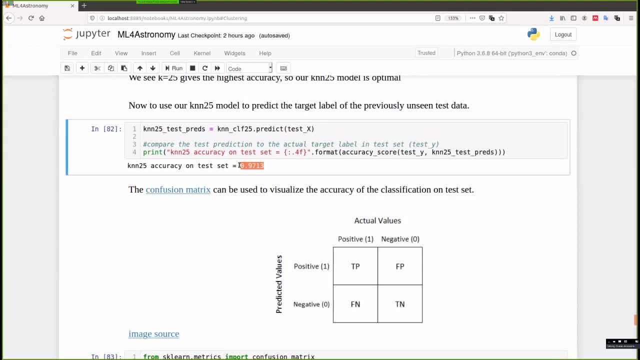 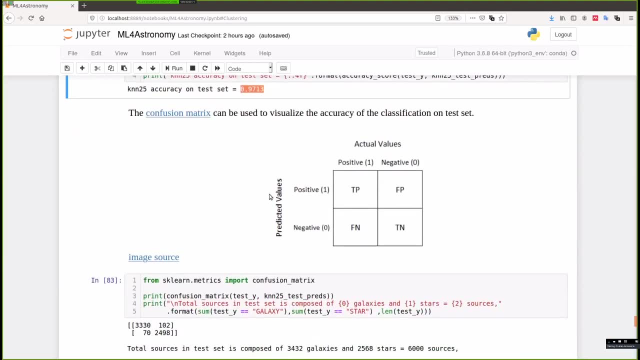 You're predicting correctly either if the source is a galaxy or a star. And to actually visualize the performance of the machine learning algorithm, you can use something called the confusion matrix, which tells you the number of true positives that you had in the data. 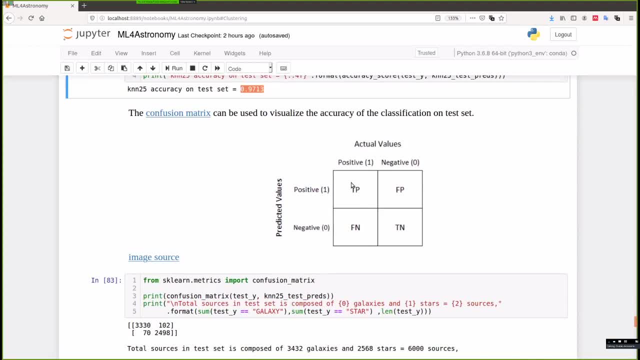 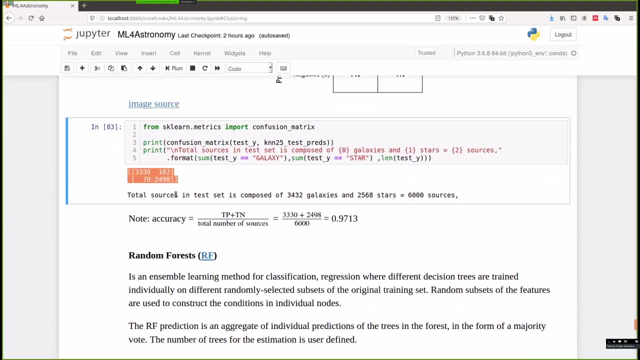 The true positives here are just galaxies- number of true galaxies. The true negatives are the number of true stars. Then the false positives are the ones that were galaxies that were classified as stars and the other way around. And running this confusion matrix on the test set shows that 3,000 of the sources. 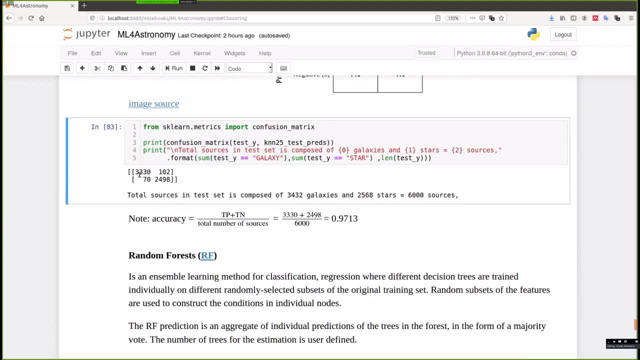 were classified right as galaxies, whereas 2,005 were classified as stars. But you can see 102 and 70 of the sources were actually misclassified, meaning nothing is perfect, right? An accuracy of 0.97 tells you that some of the sources. 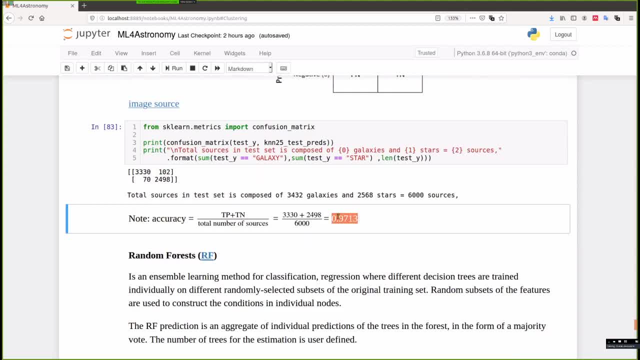 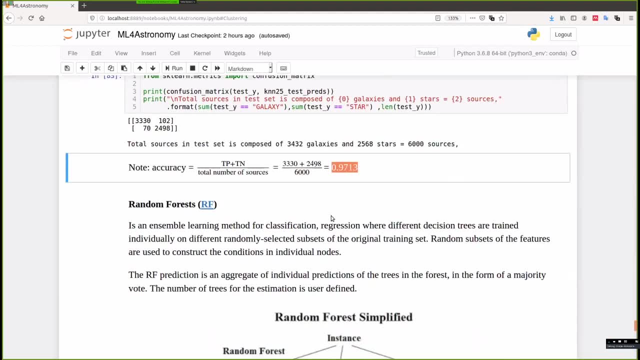 have been misclassified actually. Well, you want to minimize the number of true number of false negatives and false positives in your data as much as possible, So I think the last method I'll go through is the random forest. The random forest, basically, is a decision three. 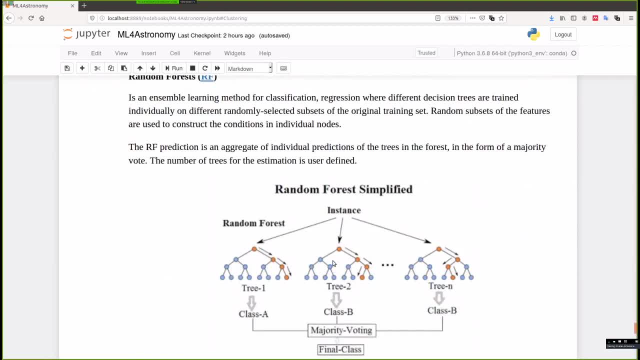 learning method, whereas it asks a couple of questions. So the data? are you beyond a particular level or not? If not, follow this part of the tree. If you are beyond this level, follow this part of the tree. It basically always asks decisions of the data. 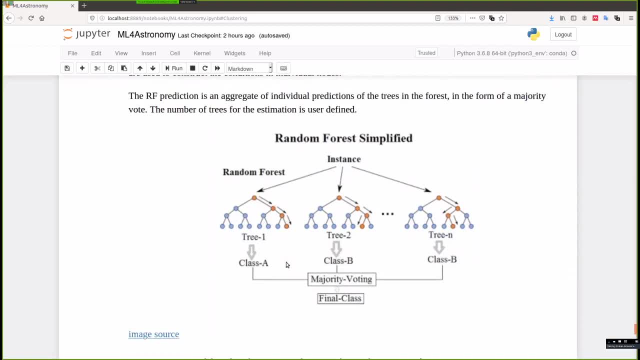 to find out what classifications they belong to, And at the end of it, it assembles all of them in a kind of majority voting technique to find out- okay, what classifications do they belong to? And at the end of it it assembles all of them in a kind of majority voting technique to find out. 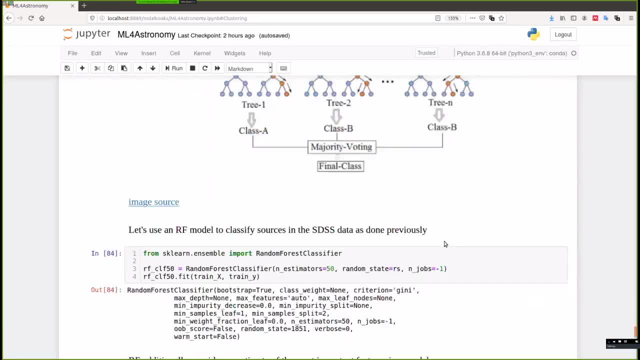 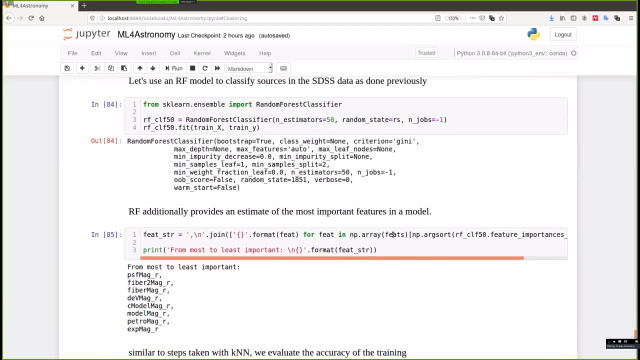 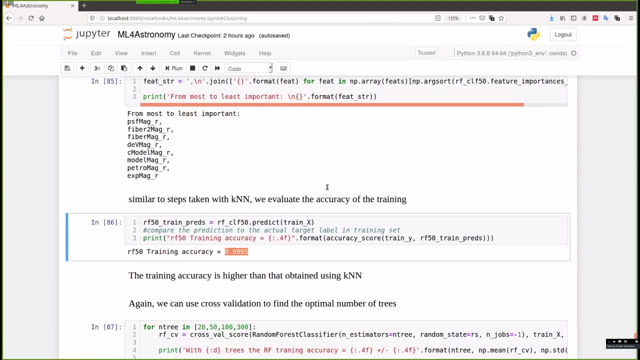 in which of the trees do you particularly fall in? Running this RF classifier on the same database, on the same data sets of galaxies and stars shows that you can have a training accuracy even way better than the KNN. You have 0.99 accuracy on the training sets. 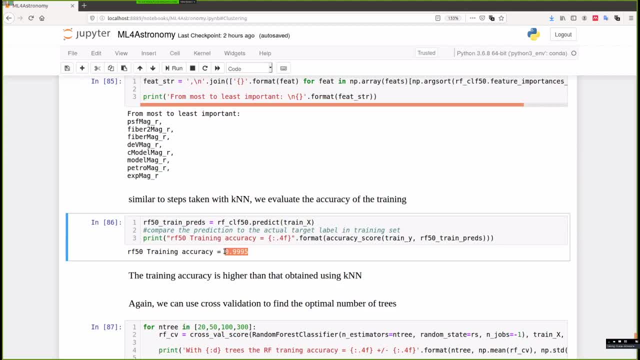 While an interesting feature of RF is that it tells you which of the sources, which of the features, are actually most important in classifying the data. In this case, I'm not going to go into the details of what the sources are, but it shows that the PSF magnitude R 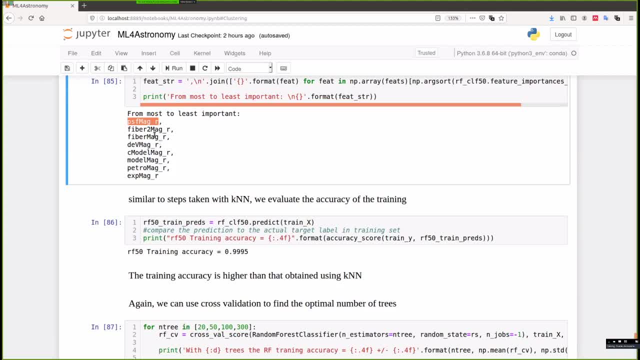 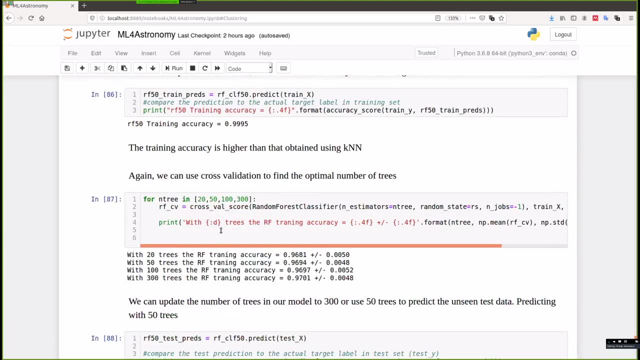 is the most important in separating between the stars and the galaxies, And if you are going to maximize your classification, you need to actually include this in your classification algorithm. But how many number of trees do we use to get a good performance? You can also do the cross-validation. 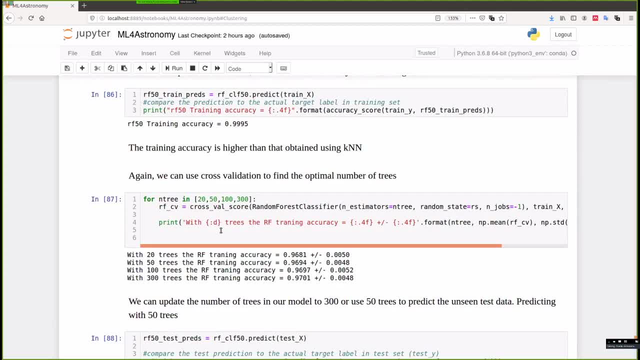 that I talked about in the KNN, to find out with 23s, what is the accuracy I get on my training set. With 100, with 300, what is the accuracy I get? In this case, we see that 300 trees actually provide the best accuracy. 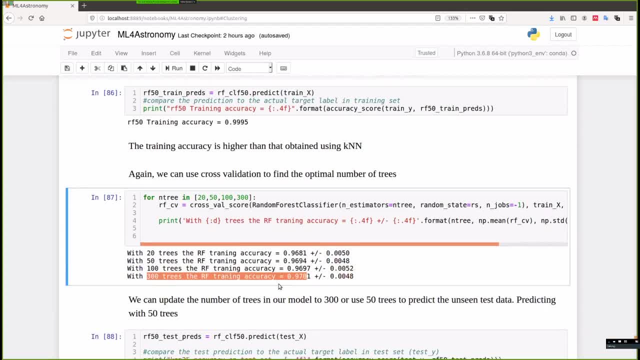 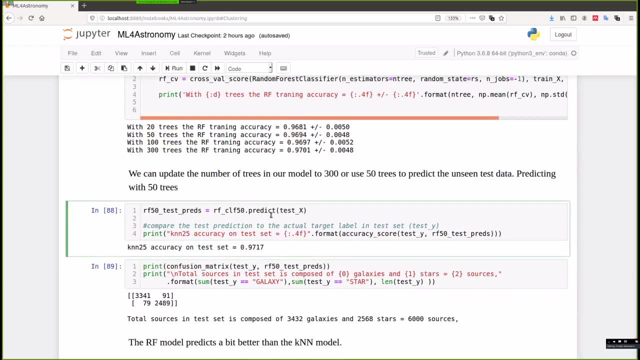 You could go so much further, depending on your use case, but I'm going to keep going with 53s because it produces a good enough accuracy. So, using this KNN model with 53s in them, I can predict the test sets, which I'm not seeing again. 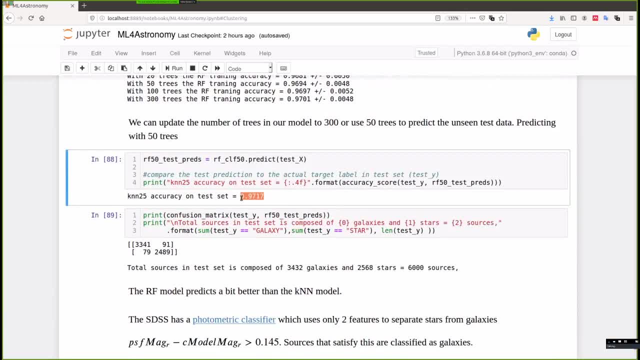 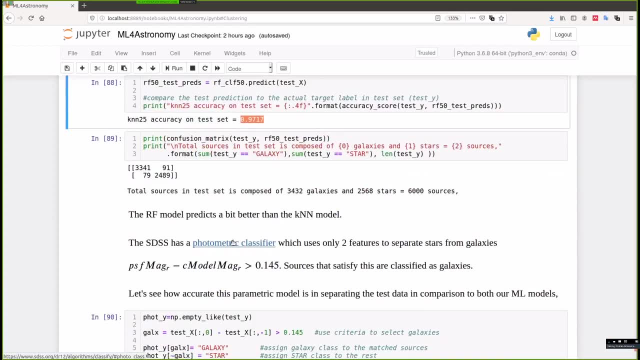 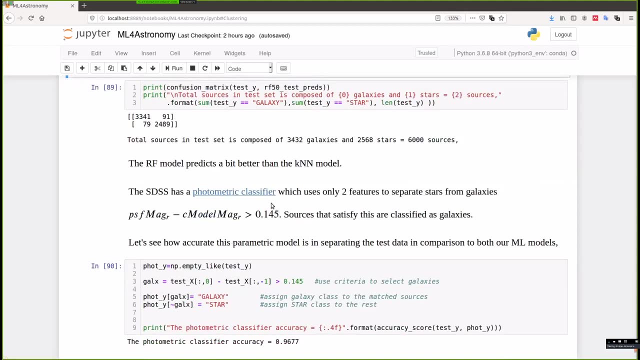 and it produces even a better accuracy than the KNN model, showing that the random forest in this case does better than the regular tree k nearest neighbors in predicting and distinguishing between stars and galaxies. but within the sdss frame itself they have a photometric classifier which is used to 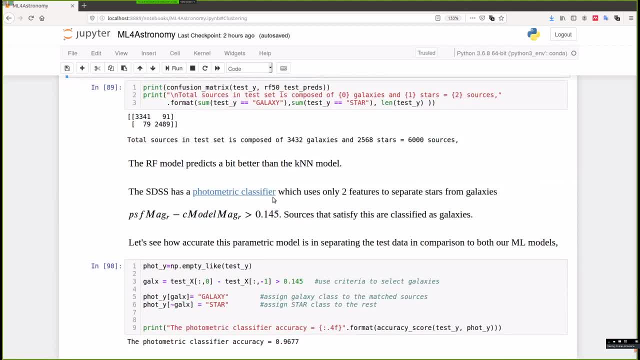 distinguish between stars and galaxies and it uses this parametric model. if the psf mark minus the c mode mark is greater than 0.15, then the source is a galaxy. so we can use this to compare how our machine learning model that we just did compares with a parametric model. that is usually 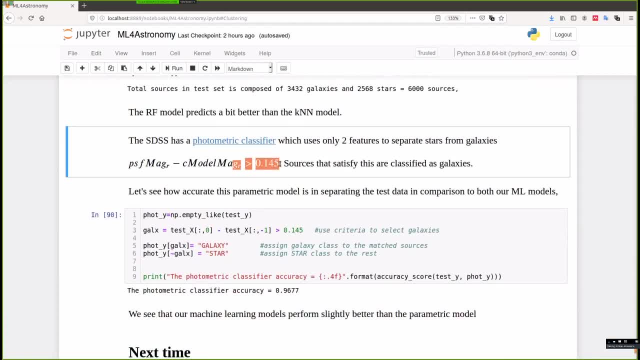 used to distinguish sources. using this parametric model, we have an accuracy of 0.96, whereas our previous algorithm has 0.97, showing that we perform better than the photometric classifier. so this already gives you an impression that machine learning is so much better at classifying. 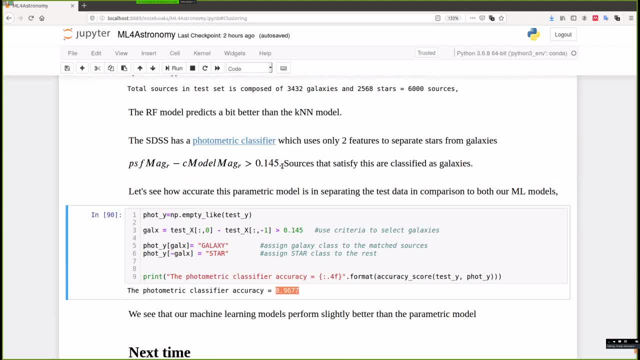 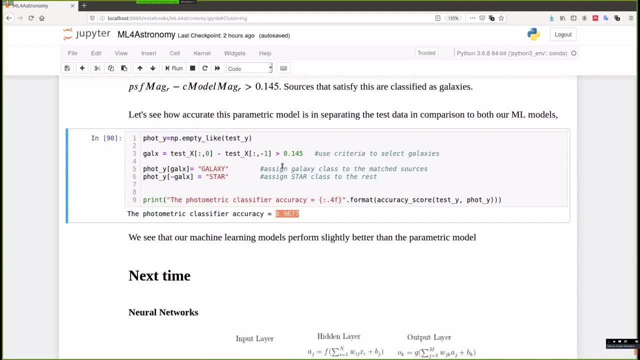 things than than parametric models, because you can use so many of the different uh features of the data set to figure it out. so basically, i'm going to stop here. i was really uh excited about talking about neural networks, which consists of a lot of things. you have convolution, neural networks, deep learning, neural 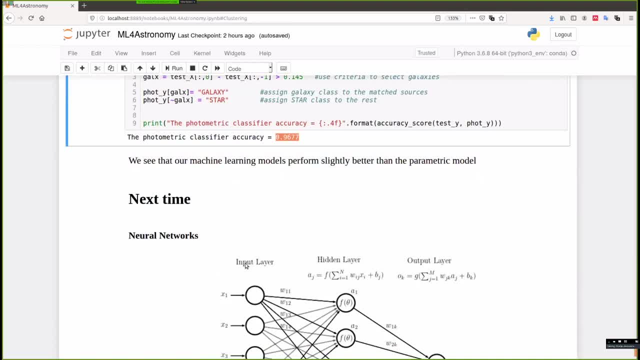 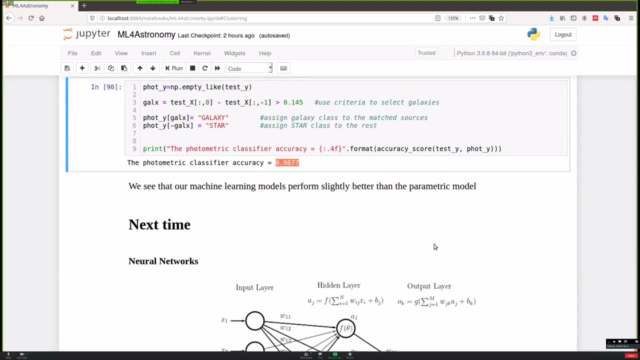 networks, but given the time frame of this presentation, i would like to do this at a separate time to actually delve into the details of of how it works for for supervised learning method. thank you. thank you, akin, for your nice presentation. does anyone have some question to to ask? please feel free to do so. 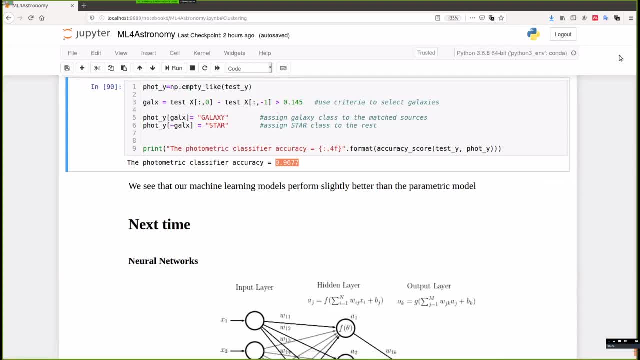 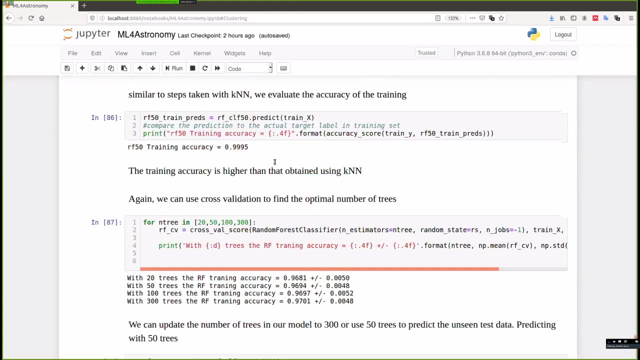 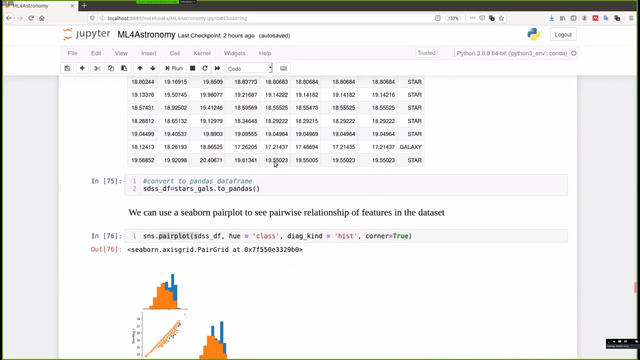 well, uh, i had a question akin. in the first part of your lecture you talked about the gaussian mixture model, i believe. gmm, yeah so, but how does how does it work? i feel like i have not understood how, how it actually is used or how it works behind the scenes. could you talk a little bit more about it? 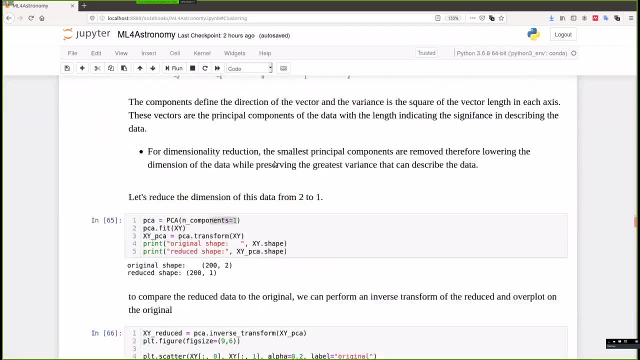 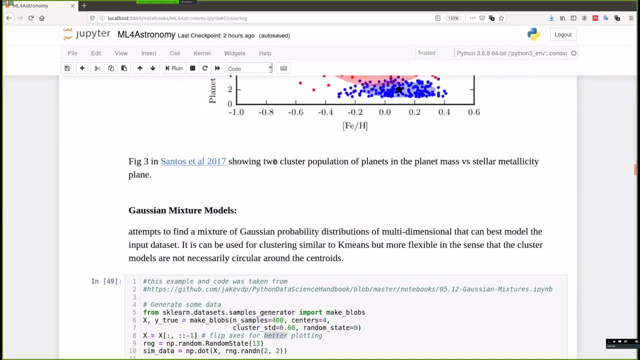 yeah, sure. so basically, starting with the gmm model, is: you have a, you have a say taking a look at it, and that's the gmm model, and you have a you you're looking for a gs that is consistent with the center of the network, so we have some sort of mapping and everything. 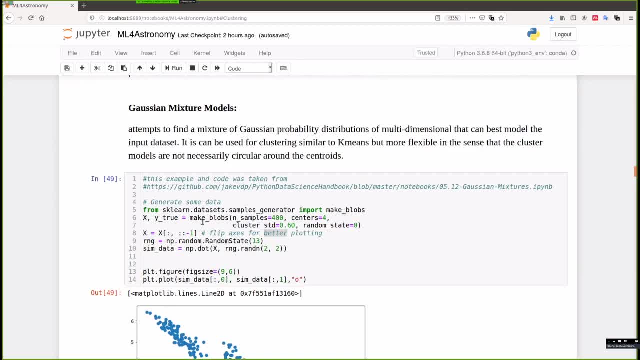 that you want to perform. and let's say: maybe you want to do a bevel tunnel, maybe you want to do a vertical field, so you can just have some sort of entire data set where you can just calculate the gmm model. and then let's say, you want to do two or several. 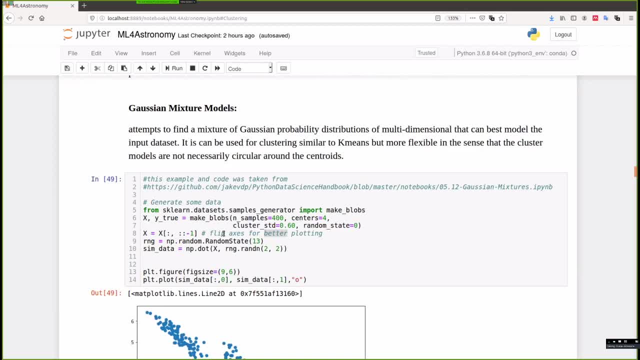 data set. so, that is, you are going to do two or three. they're all going to be Wes's gmm models- the properties of these gaussians, just that it's a mixture of several different gaussians in this case. that's why they call machine learning a kind of black box. you don't know what's happening. 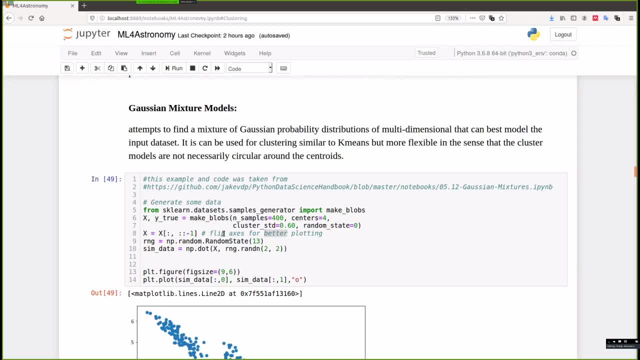 within it. you just know it's kind of mixing up gaussians to try to explain the distribution. so in this case, this is exactly what it does: it mixes up the gaussian distribution in a way that it actually models it in a particular dimension. sometimes you can put in some very specific 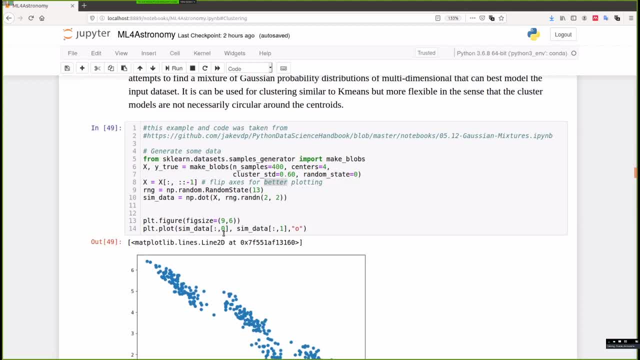 things if you know much about data set, like how you want the covariance matrix to be. you want it to fold in each direction, or you want the covariance matrix to go along the x-axis or y-axis. you can specify things like this, but beyond this i'm not. i'm not quite sure how, how it picks the. 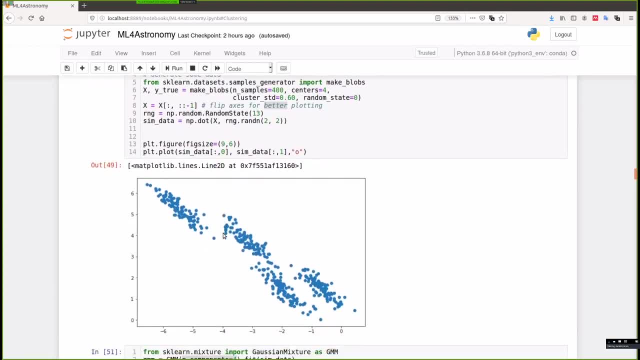 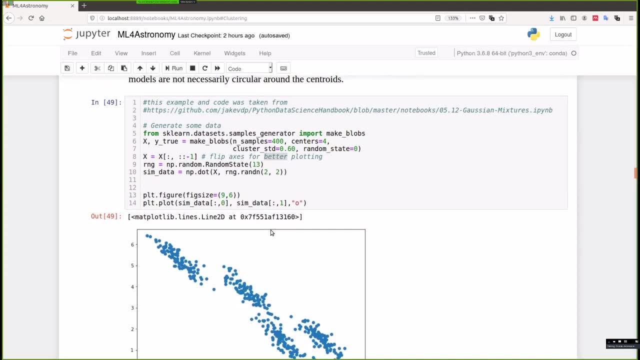 models. so i'll say that the centers are part of the model, the centers of the gaussians and some the sigma and some more stuff. but but you don't, you don't. you don't impute this by yourself. it figures it out based on the data. that's why the data driven model it finds each of these points. 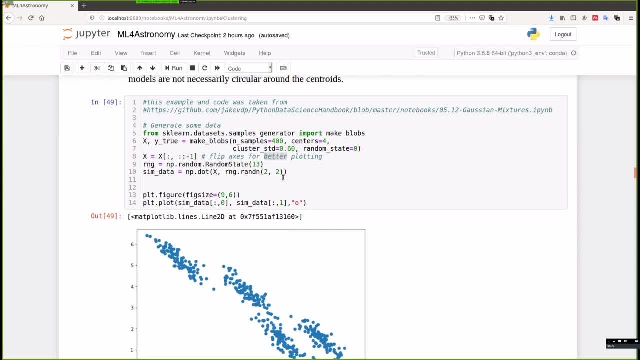 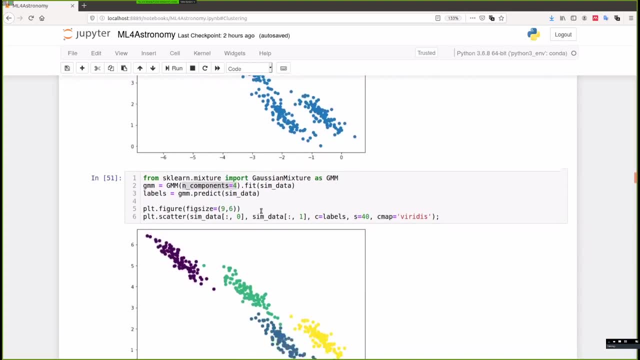 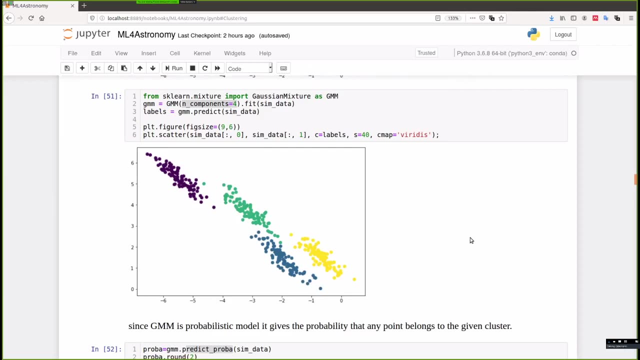 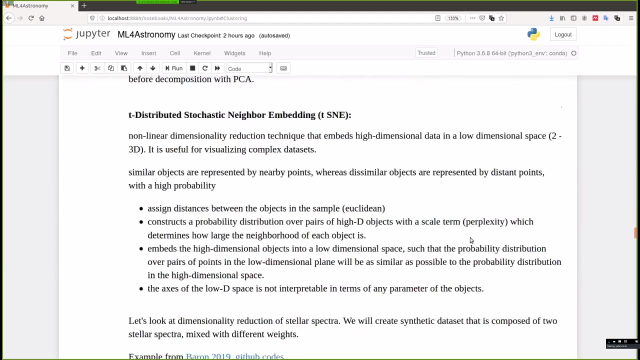 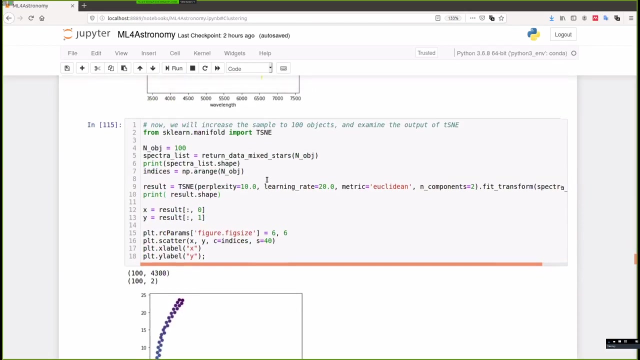 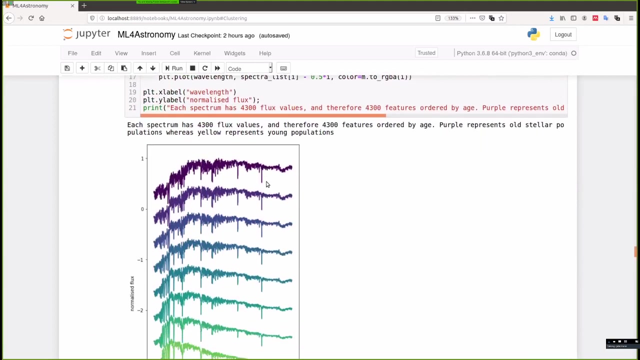 by analyzing the data. okay, so does anyone else have some question too? i have a question. okay, can you hear me? yeah, in your tsne example, okay, can you just explain me again? what was the input to the, to the function, to the tsne? okay, i mean the data. in what way does the data enter it? so it enters as. so in this case i had, i had a. 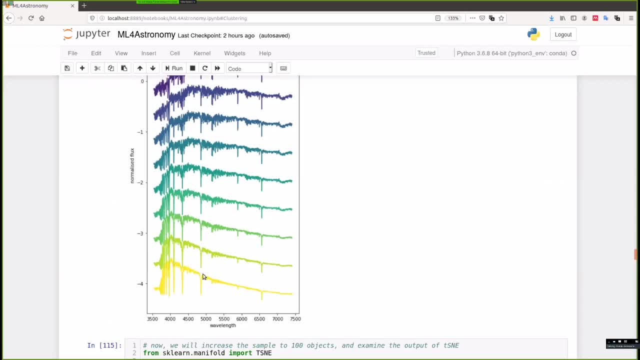 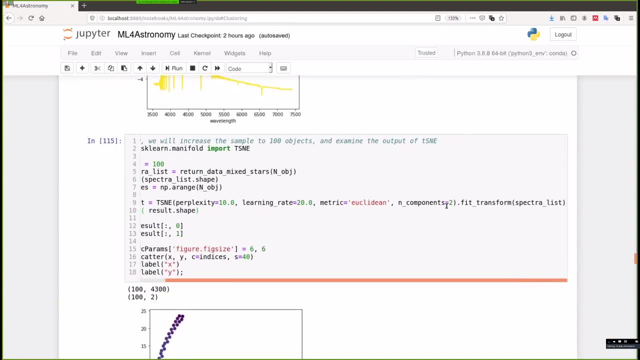 spectra. i created a list with each of these spectra in them different cases, so it enters just in the answers, exactly here. so when you create the, i created a list of this, all of this spectra, by mixing them in different ways. that doesn't matter. so if in this case it's a four, four 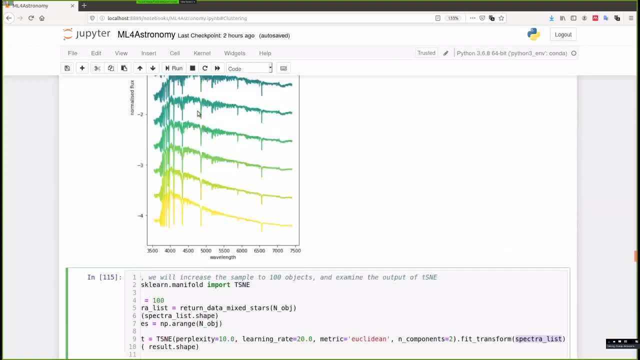 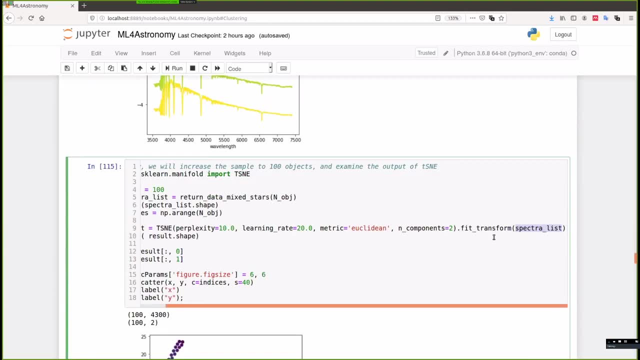 four thousand three hundred by um, by that's ten thousand. There's 10 spectra here, 4,300 by 10, basically OK. And then there's n components. is the number of x's in which you want to decouple, Sorry? 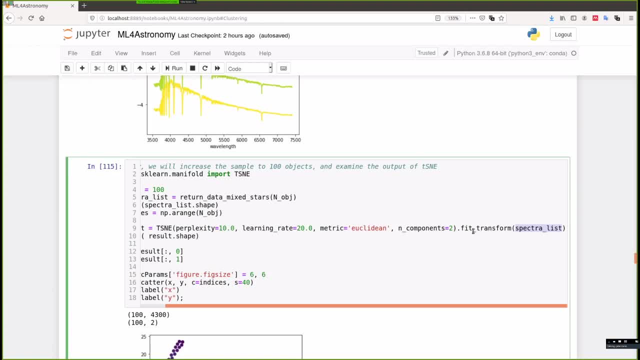 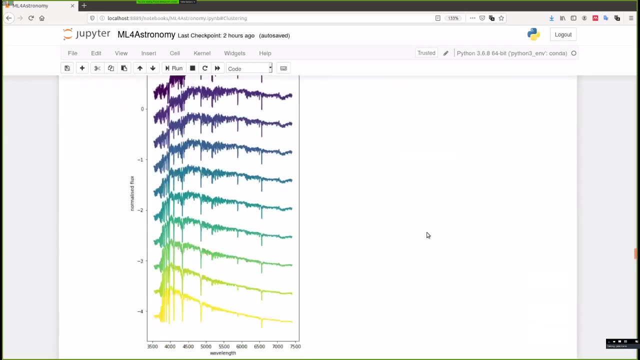 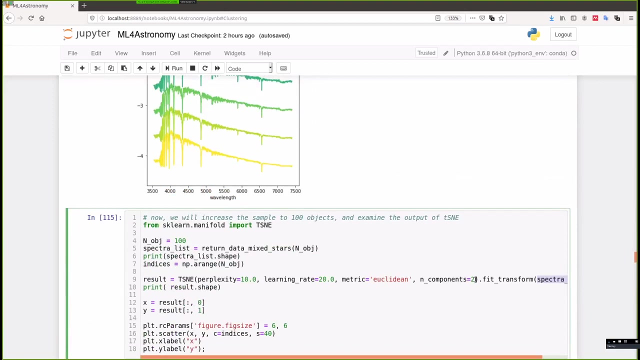 Your microphone is sounding funny. Sorry. The n components is: Can you hear me better now? Ah, yes, yes, Sorry. The n components is the number of x's that you want to decompose it, or the number of dimensions. Ah, the number of dimensions you want to reduce the data to. 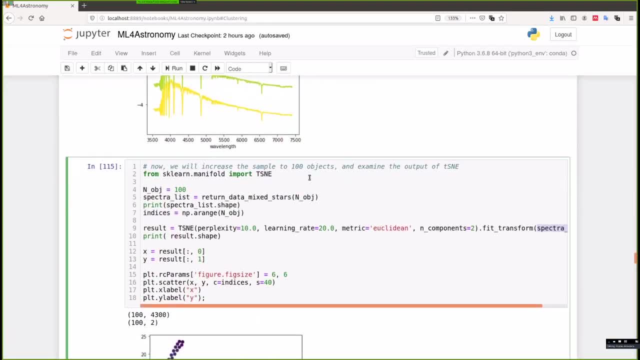 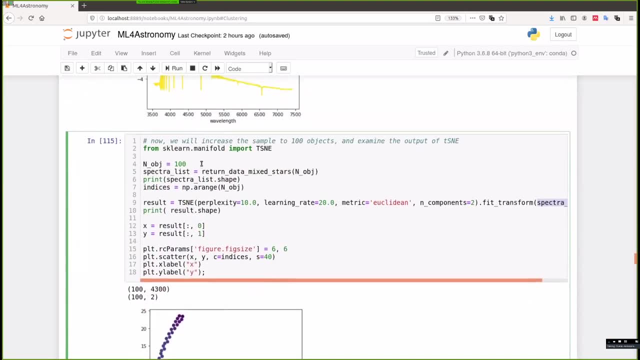 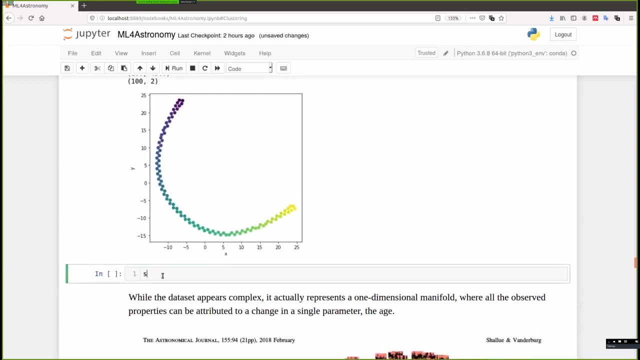 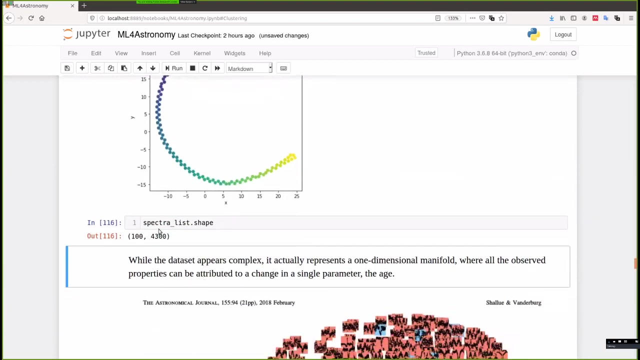 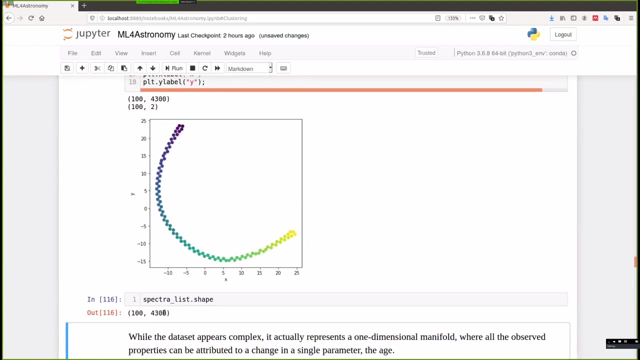 OK, So the data now is on a 400 by 2.. I have to check. OK, Thank you. So it has 4,400 features in it and it has reduced this to 2. Because there are still 100 points here. 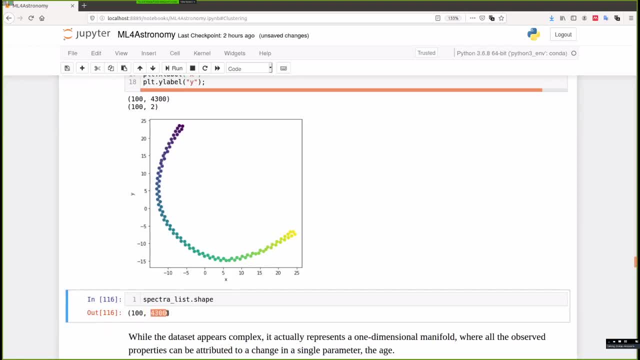 What it reduced is the 400 data points to just 2.. So the 100 is the number of spectra. It's 100 is the number of spectra. yes, OK, OK. So I think that's it. Yeah, it's fine. 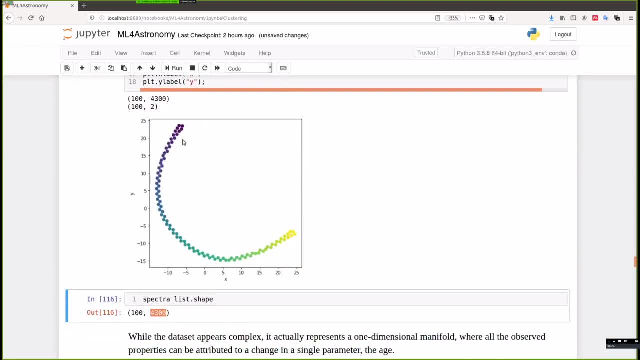 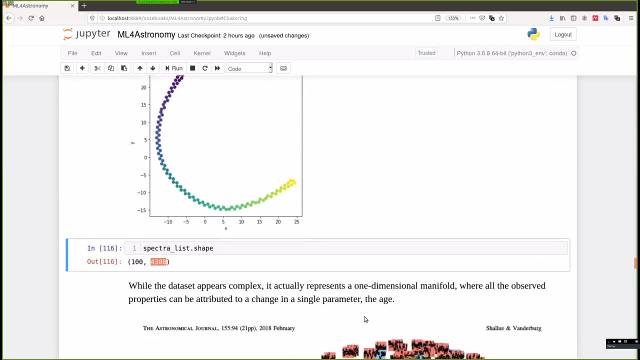 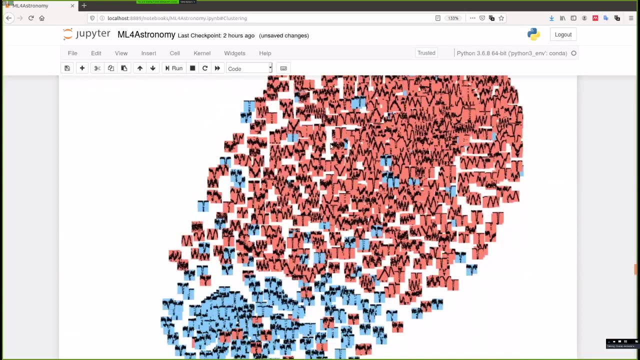 I actually represent one of the spectra that I showed above. Yeah, That would be the same case for the light curves. in this case, You would have I don't know how many number of light curves that you want to put in, depending on number of points. 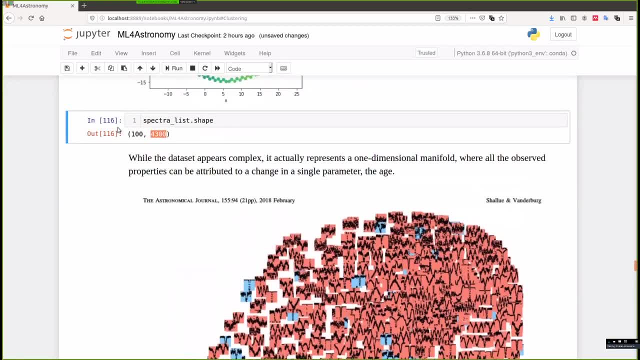 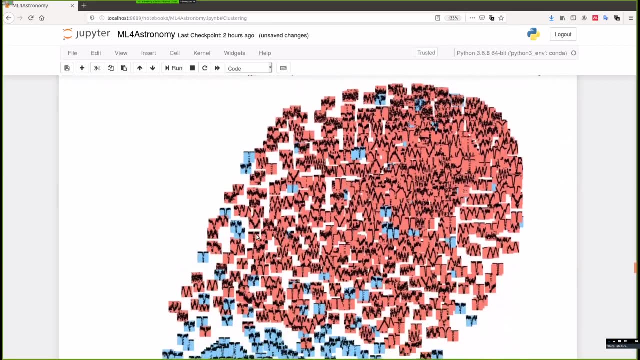 Then you put it: you also have maybe, I don't know- 1,000 light curves and the number of points. then it condenses each of the points in the life of into a single feature. do you have some experience with these hyper parameters like the perplexity? 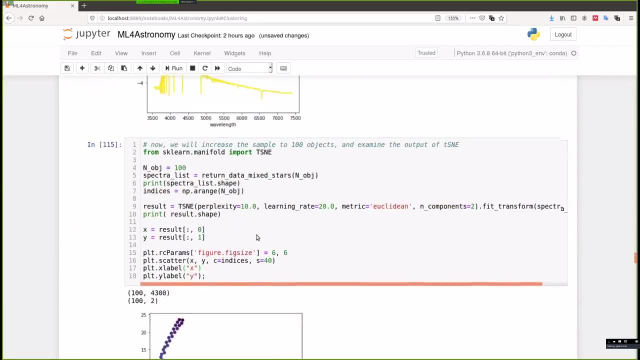 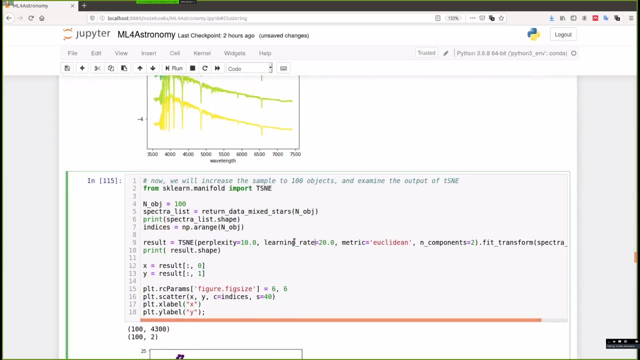 or it's something that, ah, it's actually interesting. yes, the perplexity tells. it tells, tells the data how to, how to define the neighborhood of each of the points. if you have a low perplexity, it means that your data set has a very, very small neighborhood around it. 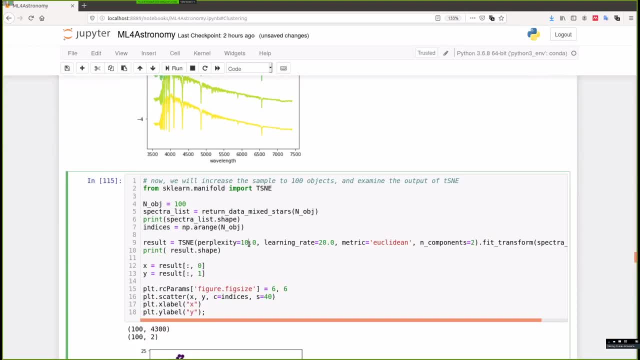 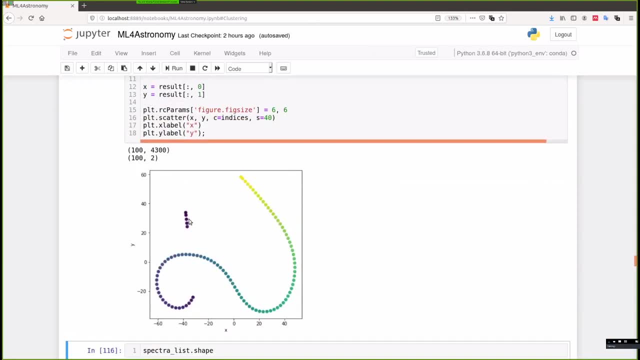 so finding neighbors will be very difficult in this case. let's try a perplexity of one and see what happens in this case. you can see it's, it's. this is. this is a fairly straightforward one around the second time, but it doesn't work very well if the if the neighborhood is very small. 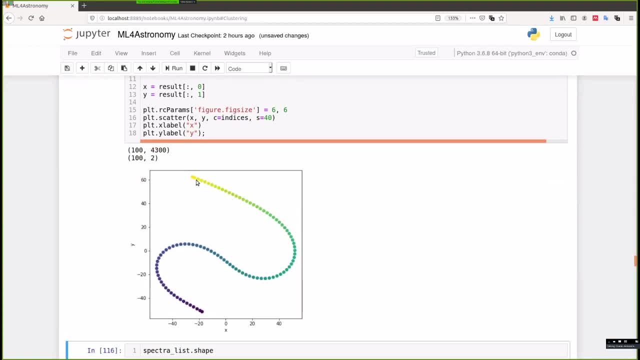 because you could have the impression now that this yellow point here is not so far from the green points down here because of this curved manifold that it eventually produces, which is not necessarily true, because the yellow point here is more related to the lighter green point than it is to the dark green point. but if you 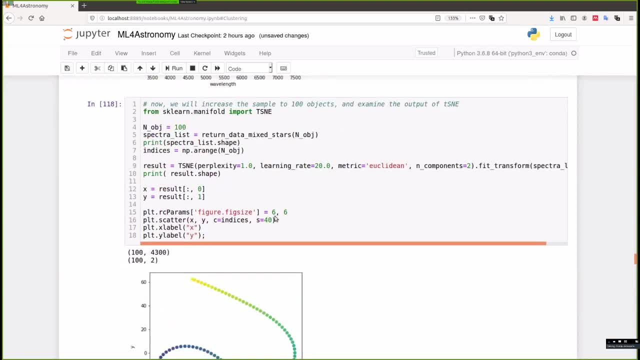 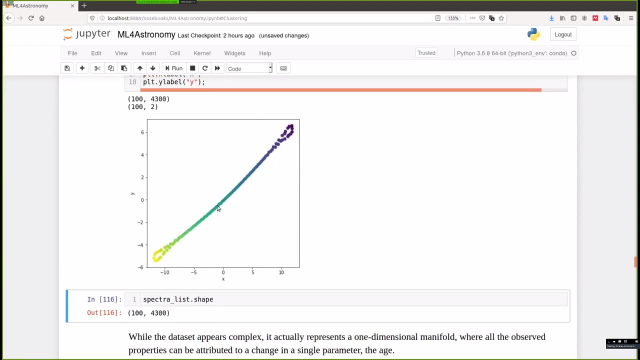 increase the publicity. it means that you are allowing more, more, more spectra to fit into a closer neighborhood of of another one. right, yeah, okay. so if i have a plasticity of 20, it's you can say the points are more condensed together because they're allowed to to fit into a closer neighborhood. 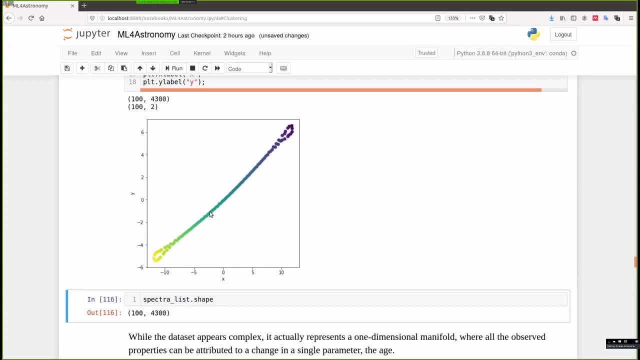 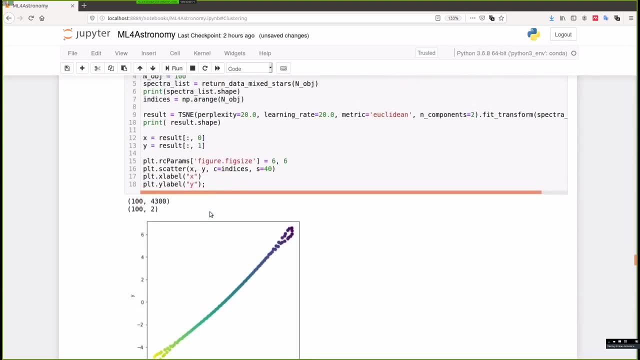 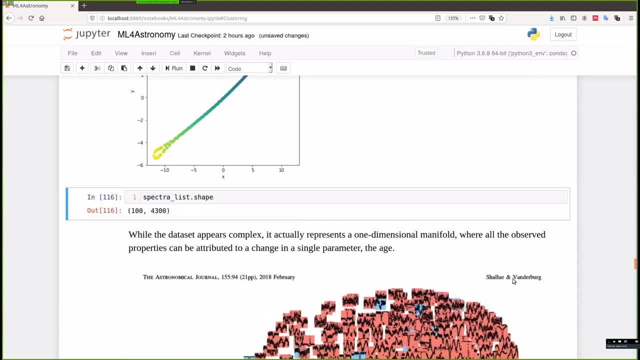 of each other. it's literally it's. it's actually just specifying how big is the neighborhood around a particular uh data point, but i actually don't have experience using it on my own data. besides this, and just another question- sorry, maybe it's, i don't know if you tried it- um the fact that it's. 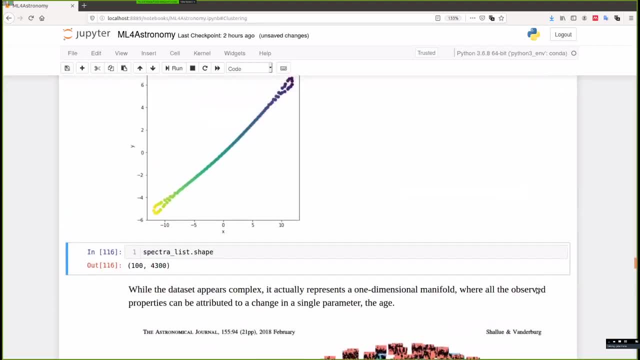 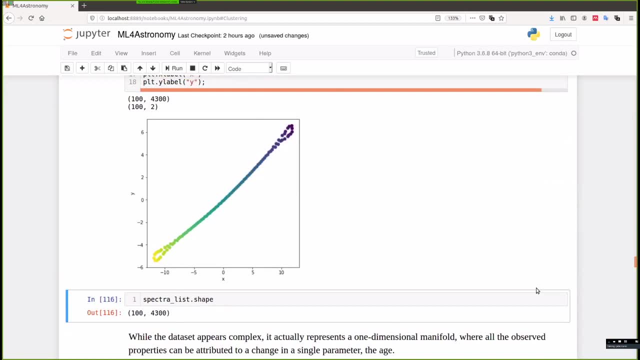 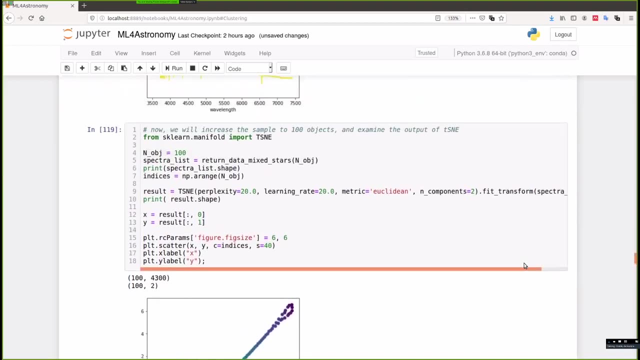 continuous sort of the output from the tsne? what? what would happen, for example, if you removed some of the ages, some of the spectra? uh, because the the difference in age between all the spectra is also continuous. ah, this is true, would you? i don't know if you tried, or maybe you would see some more. 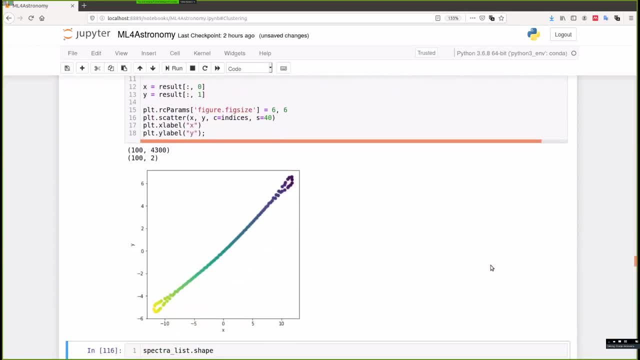 blobs in the output. i didn't, i didn't try it, but, yes, i think this is exactly what one would expect to to happen if there's, if there's a break, a distance between- say, if some of the points between here did not exist, i would expect a further distance. 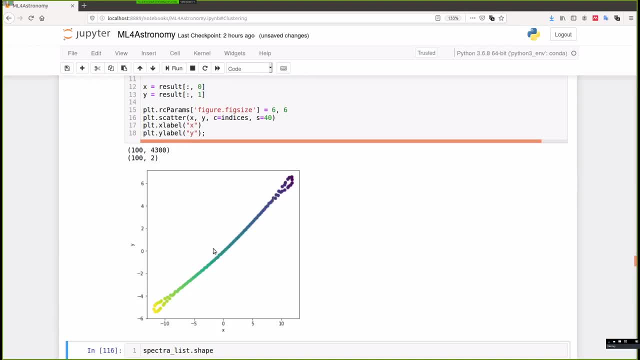 lizik huh, and if there's a distance between here do not exist, i would expect a further distance do not exist. i would expect further distance do not exist. and this is exactly one of the best conditions in the watch: uh, data between each of these points from each other. yeah, this is what i would expect. 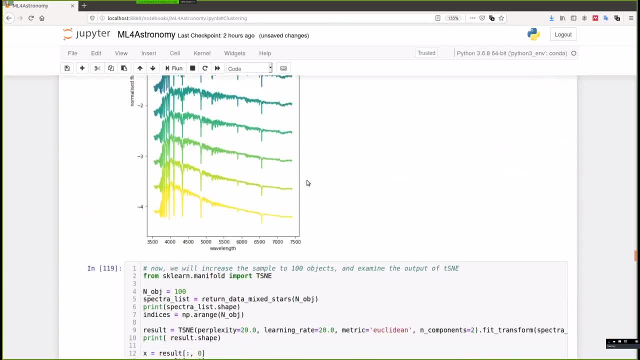 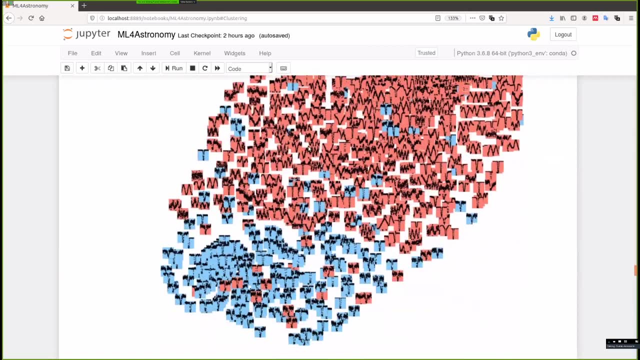 but yeah, something that i should try, fine. but because if you look at, if you look at this, uh, the tisny on this algorithm- you can see spaces in this data, which shows that even though this point, for instance, is close enough to this, it's not as close as some of the other dense points, right? so if you had some missing missing. 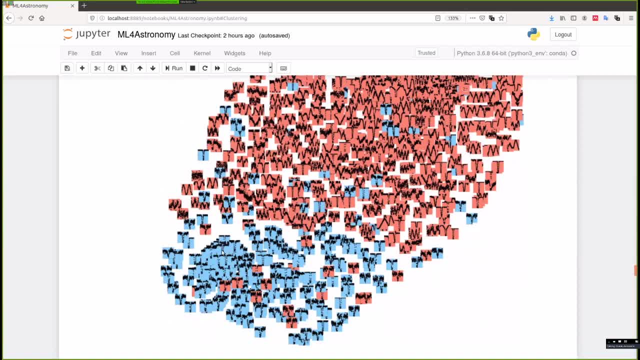 points within the relationships. they would appear as spaces in the, in the, in the output, and in that case, i guess the restriction is that all the data has to be the same right you have. you have to have the spectra with the exact same number of points. yeah, yeah, that would imply so, yes, and here the, the white curves also. okay, yeah, but but in this. 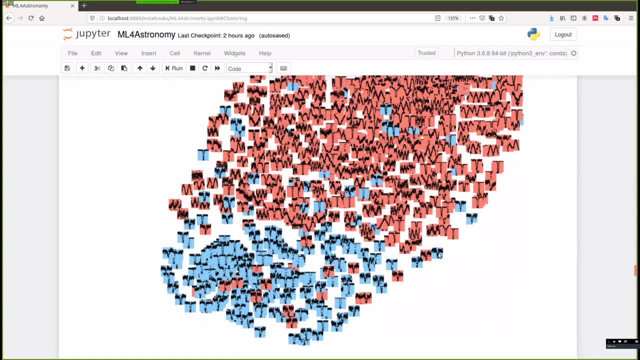 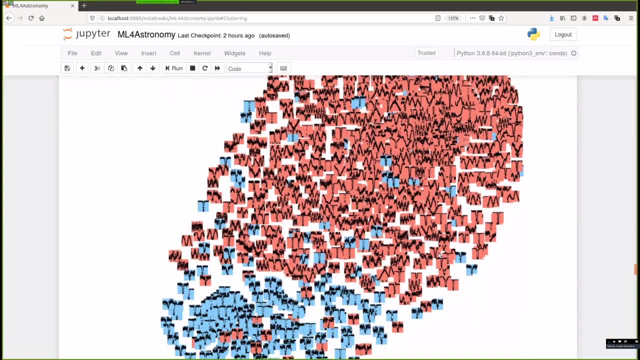 case, i guess one would just be in the light curves to have the same number of points before, uh, putting it into the t-snake. another. another recommendation of the algorithm actually says: if you have too many data points or too many dimensions, you can first reduce it using the. 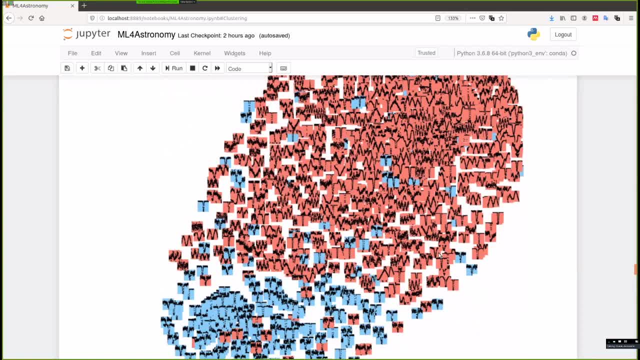 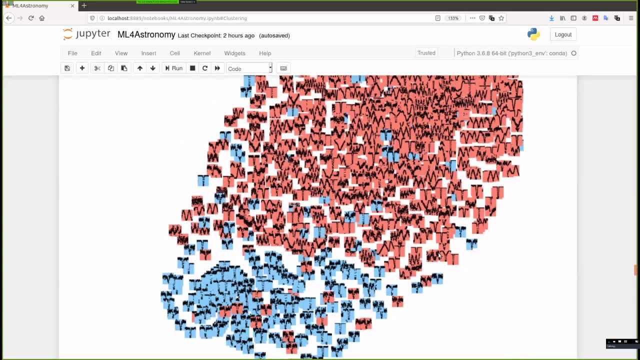 principal component analysis before feeding it into the t-snake. thanks a lot. yeah, okay, so if no one else has something to ask, we can finish in here. it's almost one hour. once again, thank you, akin, for your nice talk and